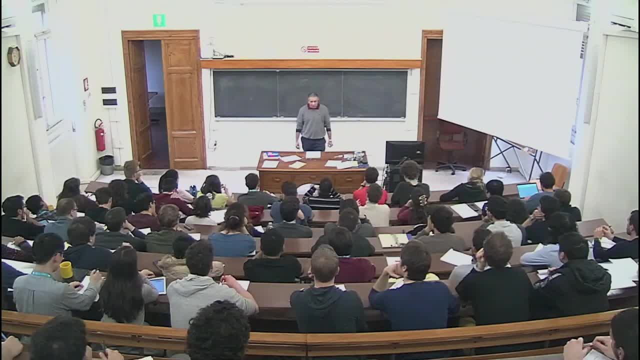 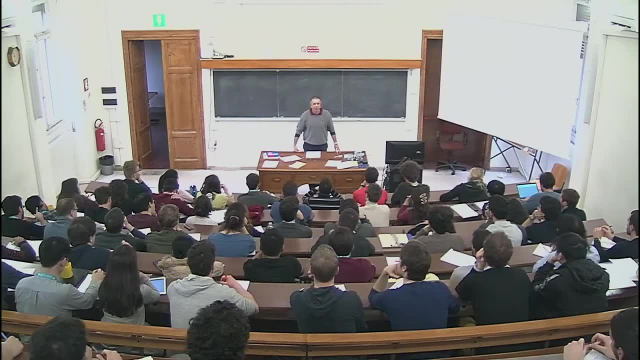 theory is the language of Feynman diagrams in order to compute decay rates and cross-sections. If you are unfamiliar with any of these subjects, of course we will not have time to cover all of them, but we can discuss them in the 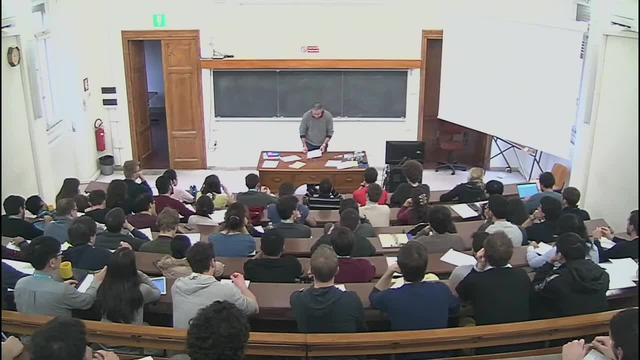 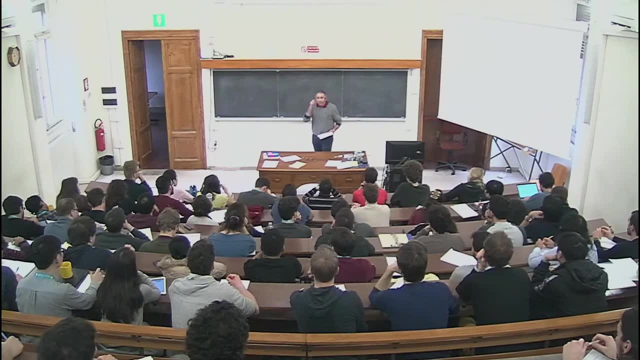 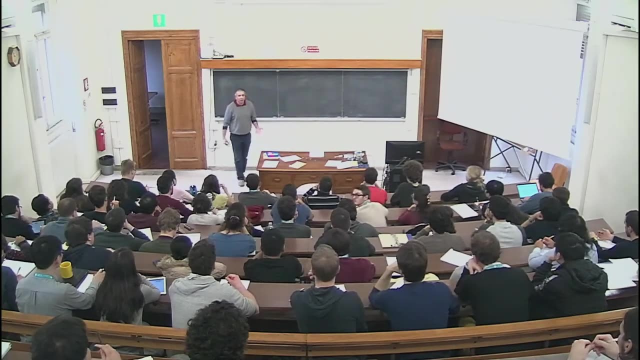 afternoon or in the tutoring sessions. So I think you all know what electromagnetism is. so let me say something about basic facts. in weak interactions, The first processes which were observed and recognized not to be determined by electromagnetic interaction are beta decay. 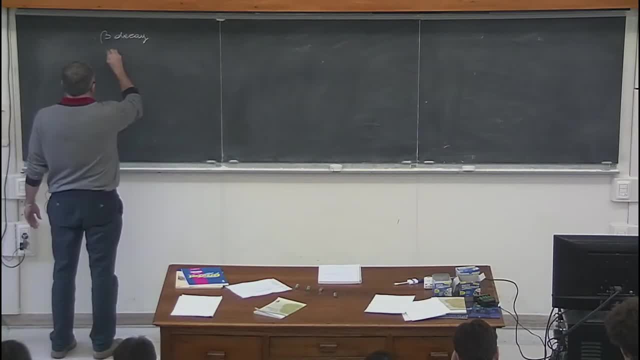 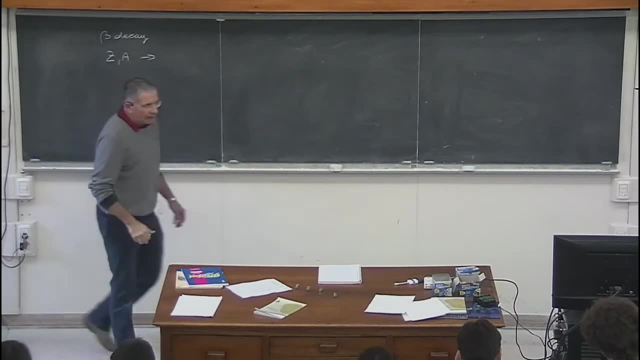 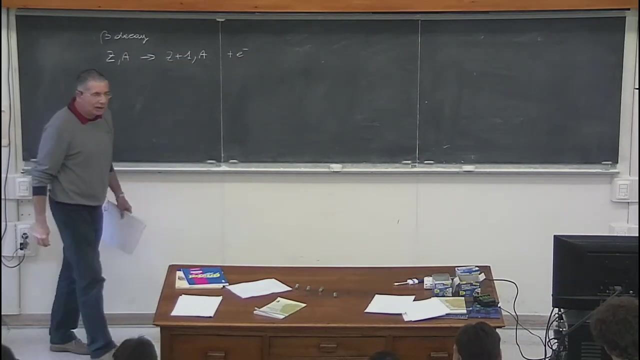 Beta decay of nuclei is the decay of a nucleus with charge z and atomic number a into another nucleus with charge z plus one and the same atomic number a, with the emission of an electron. and it was soon recognized that this is not enough. the emission of beta electrons is: 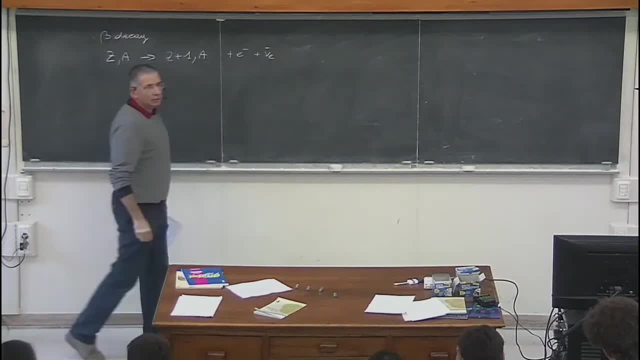 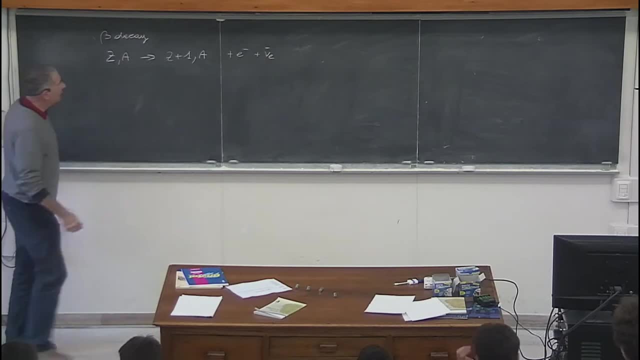 accompanied by the emission of electrons, And we will learn soon that neutrinos come in three different types, three different flavors, and this particular neutrino is called an electron neutrino. And a second process which was early discovered in weak interaction is the decay of the muon. Muons are present in cosmic rays and 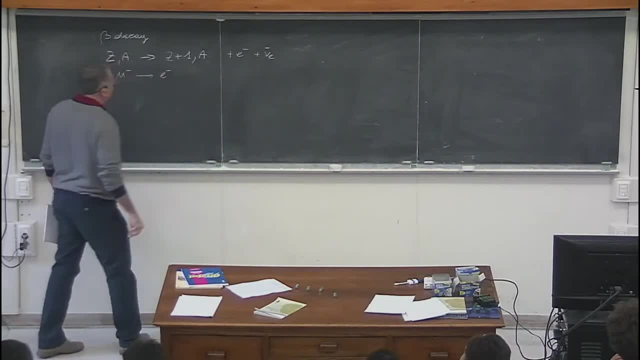 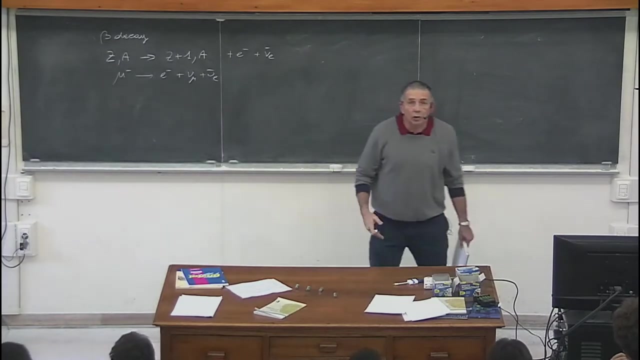 they are known to decay into an electron- this minus sign is for the electric charges you know- with the emission of which is accompanied by a muon neutrino and by an electron anti-neutrino. These processes are new. are new in the sense they are not strong interactions processes, nor electromagnetic. 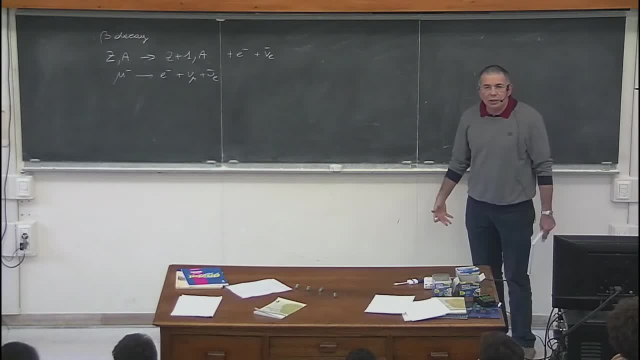 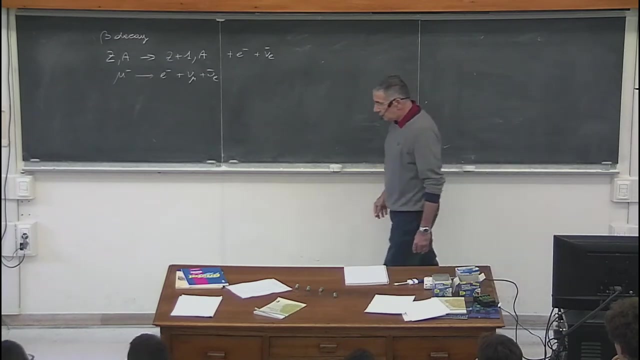 interaction processes. they you need to introduce a new kind of interaction, the weak interactions, And these generations of neurons also severally altered and the transfer of preterm actions move to자를. A testing is done conditionally in order to explain there existence. 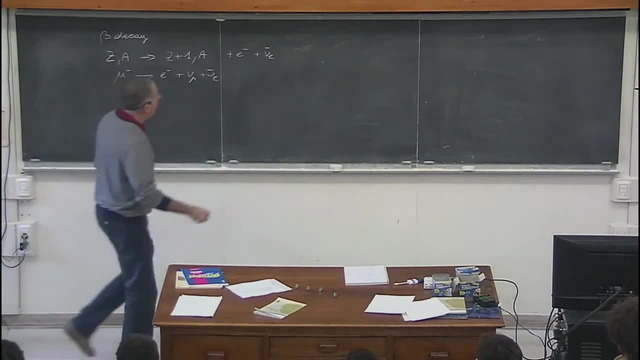 So the early, the earlier attempt to those theory of of weak interactions were made by Fermi, as you all know. and Fermi Did the naive thing: He just observed that these two processes involved four different mechanisms by where this process has been generated. 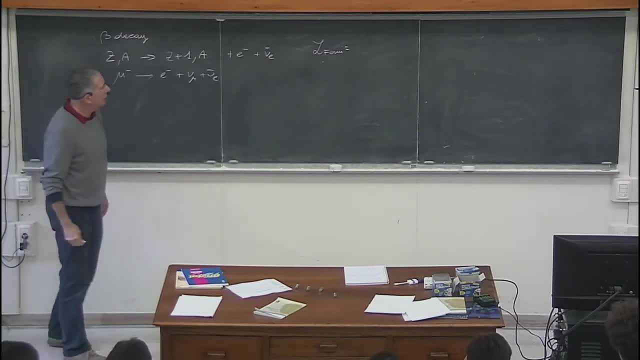 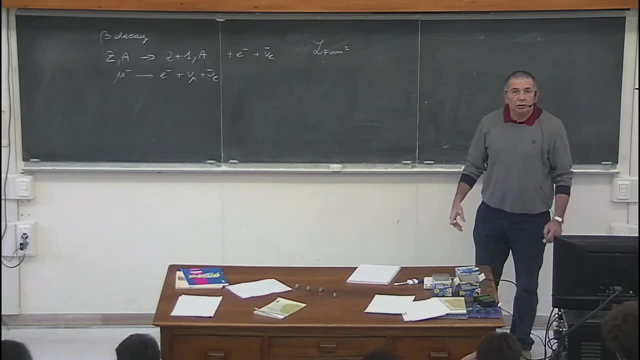 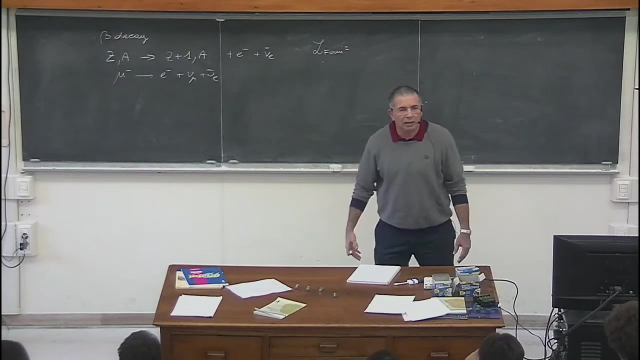 fermion fields for different spin 1 half particles and he wrote a Lagrangian density for this kind of processes which is essentially the product of four Dirac fields or four fermion fields combined in such a way as to be a Lorentz invariant. 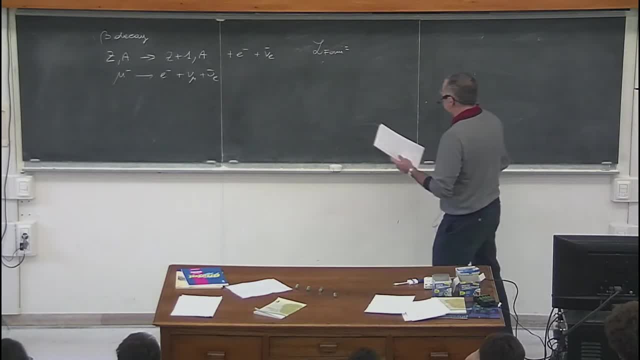 interaction term. The interaction term of the Fermi-Lagrangian is something like. I will be more precise in a while. there is a constant times a Lorentz invariant, a Lorentz invariant combination of four Fermi fields and I will say in a moment what. 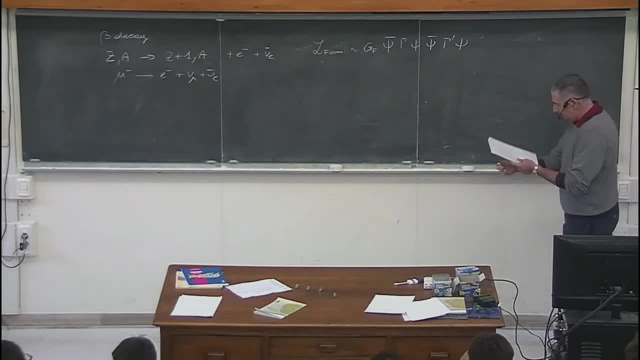 this capital gamma and capital gamma prime are. This constant here was soon recognized to be of the order of 10 to minus 5 times the proton mass, to the power minus 2 each fermion field carry a mass dimension of three halves and the Lagrangian density is a quantity. 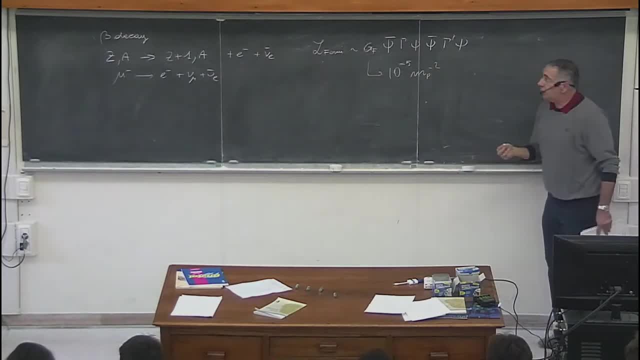 with mass dimension 4 in the units in which the Planck constant and the velocity of light are taken to be dimensionless. So three halves plus times four makes six. you need a constant with the dimension of an inverse square mass, and this is an important point. 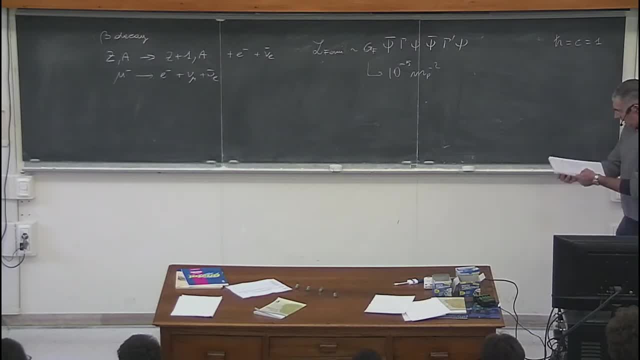 we will see in a moment why. Ok, so it was soon clear that weak interactions do not commute, to use the language of quantum mechanics, with the parity inversion operator. Parity is not conserved by weak interactions, which means that weak interactions distinguish left from right. 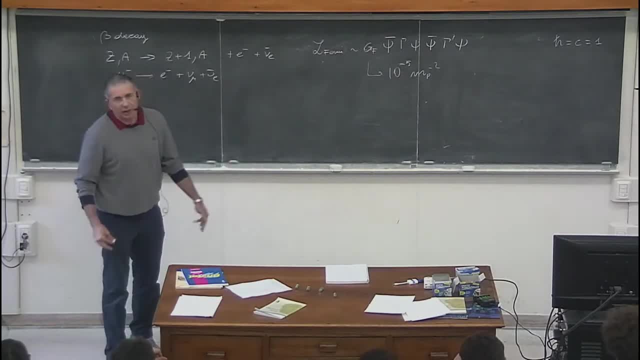 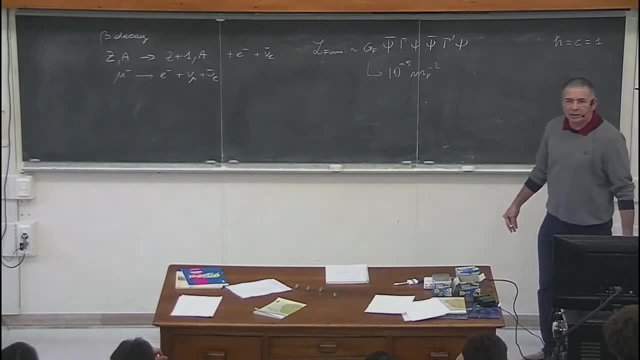 in a maximal way. There is a very long and interesting story of the experiments that lead early experimentalists to this conclusion. I will not go through it. Anyway. the precise form of the Fermi-Lagrangian and in particular of these two 4x4 matrices which appear. 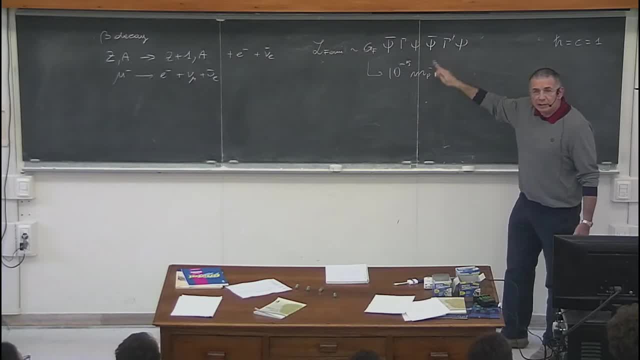 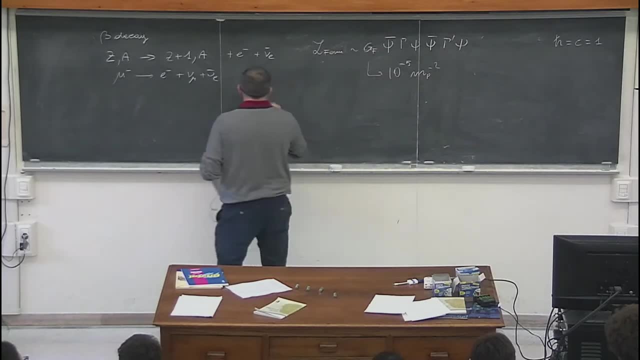 here is completely determined by the observation that parity is not conserved in weak interactions, and the final form of the Lagrangian density- let me copy it in order not to miss any factor of two is something like this constant, which is traditionally defined with a root of two in the denominator: 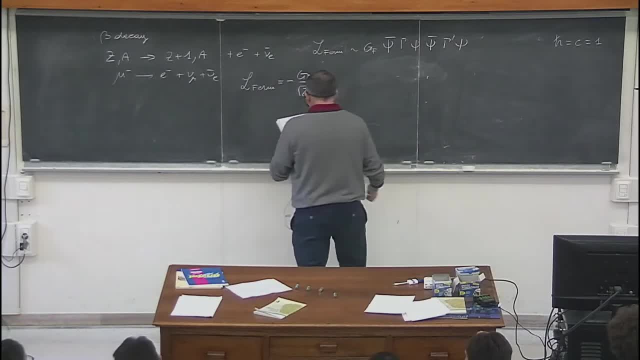 don't ask me why. and then there is a product of two currents. you will see in a minute why I call them currents. you need a creation operator for the proton, so you need a psi bar for the proton field times, the combination gamma mu times one, plus a constant gamma five. 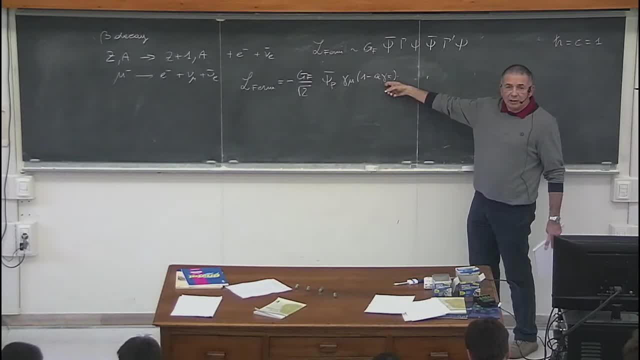 the presence of this gamma five is what signals violation of the parity operator times a Dirac field which contains the destruction operator for a neutron and the rest of the Lagrangian is given by psi bar. we need to create an electron. so sorry, this is an n. 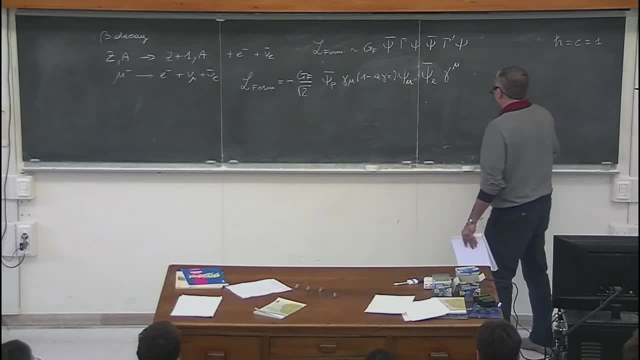 not a mu, psi bar gamma, mu one minus gamma, five times an operator which contains the creation operator for antineutrinos, which is psi. this constant a is there because of reasons which are not of our concern at the moment, but it is rather close to one. 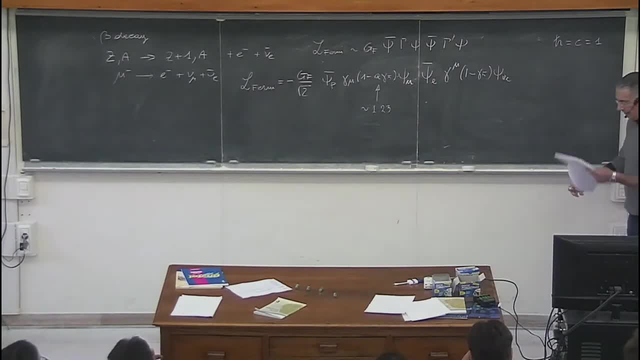 actually. and that's it, and it is a useful. obviously there is another term in the Fermi Lagrangian, which is the one which describes the decay of the muon, is something like minus g fermi divided by root of two. we need to destroy an electron. 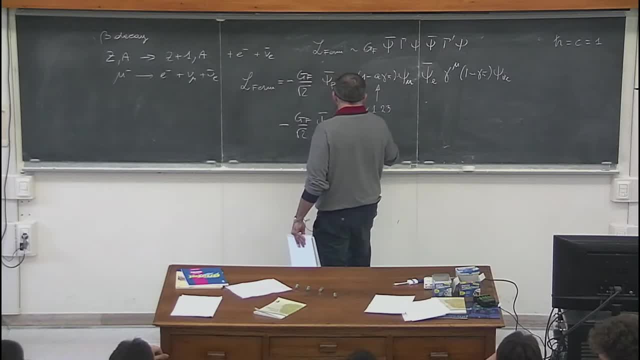 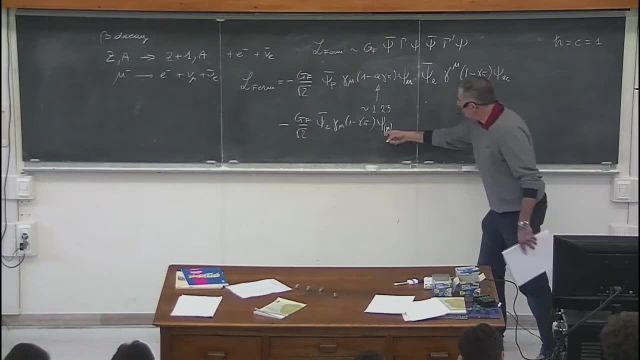 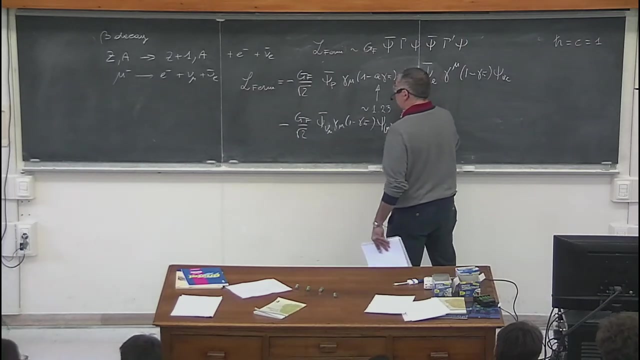 psi bar e gamma mu, one minus gamma five times the destruction operator for the muon. I put it in brackets to distinguish it from the index times. sorry, mu mu mu. and then I have to create an electron psi bar e gamma mu, one minus gamma five psi. 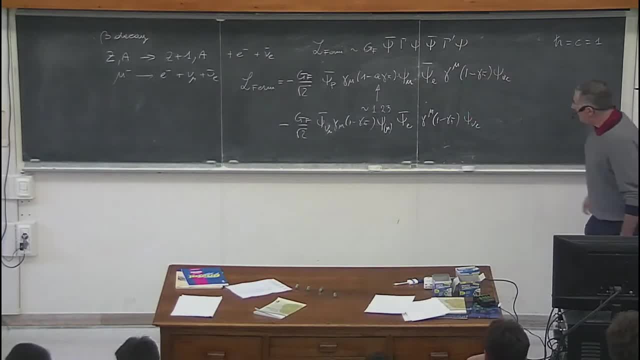 mu e and these operators, one minus gamma five, as you probably know, have the role of projecting the Dirac field onto the left-handed components, left chirality, fermion fields describing the massless limit, left-handed, left elicity states, physical states. so it's an interesting 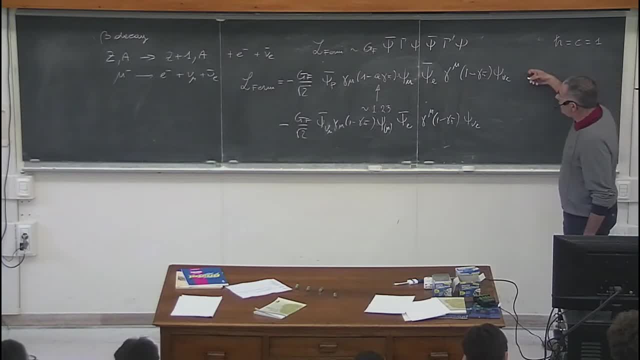 exercise to compute the lifetime of a neutron and the lifetime of a muon, given this Lagrangian density, and to observe that, given the measured values for these two lifetimes, the lifetime of the neutron is around fifteen minutes, while the lifetime this neutron- the lifetime of the muon- is around. 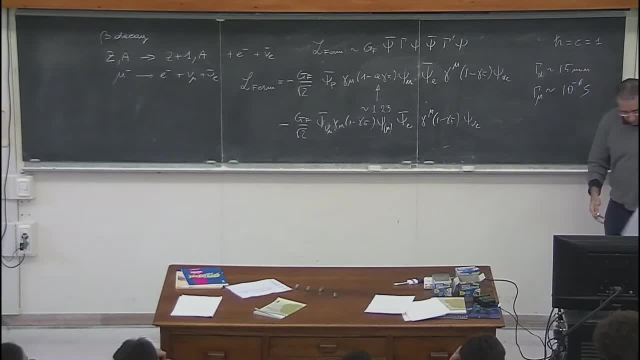 I don't know: ten to minus six seconds, something like that. I didn't write it down, but something like that. these are very different from each other, but the point is that the phase spaces involved in these two processes are also very different and the same value of the coupling constant. 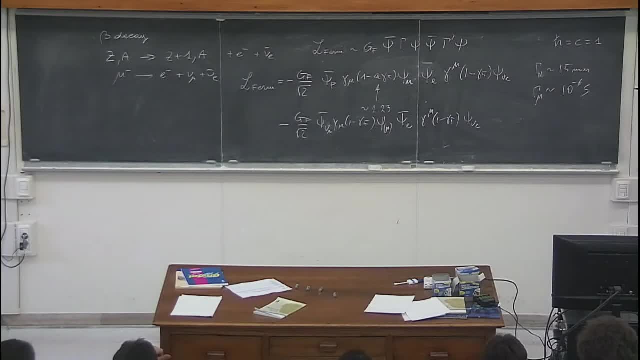 here signals the fact that both processes are governed by the same kind of interactions. we will probably figure out how to compute these quantities in the tutoring lectures anyway. so the Fermi Lagrangian describes correctly these two processes and we could be happy with that, were it not. 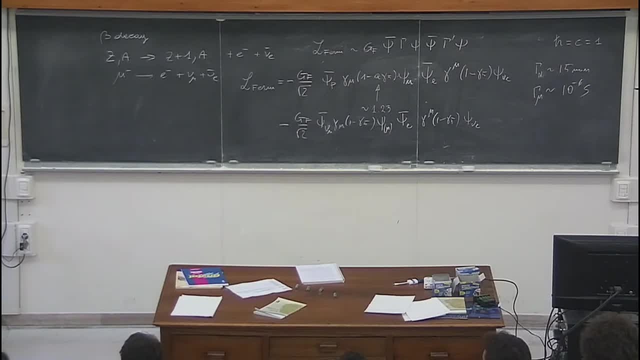 for a couple of observations, and this is also something we can discuss during the tutoring lecture in more detail. the point is the following: the Fermi theory of weak interactions is not a renormalizable theory. renormalization is a complicated subject. I will not go through it. 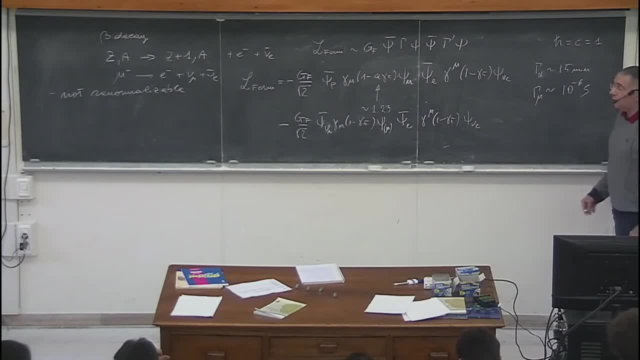 anyway, there is a simple criteria, necessary criterion to decide whether a field interaction term in the Lagrangian density gives rise to a renormalizable perturbation theory, and the criteria is to count the dimension of the field operator. if the dimension of the field operator appeared in the 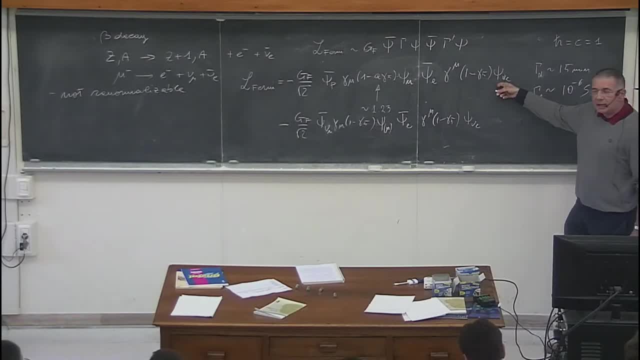 interaction term exceeds 4- the dimension of space-time- then the theory is not renormalizable. so only dimensionless or couplings with dimension of a positive power, of an energy, of a mass are allowed to appear in a renormalizable theory. here the coupling constant is not. 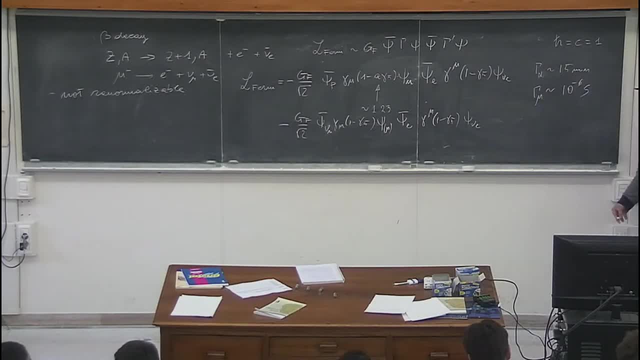 has the dimension of an inverse square mass, so the theory is not renormalizable. and perturbation theory: it is not possible to use perturbation theory beyond leading order. this is an effective theory. you will have lectures on the subject of effective field theories during this same week. 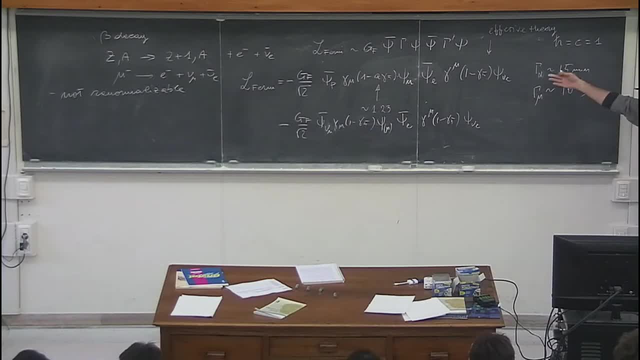 and this is appropriate, because the Fermi theory is the first and most known example of an effective field theory, which means a field theory which is valid only up to a given value of the energy involved in the process you are considering. why am I talking about energy? I am talking about energy. 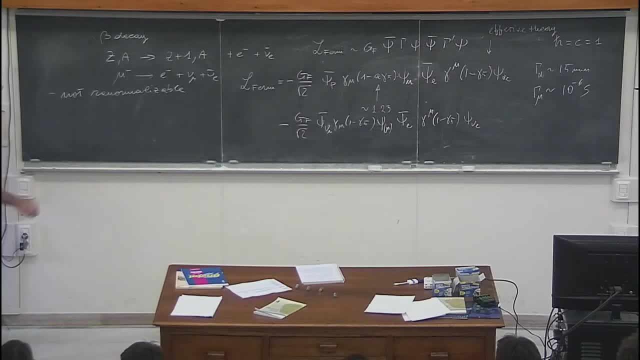 because non-renormalizability of the Fermi theory is closely related to non-unitarity of the Fermi theory. non-unitarity is what was first observed historically and this means that if you you know that the scattering matrix in any field, in any acceptable field theory, 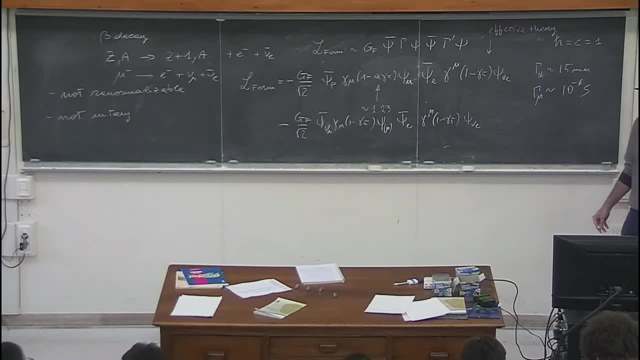 must be unitary. the S matrix is a matrix which connects in and out states in the scattering theory and in and out states two different bases on the same Hilbert space of states. so the connection matrix must be a unitary matrix and the constraint of unitarity 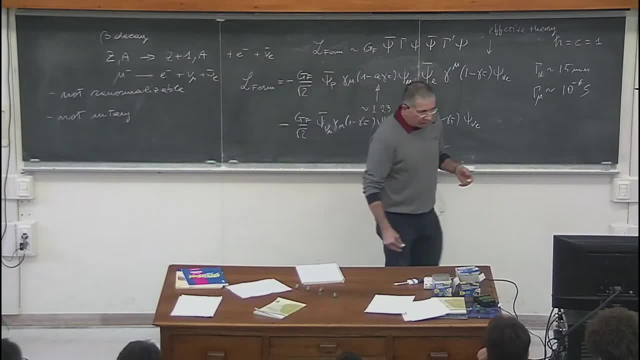 which is, as you know from basic quantum mechanics, amounts to the constraint of conservation of probability. so it is a very basic thing- is violated by the Fermi theory. roughly speaking, the reason is again related to the dimension of the coupling constant, since there are two powers of a mass in the denominator. you have to compensate for that with some power of kinematical invariance, and that amounts to the fact that some cross section grow with energy and if you go to sufficiently high energies, you will end up with amplitudes which violate the constraint of perturbative unitarity. 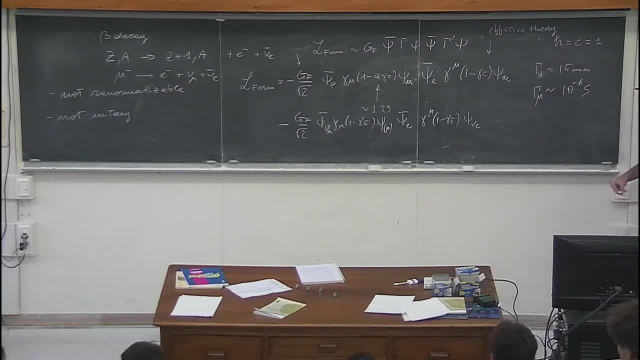 so the Fermi theory is an effective theory, which means that it works perfectly well as far as you are concerned, with processes at sufficiently low energies, but at some value of the energy- we will see which values of the energy- it is bound to fail at some point. 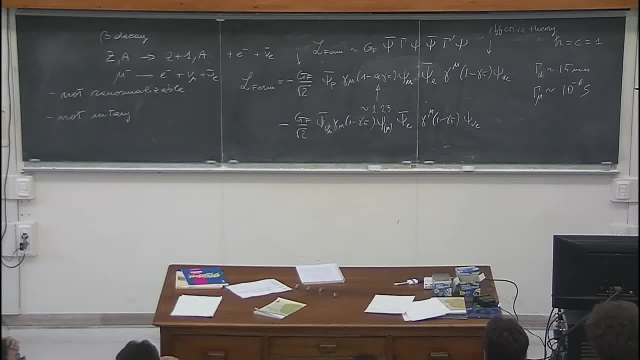 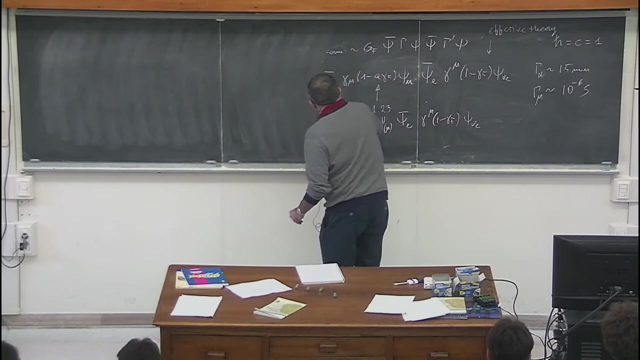 so we would like, for both conceptual and phenomenological reasons, to have a renormalizable and unitary theory of weak interactions. so this is the idea which is at the basis of the birth of the unified theory of electroweak interactions, at the time when 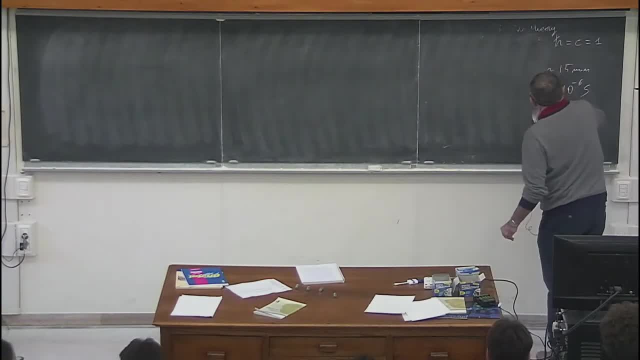 weak interactions were discovered and first studied. an example of renormalizable theory was already attended, which was QED. in QED you do not have any interaction vertex with four fermion insisting on the same vertex, but you do have four fermion interactions, except that they are mediated. 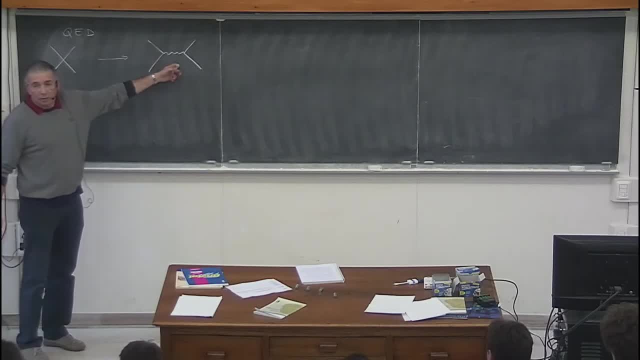 by the exchange of a vector boson. I guess you all are familiar with this kind of of diagrams. it is customary to use solid lines for fermions and wavy lines for vector bosons, and the vector bosons which is relevant in QCD is the photon, of course. 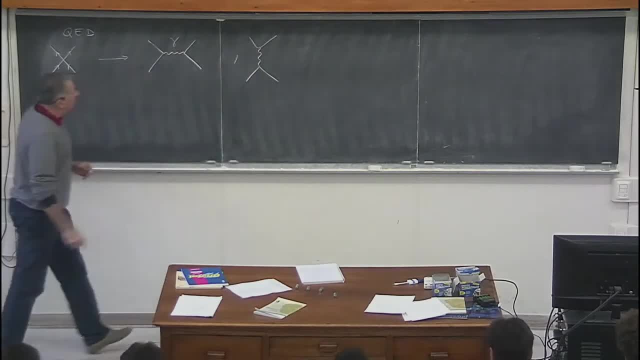 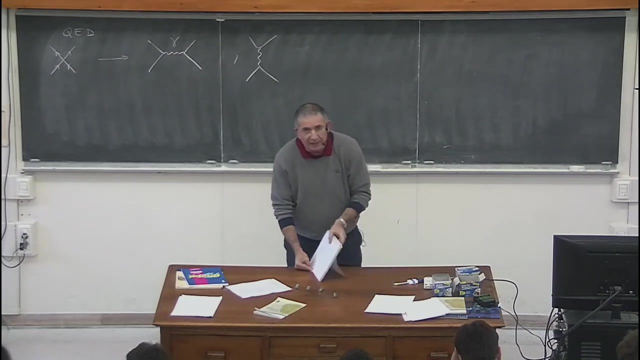 you may have even diagrams like this. so in QED, which is a renormalizable field theory, four fermion interactions are arise from the exchange of a vector boson of a vector boson. so it was very soon recognized that something like that must be done. 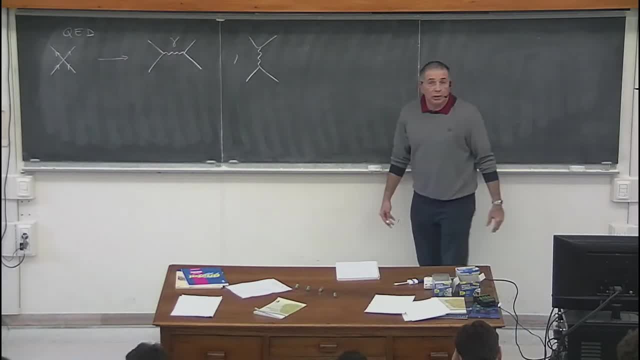 in order to transform the fermi theory into a renormalizable theory of weak interactions. however, it was also very soon recognized that, while the photon is a massless particle- which was at the time and today- even today recognizes the origin of the fact that electromagnetic interactions 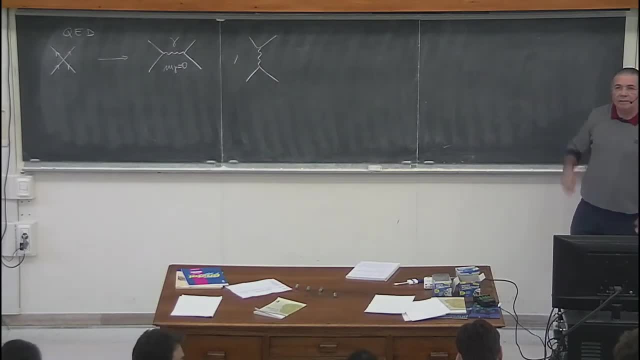 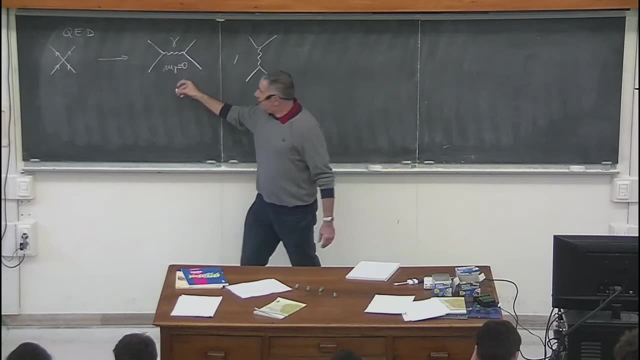 are long range interactions. they can be transmitted at very long distances because of the fact that the photon is massless is related to the fact that the static potential of the photon can be transmitted at very short distances. for example, if you look at weak interactions, you recognize that weak interactions. 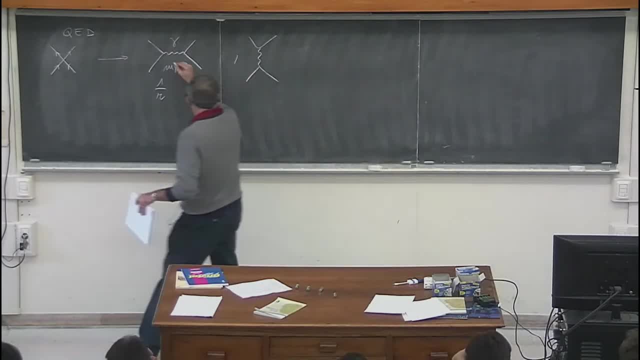 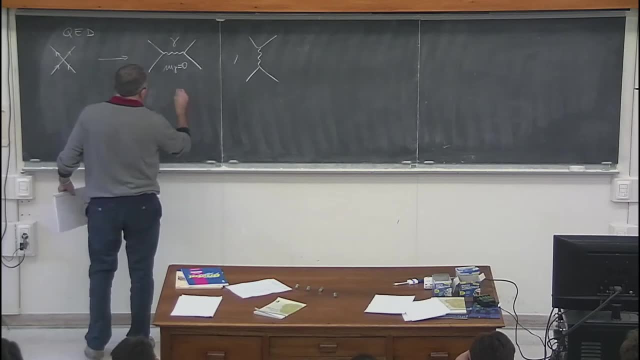 are very shortly ranged, and the easy way to see this is that the presence of a propagator like this gives you a factor, which is the distance between two forces divided by q squared, which is the propagator of a vector boson with zero mass. here q is the difference. 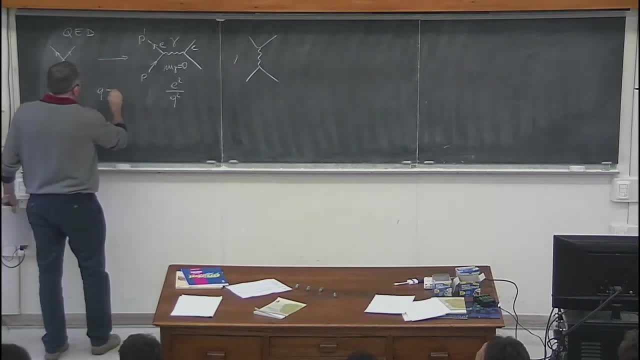 the momentum transfer. this is p and p prime, outgoing p prime. q is p minus p prime, while in the case of the fermi theory you can see that if you multiply the spinors connected to the four external legs, which means that if you replace this four fermion vertex, 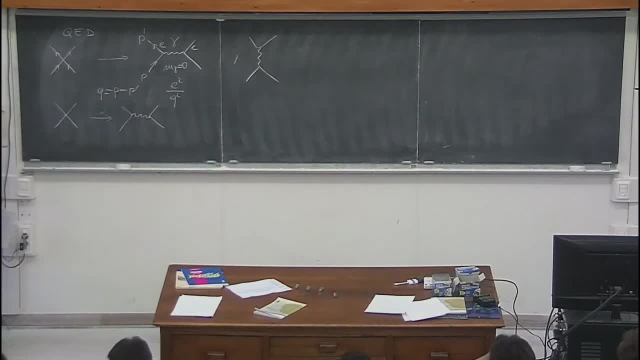 by the diagram with the exchange of an hypothetical vector boson mediating weak interactions. this must be related to a factor like this: a propagator of a massive vector boson with q squared much less than the square of the mass of the weak vector boson. 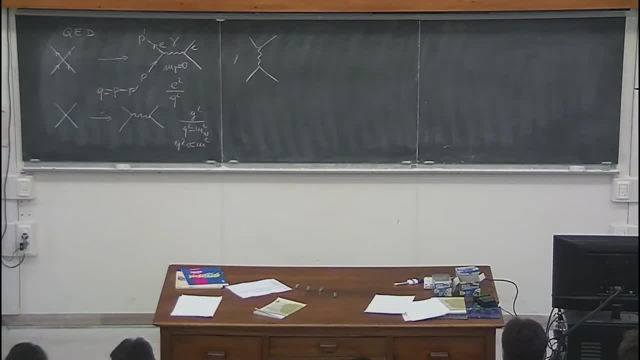 let me call it w, as it was done very soon. w stands for weak, and if the, the vector boson mediating weak interaction, is heavy enough, then this propagator can be replaced by a constant with the dimension of an inverse square mass, so by this rough. 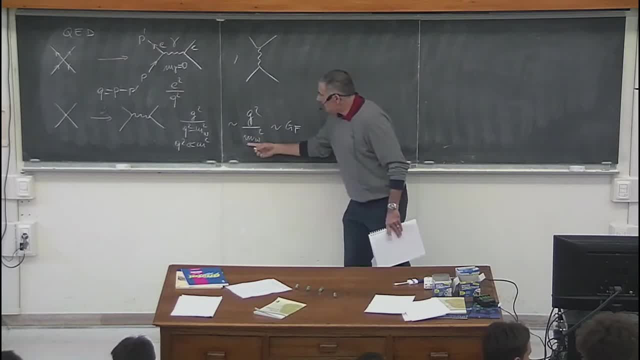 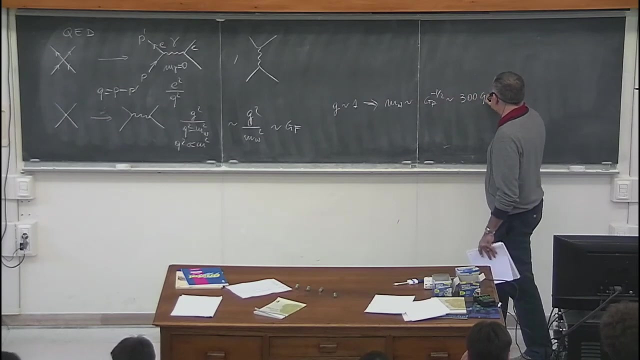 argument you can infer some estimate of the value you expect the weak vector boson to have. for example, if you take the coupling constant g to be of order one, you get mw of the order of the inverse root of the fermi constant, which means 300 gv. 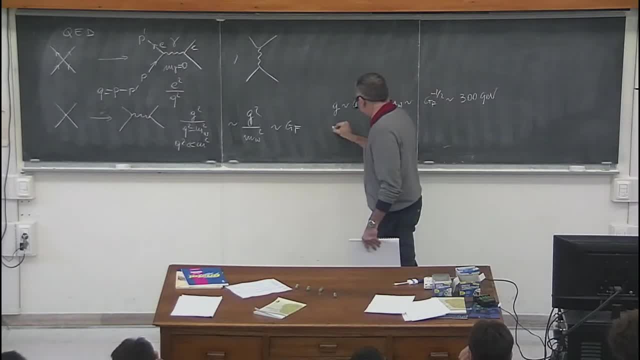 if you, on the other hand, assume, for some reason, the coupling constant g to be of the same order of the proton charge, which is what we will actually see to be true, then you get a slightly smaller value of the mass of the vector boson, which is around 100 gv. 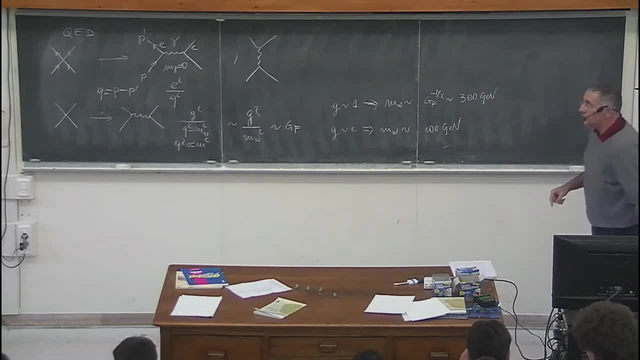 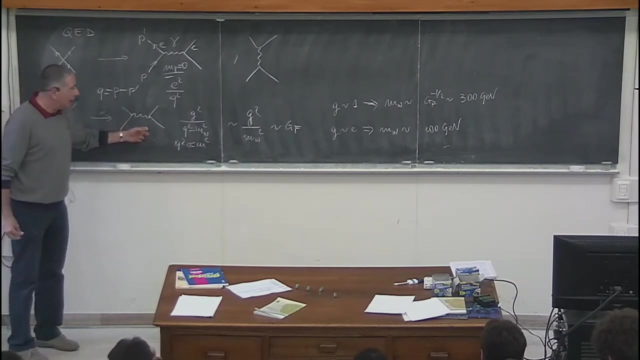 anyway, enormous number, enormous numbers compared to, for example, to the mass of the proton, but the value to which you have actually to compare them is the value of the photon mass, which is zero. so we want to build a theory of weak interactions, where weak interactions are mediated by the presence. 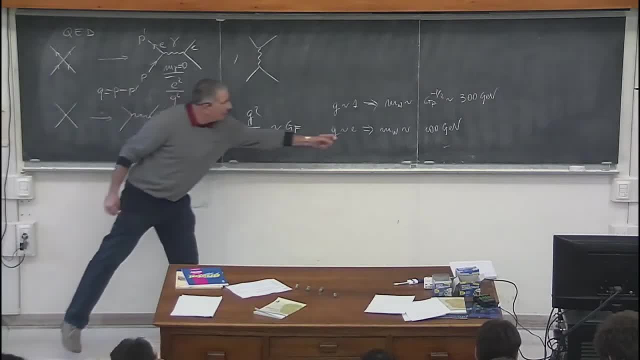 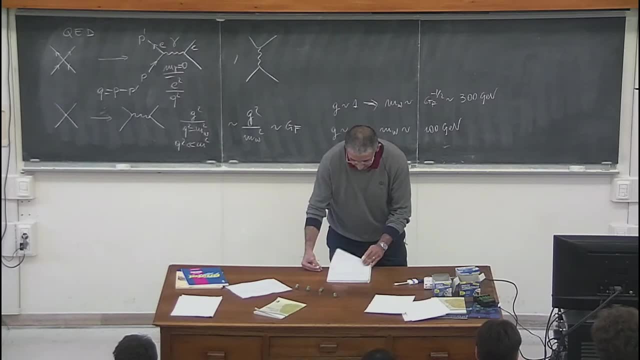 of a vector boson, but this vector boson must be a massive one. this was recognized very, very soon in the history of weak interactions, actually the reason why at first it looked like there was no hope to to build a renormalizable field theory for weak interactions. 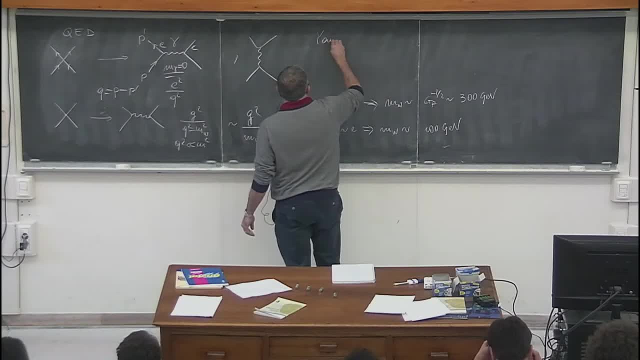 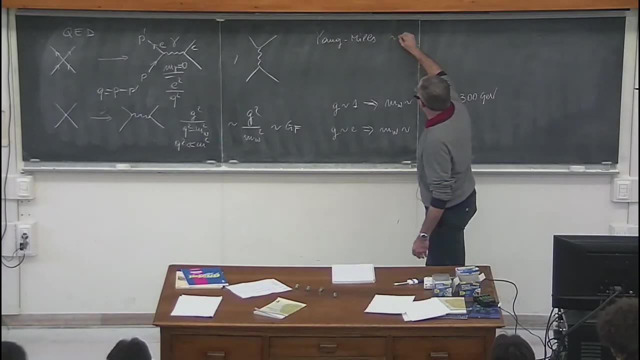 because the young mills construction, which is the construction of field theories with a gauge invariance based on abelian invariance groups- this dates back to 1954. write it down and in the young mills construction mass terms are forbidden. young mills, the gauge invariance as in QED. 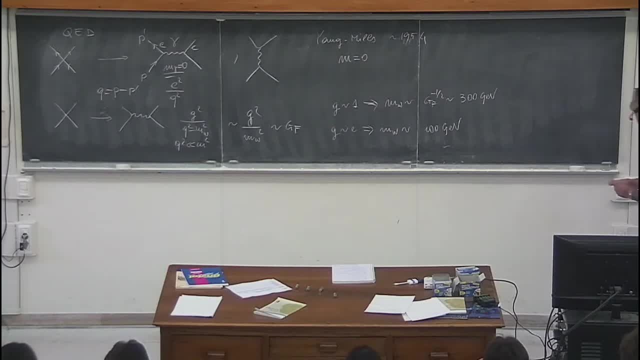 gauge invariance forbids masses for the vector boson. anyway, let me for the moment ignore this relevant and important problem and let me go ahead and try to build a field theory of weak interactions which is based on the idea of gauge invariance, gauge invariant field theories. 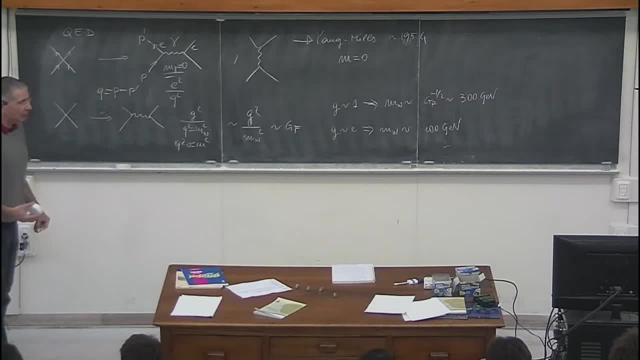 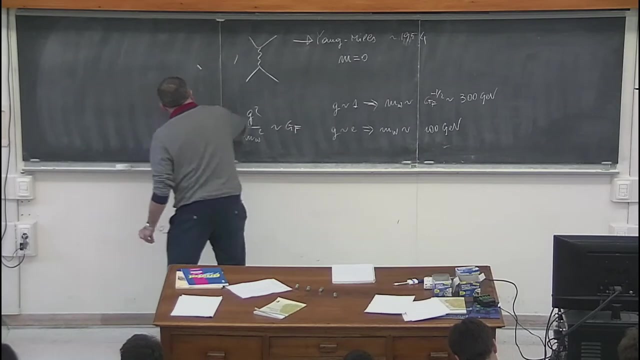 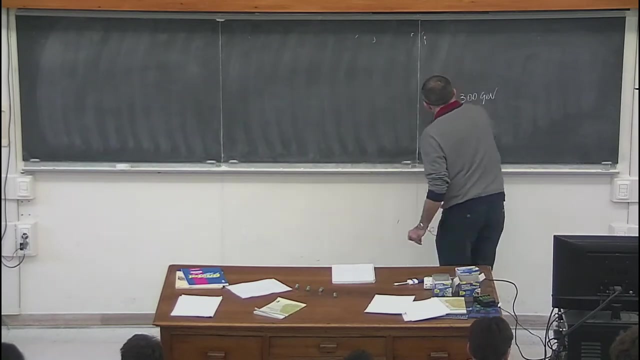 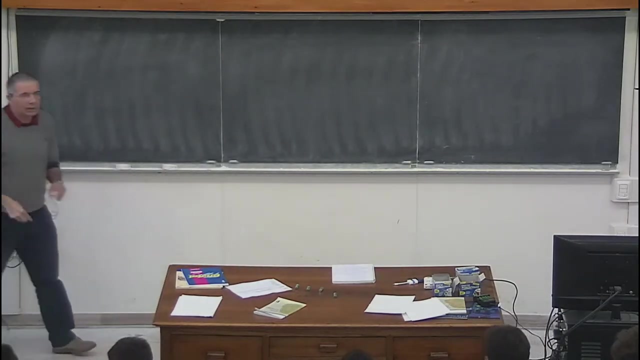 even in the non abelian case, were already known to be renormalizable and unitary, and I will solve at some point the problem of the mass of the weak vector bosons. so in order to build a gauge theory of weak interactions, I have to do two things. 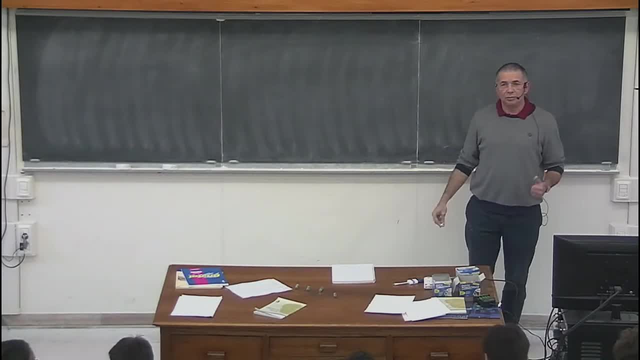 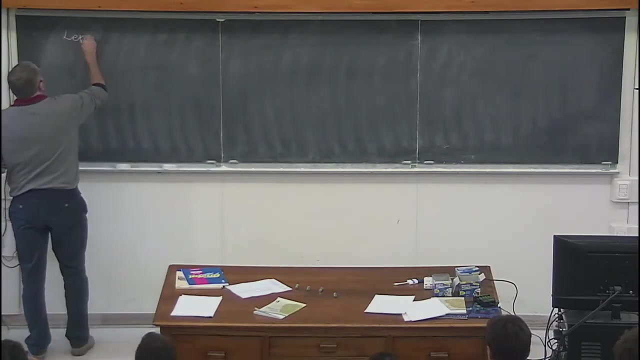 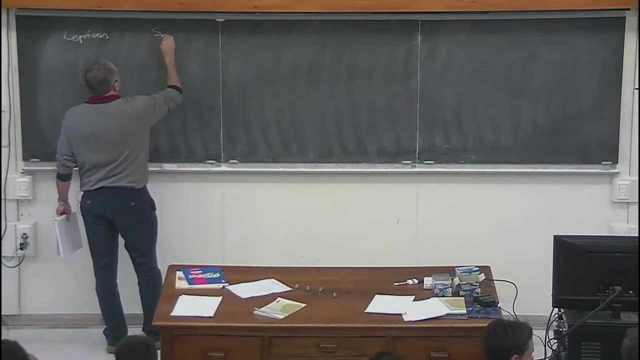 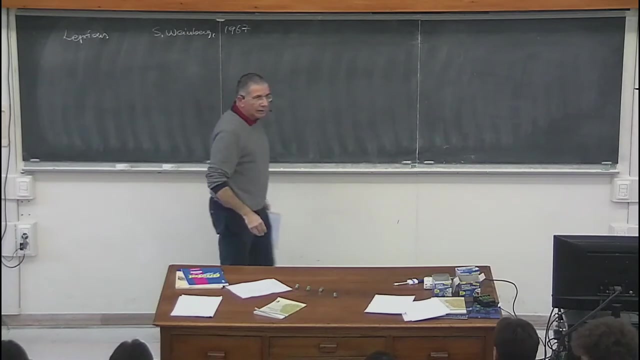 first I have to identify the invariance group and then I have to assign fermion fields to representations of that gauge invariance group. and I will do both things, starting from the lepton sector. the paper by Steve Weinberg, nineteen sixty seven, his title is: 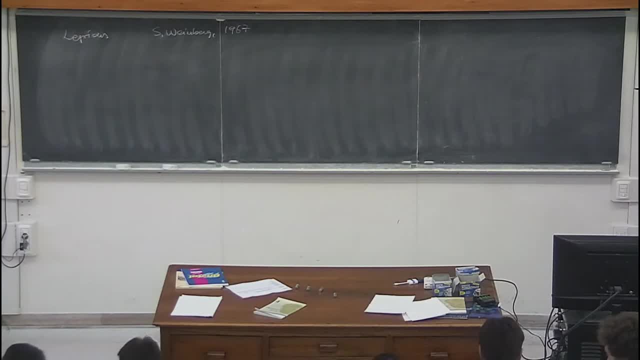 a theory for leptons. he started with the lepton sector, which is easier. we will see that hadrons pose different problems anyway, leptons. let me write down again the Fermi Lagrangian in the lepton sector. this is given by. I just wrote it down. 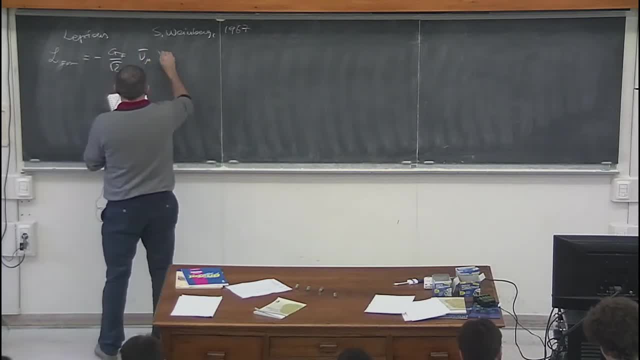 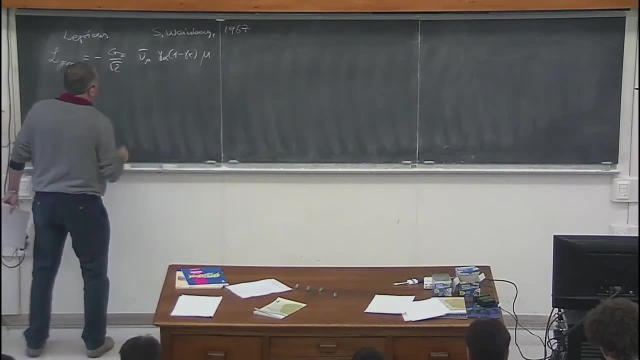 g fermi over root of two mu bar mu, alpha one minus gamma, five times mu. let me change slightly notation: instead of psi nu, I just write mu. instead of psi mu, I just write mu. I just use the symbol of the particle for the fermion fields. 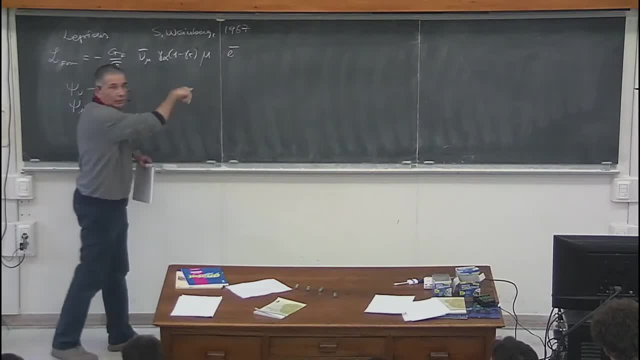 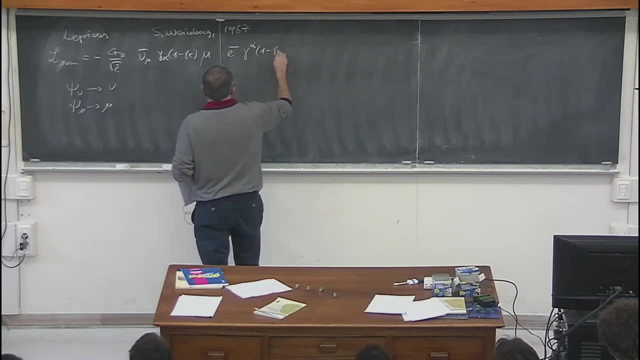 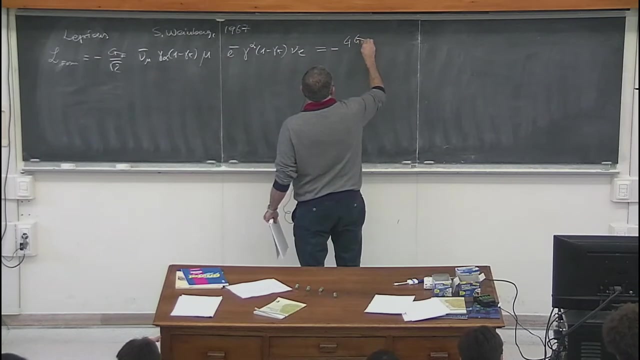 in order to save writing times, e bar e bar now stands for the fermion field, for the electron times one minus gamma five, mu e. this is the Fermi Lagrangian for mu decay, and this can be written in the following form: minus four g, f over root of two. 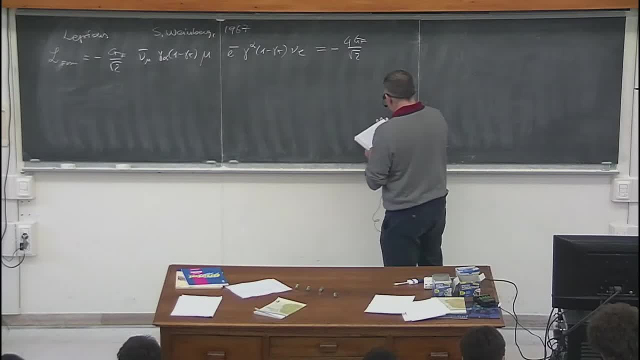 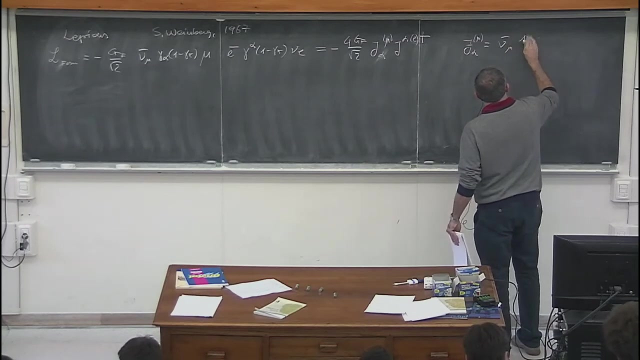 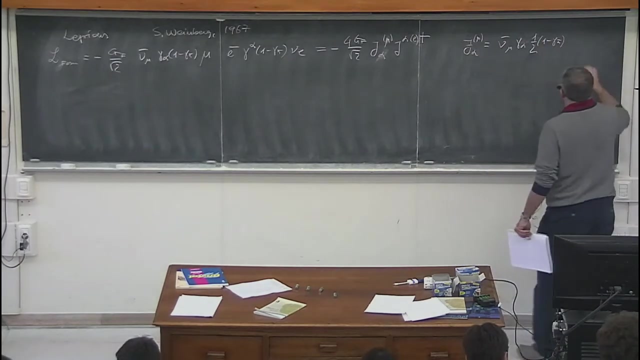 you will see in a moment the reason of this extra factor of four times j mu e, j mu, sorry, alpha mu, j alpha e fermion conjugate, where I have defined j alpha mu to be mu bar mu, gamma alpha one half minus one minus gamma five. 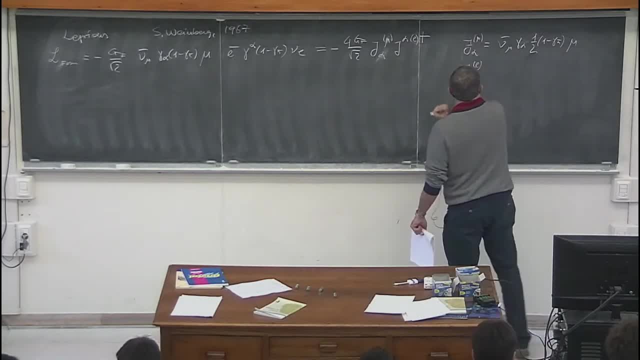 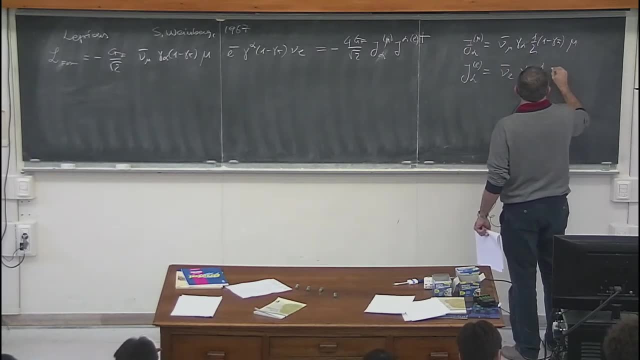 times mu and j. alpha for the electron is just the same thing: u bar e. gamma alpha one half one minus gamma five e. I have inserted this factor of one half here in order to have a projector. this is a true projector, an operator which is equal to itself. 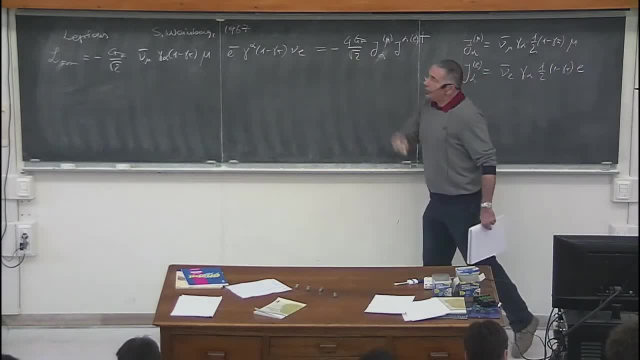 when you take its square. so I pay a tax of a factor of four. okay, so this is just an identity. I have defined these two objects, but these two objects have now the appearance of another current, of a current which is related to some invariance of the theory. you know that in field theory, 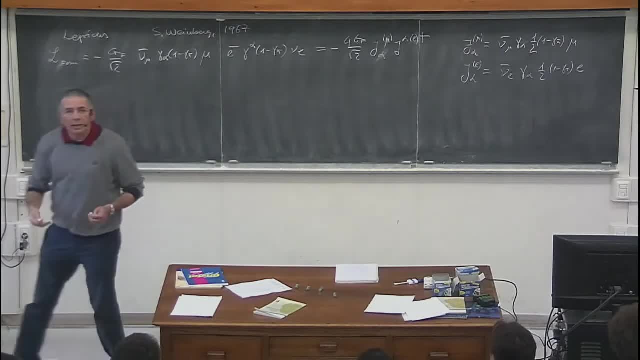 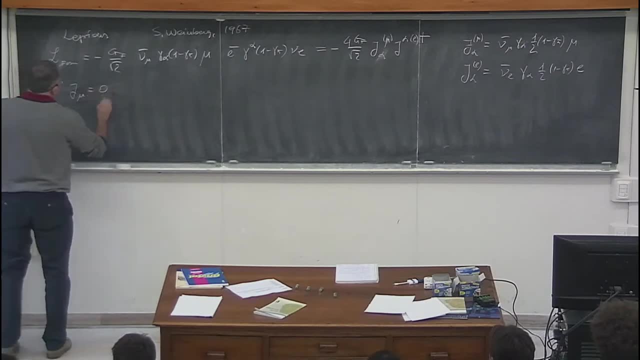 when you have an invariance property, then you have a way to construct conserved current current which satisfy the continuity relation mu j mu equal to zero, which corresponds to the conservation of the space. integral of the fourth component of the time, component of the of the current. 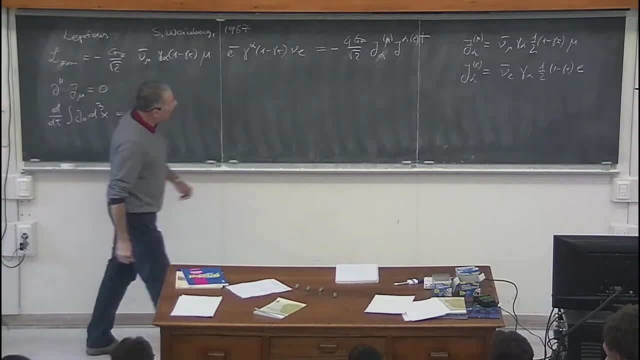 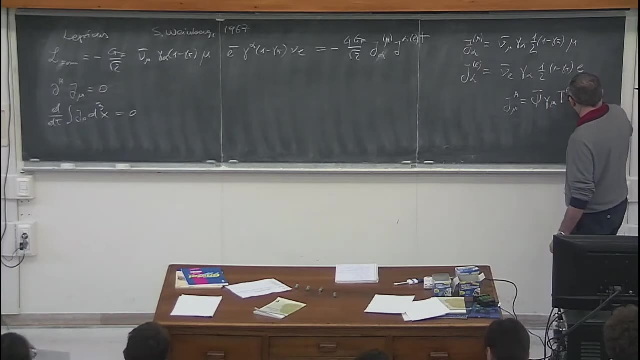 so current related to fermion fields have the following form: that for a generic collection of fermion fields in a given representation of the gauge group of the invariance group, you have a conserved current for each generator of the gauge group. a is an index which labels: 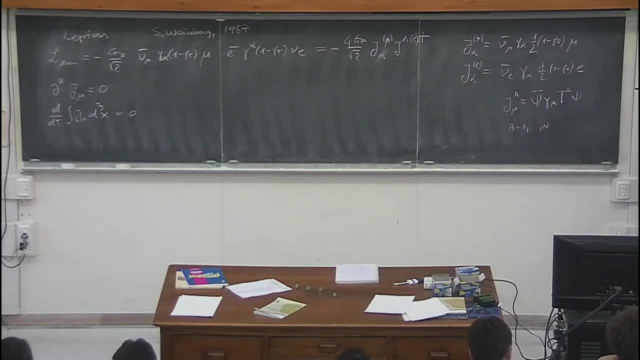 the generators of the algebra of the gauge group and for each of them there is a conserved current and the ta are the generators in the representation of the fermion fields, psi. if you are not familiar with this language, we can discuss it in the afternoon or during the 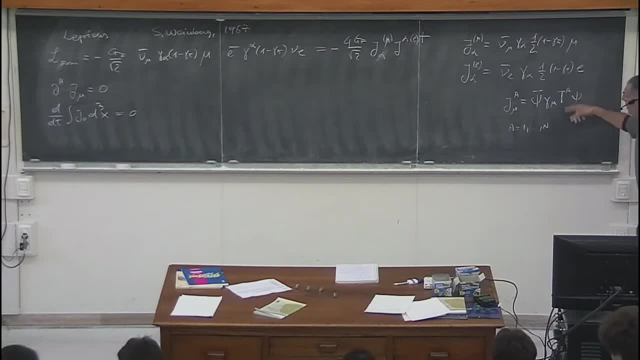 tutoring lectures. anyway, i will assume that you are all familiar with this idea. so my purpose now is to cast these two currents in the form of another current for a gauge invariant, and this is easy to do. this can be done in many different ways, but the simplest way. 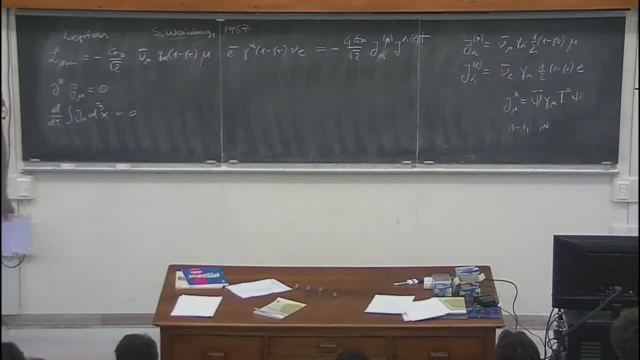 the way which was suggested by Steve Weinberg, and which turned out to be the correct way, actually is the following: first of all, let me observe that, for example, the electron current can be written like this: you can insert an extra factor of one half one minus five. 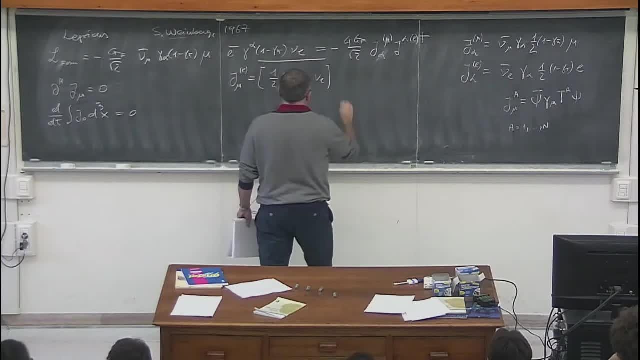 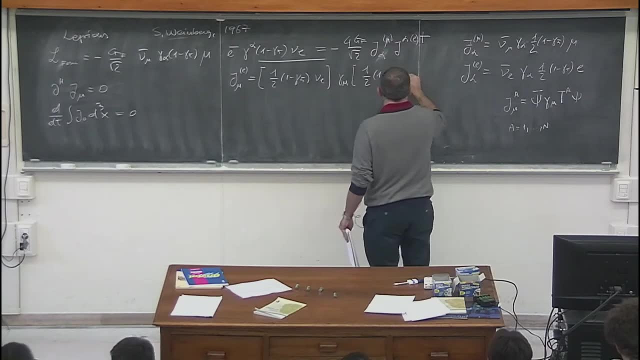 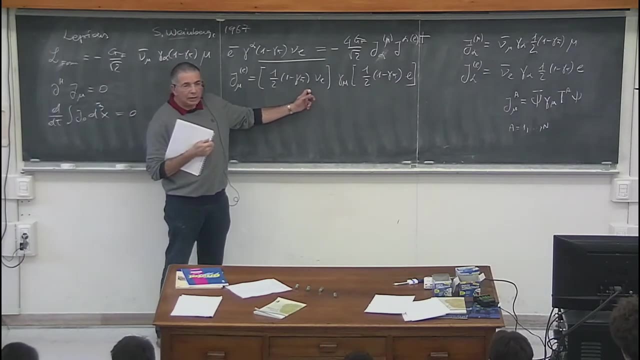 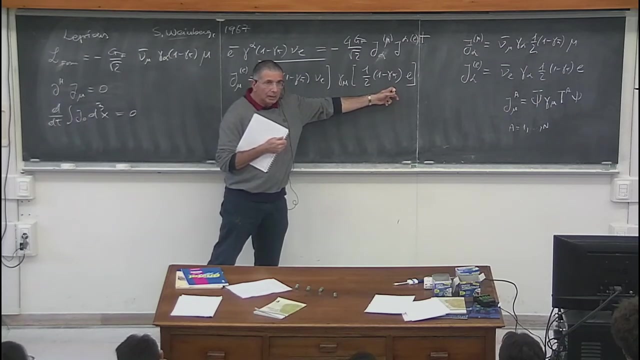 here because gamma five anti-commutes with gamma mu and anti-commutes with the gamma zero which is hidden in the Yirach conjugation. you can also insert an extra factor of one half one minus five, so in the end it is multiplied with one half one minus gamma five. 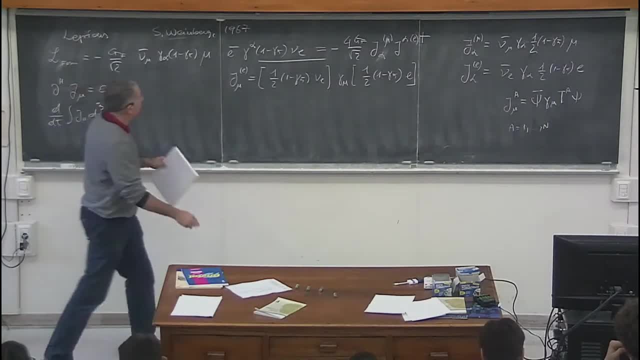 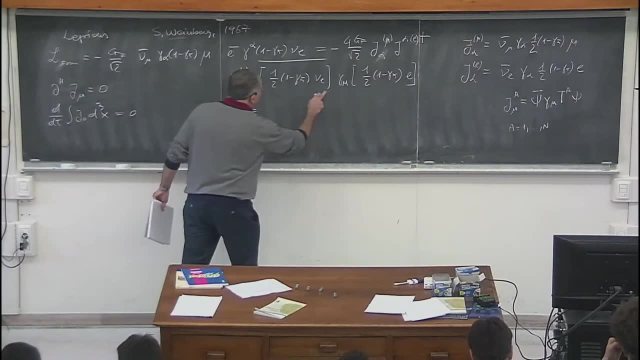 which gives one. so these two currents, the two currents appearing in the Fermi Lagrangian, can be written in terms of the left-handed components of the two Fermian fields only. this is nu bar left, gamma, mu e left, and the same is true for the other two currents. 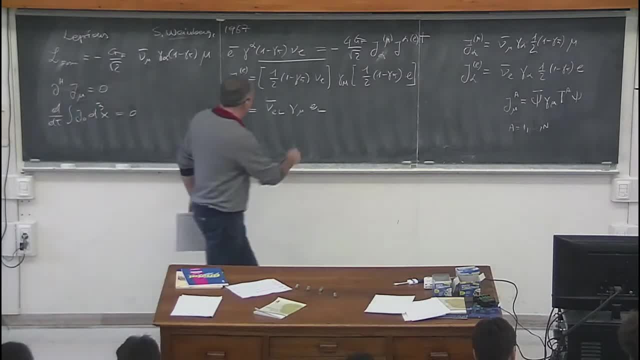 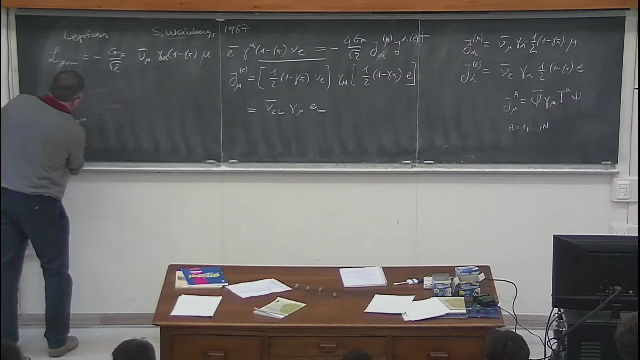 so it turns out that only left-handed components of the Fermi fields are relevant for the Fermi interaction, for the interactions described by the Fermi Lagrangian. so simplest and in the end correct idea is to define a doublet of left-handed fields. let me call it: 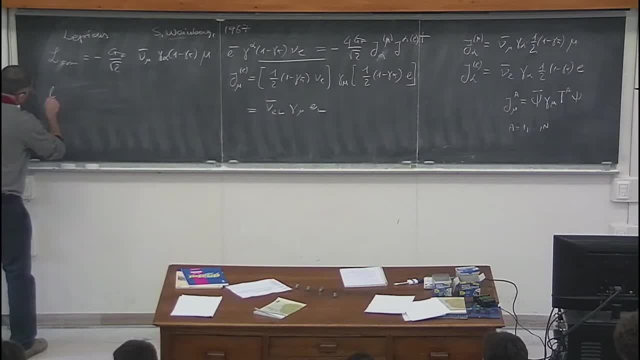 L, this script. L stands for lepton and this capital L stands for left. and this doublet is formed out of the left-handed component of the electron neutrino and the left-handed component of the electron Fermian fields. this is the doublet for the electron family. 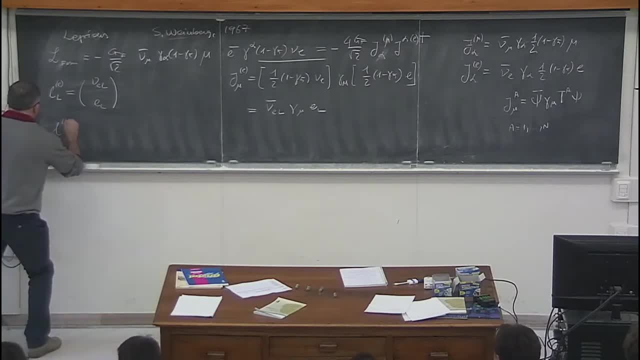 there is a similar doublet for the muon family, which is formed with the left-handed component of the muon neutrino and the left-handed component of the muon Dirac field, and you will agree with me that this current here can be written like this: 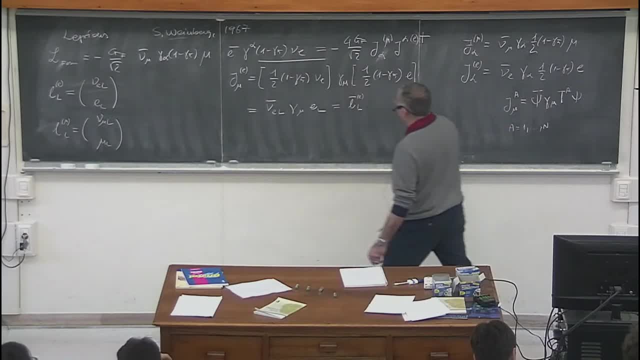 L bar for the electron left-handed gamma mu, a two by two matrix, which I call tau plus times the doublet and tau plus is zero, zero, zero, one, zero, zero. this is an identity. this is very trivial. this equal sign here is just a consequence of this definition. 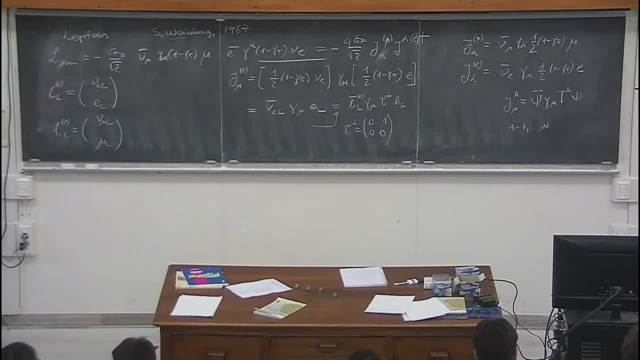 and the definition of tau plus. but if you do that, you have succeeded in casting the current in the form of a neutral current. you see, there is a fermion field, actually a doublet of fermion fields, actually a doublet of left-handed fermion fields. 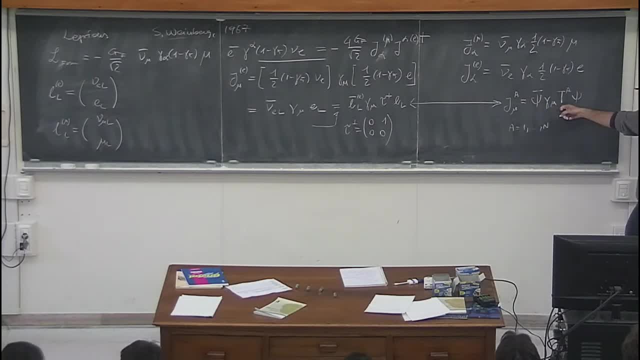 gamma mu is fine, a matrix which I am now interpreting as one of the generators of the gauge invariance group I am looking for, and the same collection of fermions. so this is the simplest idea. I will also have to include the Hermitian conjugate. 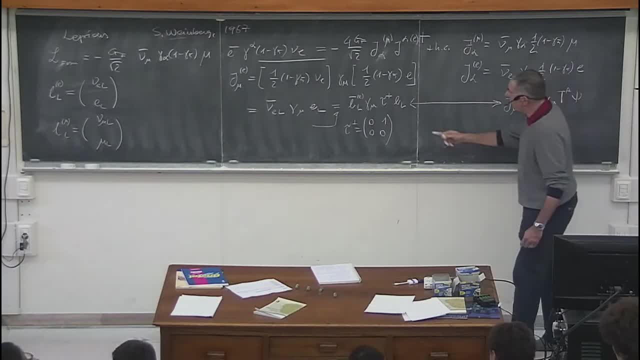 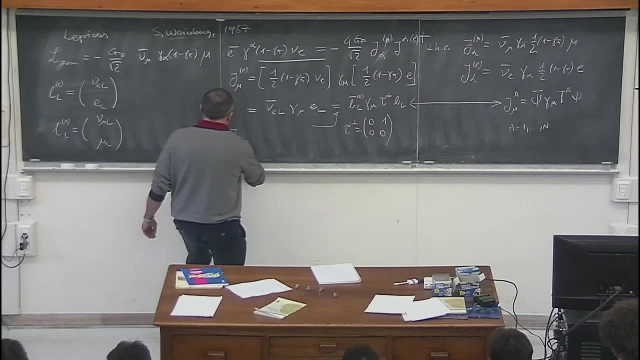 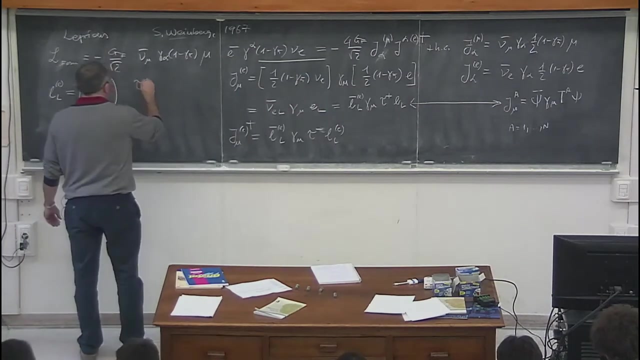 of this Lagrangian term, which means that there will be the Hermitian conjugate of this current. and if you just take the definitions, you easily find out that the Hermitian conjugate of this current can be written like this: tau minus and tau minus. 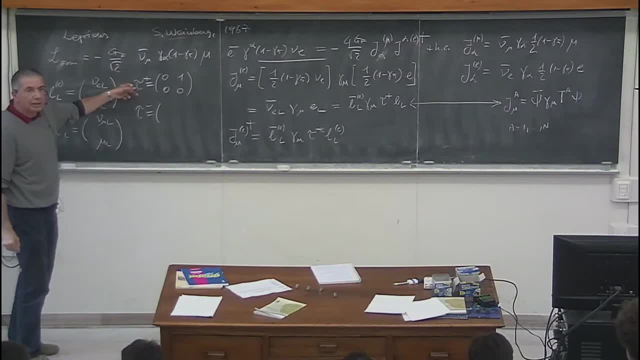 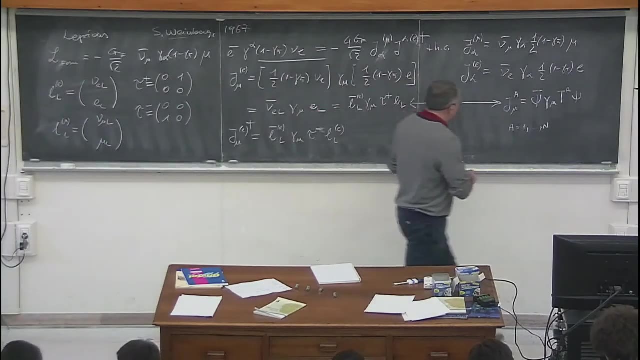 is the Hermitian conjugate of tau plus. but tau plus is real matrix: 0, 0, 1, 0. how do we go on? well, you probably remember that the generators of the algebra of a Lie group are closed under the commutation operators: the commutator. 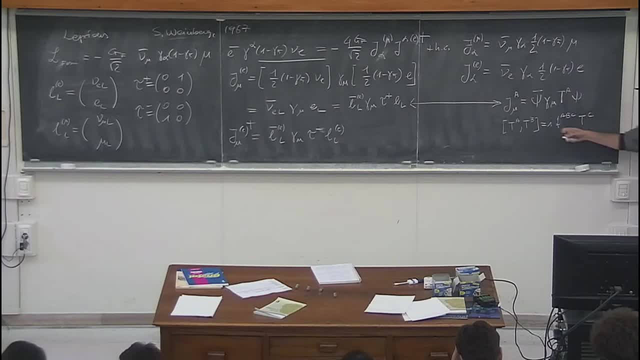 of two generators is a linear combination of the generators themselves. so if tau plus and tau minus are to be interpreted as generators of a gauge invariance group, then I will have to assume that there is a third current, which I call J mu 3, which is the current. 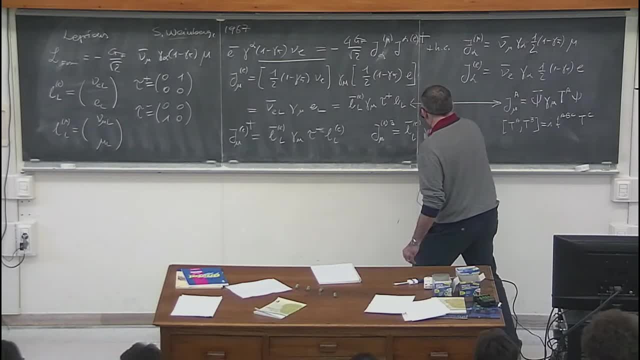 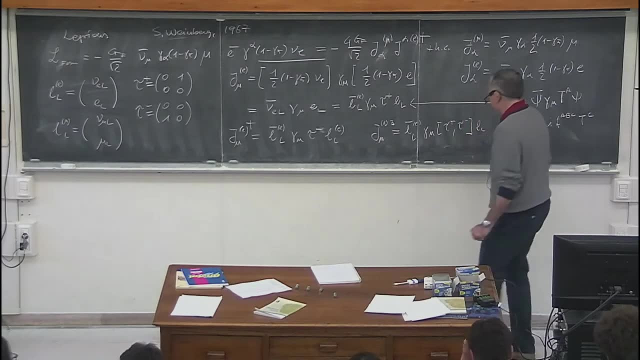 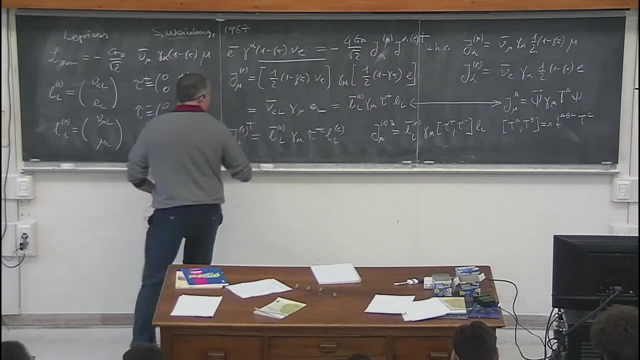 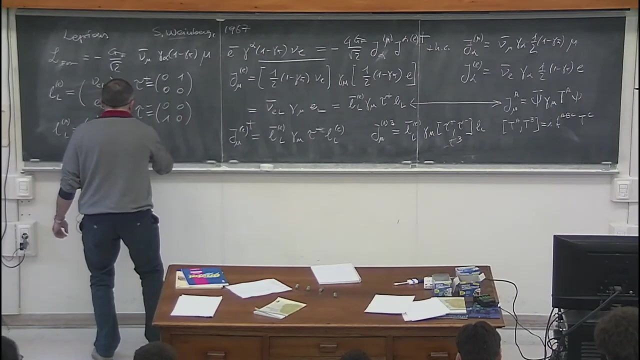 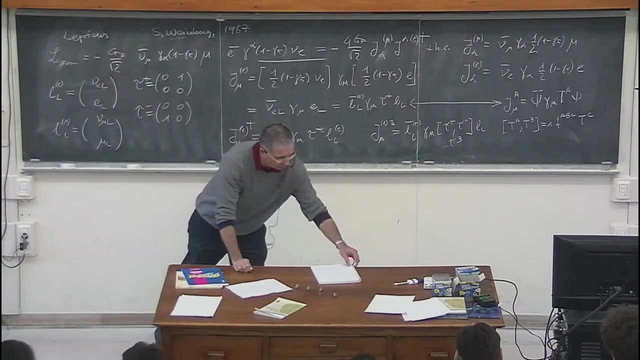 built out of the commutators, the commutator of tau plus and tau minus, and the commutator of tau plus and tau minus is easy to compute. I can do it here. this is what I call tau 3 and tau 3, sorry, yeah. 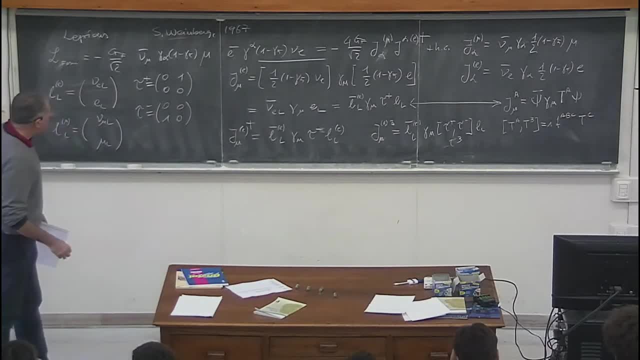 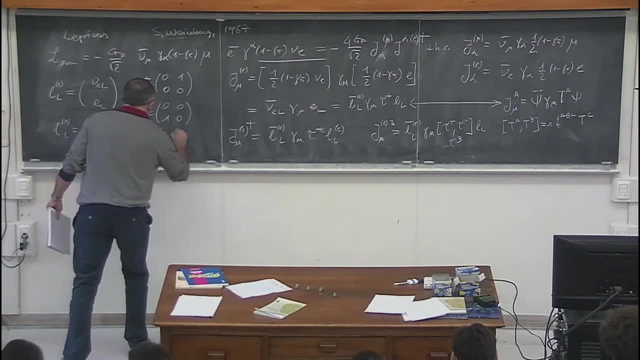 this is what I call tau 3, and tau 3 is 1 0, 0 minus 1. I am not going to compute the commutator in front of you because, ok, we are not done yet, but now we have to check that taking the commutator. 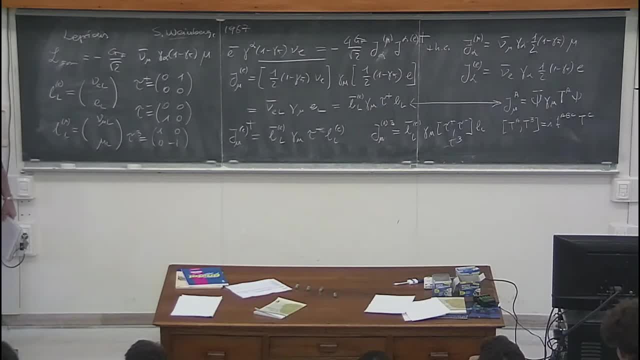 of tau 3 with either tau plus or tau minus, I don't get anything new. if I get something new, I have to include it in the commutator algebra, otherwise I am done. the algebra is closed. but now, at this point, you have already recognized this algebra to be the algebra. 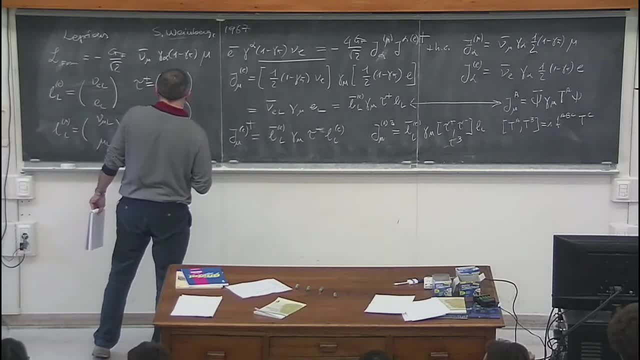 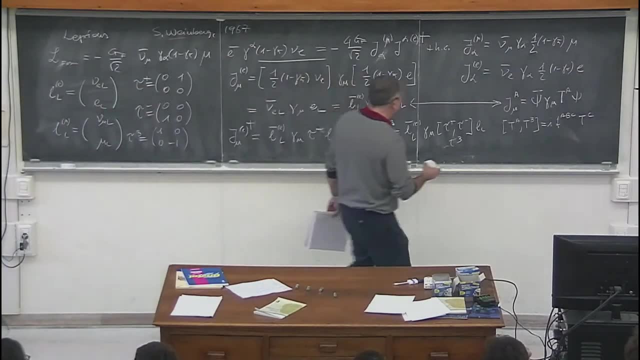 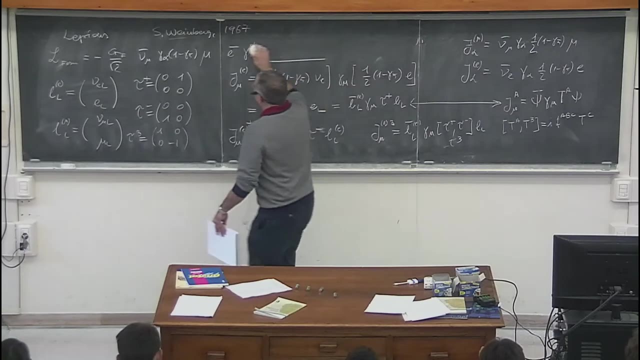 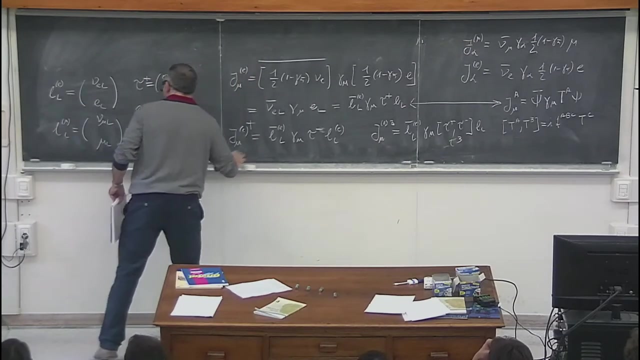 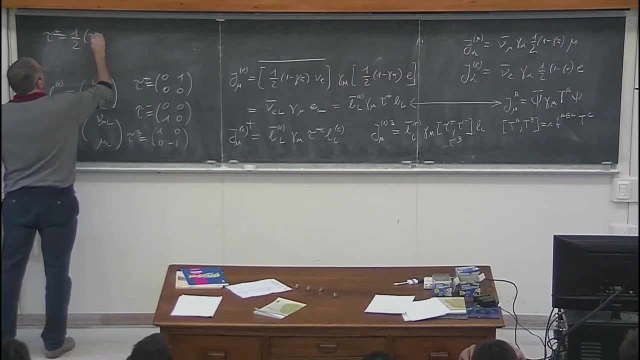 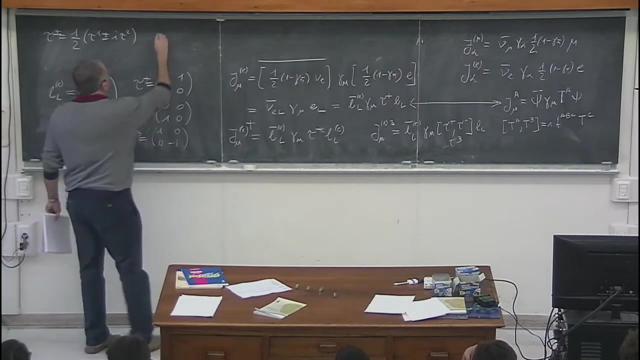 of the loop SU 2, I introduce matrices. this blackboard is too small for my. what can I erase? I can erase something here. I can write tau plus and tau minus in this form: where tau 1 is 0, 1, 1, 0 and tau 2. 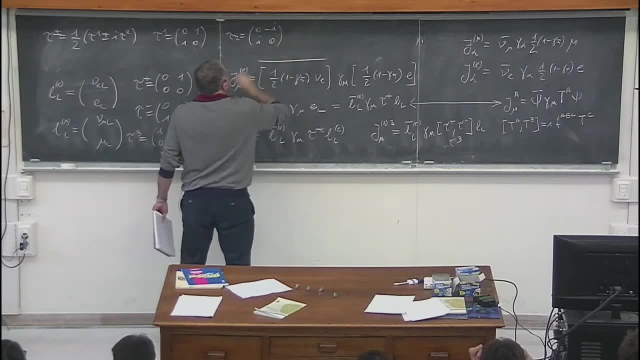 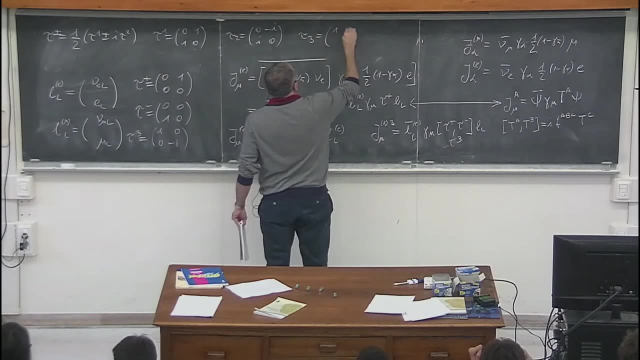 is 0 minus i i 0, and at this point you recognize the spin 2 representation of the group SU 2, which is the same group as angular momentum here. angular momentum is of no concern for us, but the algebra is the same. so what we are saying, 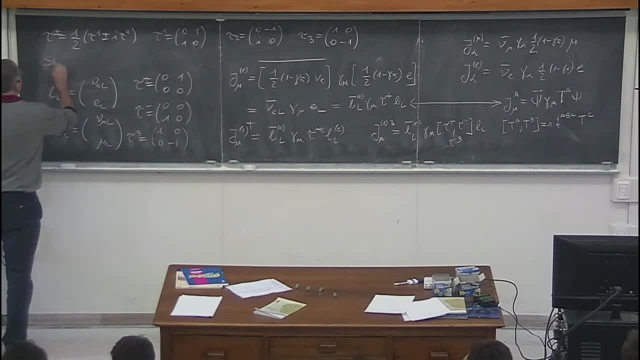 we are guessing that the gauging variance group, which is what we are looking for, is the group SU 2 and we call it SU 2 left, to remind us that this SU 2 only acts, has a non-trivial action, only on left-handed. 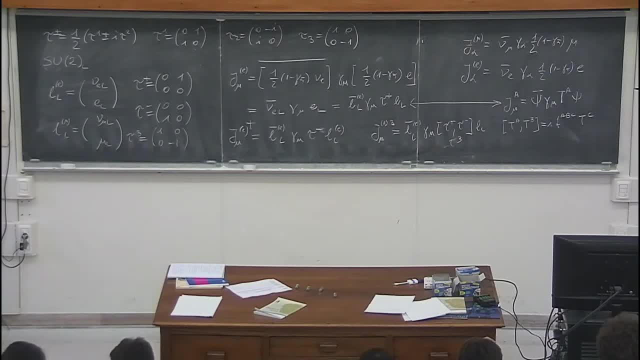 components of the fermion fields involved and the three currents which appear as a consequence of SU 2 left invariance are the two currents J mu and J mu dagger, plus the current which I called J mu 3. there is a problem, another problem we always have the problem of 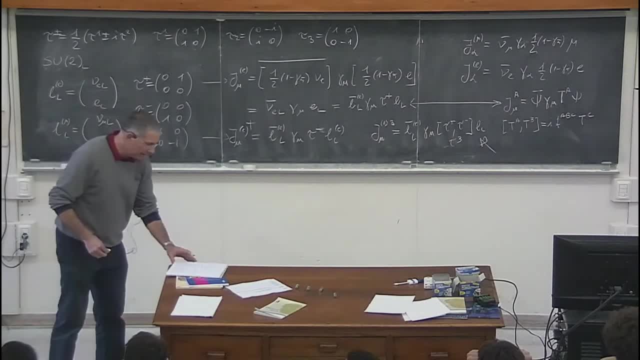 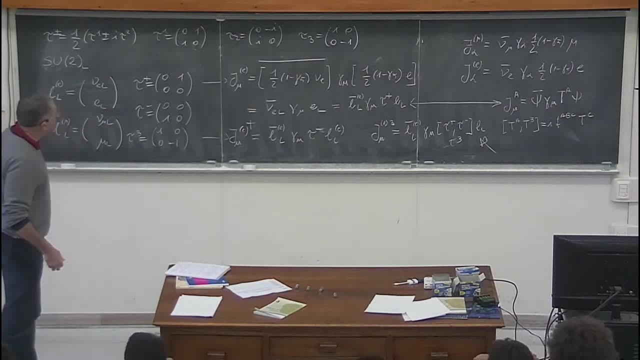 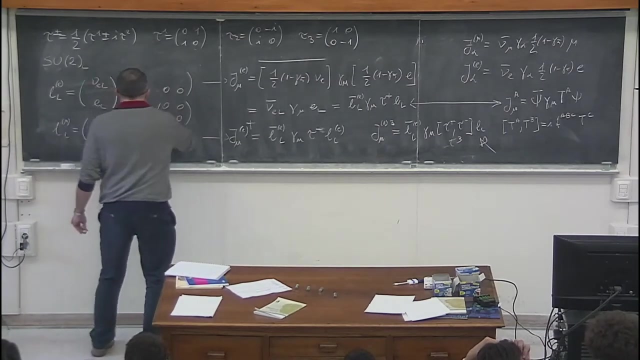 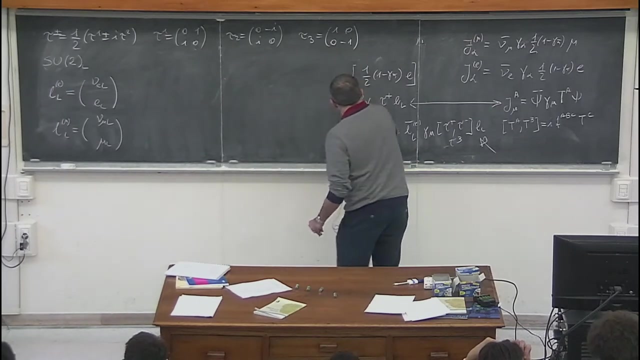 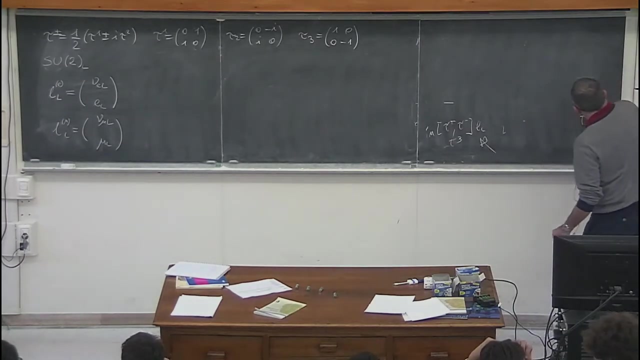 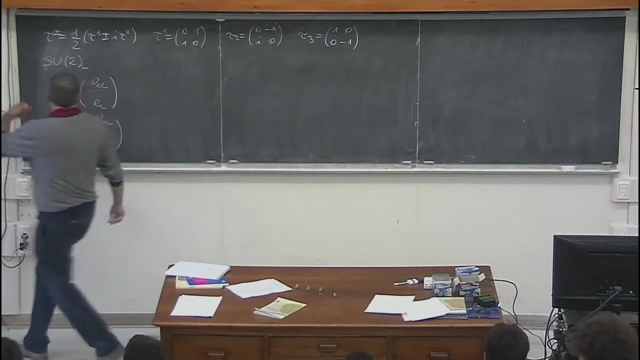 the masses of vector bosons. but now a new problem appears. well, let me, before saying speaking about the new problem, let me tell you something else. so we now have a guess about what the gauge group might be, if the Fermi Lagrangian is an effective theory. 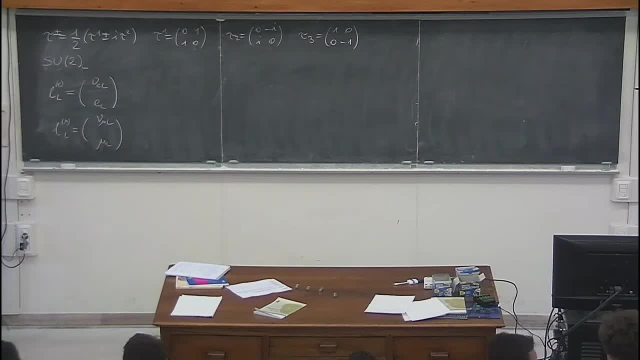 of a renormalizable gauge theory of weak interactions, I have a guess of which irreducible representation is connected to the left-handed fermion fields. the left-handed fermion fields form a doublet, a dimension, a representation of dimension 2 of SU 2 in order to complete this picture, 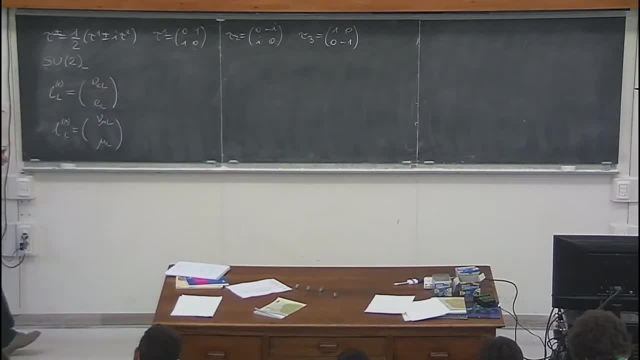 I have to say something about the right-handed components of the same fermion fields and since they do not appear at all in the Fermi Lagrangian, what I'm saying is that the right-handed components of both the neutrino fields and the electron field 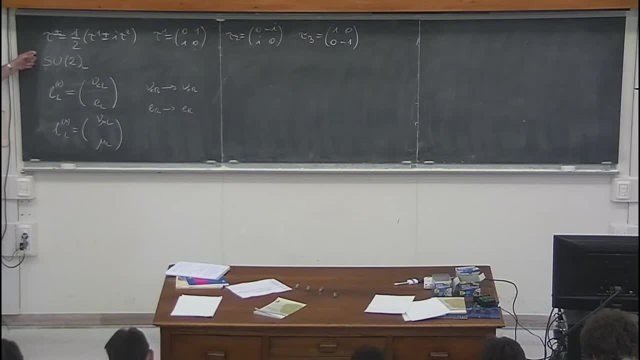 transform trivially under the action of SU 2 left. they do not transform at all. they transform according to the trivial representation of SU 2 left. this structure can be replicated. you can do, you can form a doublet out of the electron neutrino and the electron. 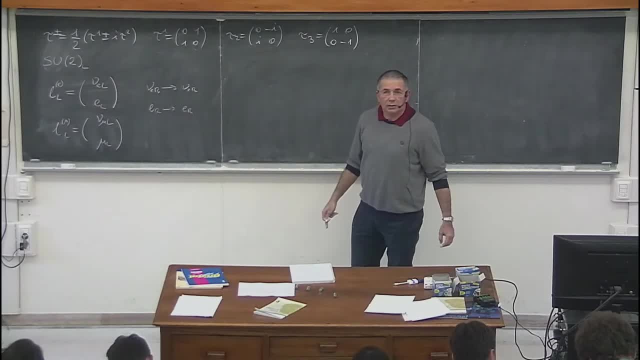 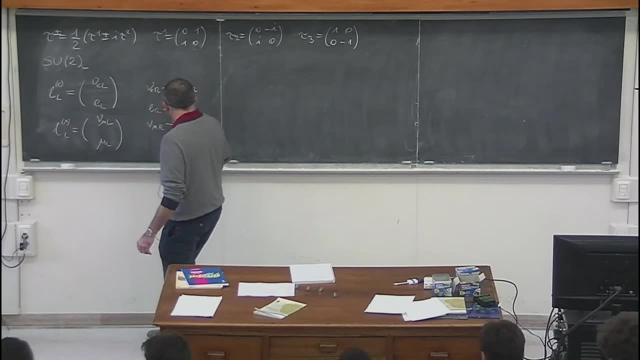 and then assign the right-handed components to singlets, and then you can do the same for the muon, and in principle, you can replicate this structure as many times as you wish, and in fact we know that there is at least one third generation of leptons. 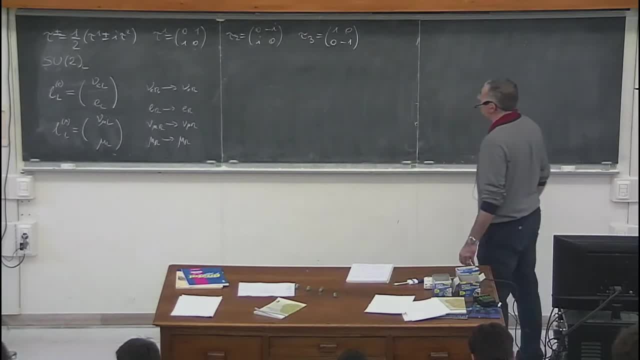 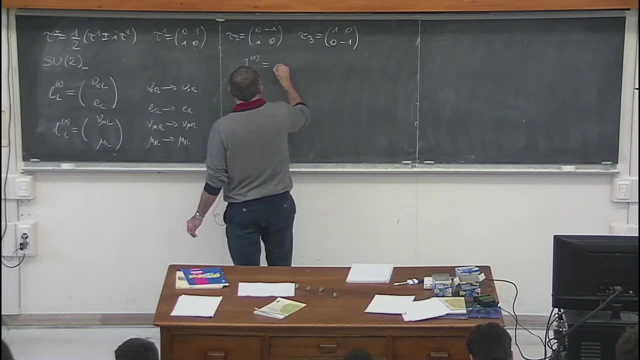 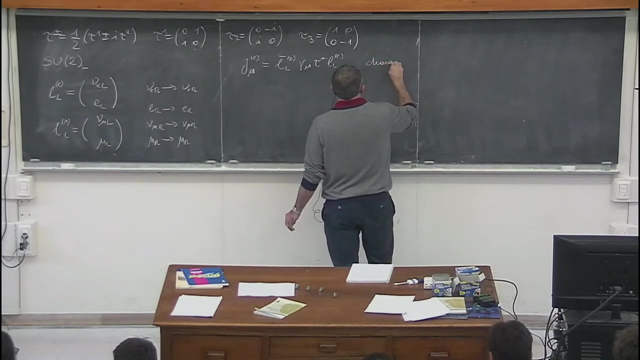 what is the problem I was mentioning? the problem I was mentioning is that what I call J mu, which is the current form of tau plus, is what we call the charge current. what do we mean by that? we mean that, if you consider it as it is, 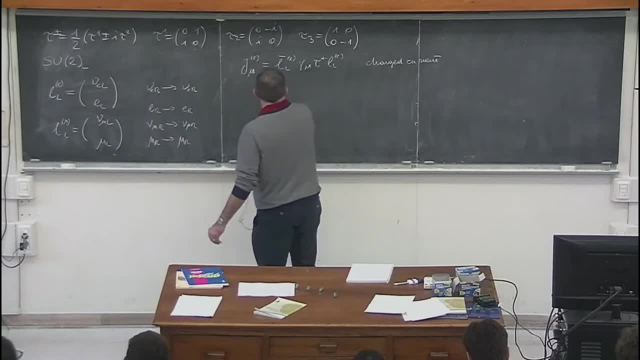 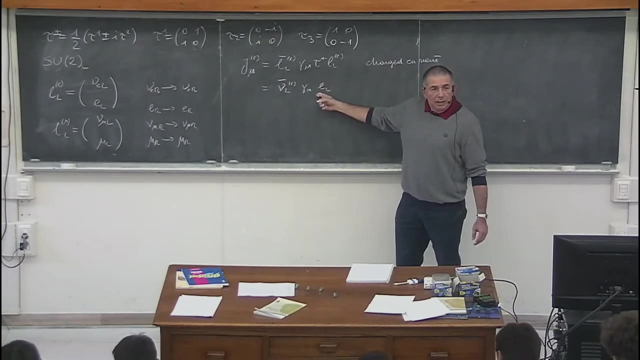 as a field operator, it contains- let me write it in the original way- nu bar left, gamma, mu e left. it contains the destruction operator of an electron, which is a charged particle, and the creation operator of a neutrino, which is a neutral particle. so as an operator when it takes on. 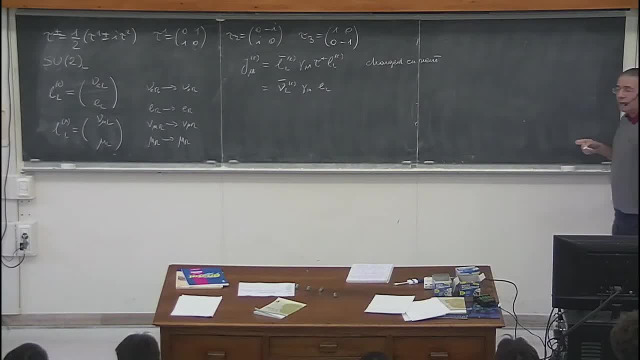 Hilbert space vectors. it changes the charge of the state vector it takes on. it is a charge, current and, as far as we know, only charged currents are involved in the Fermi theory. only charged currents are involved in the low energy weak interaction processes and, of course, 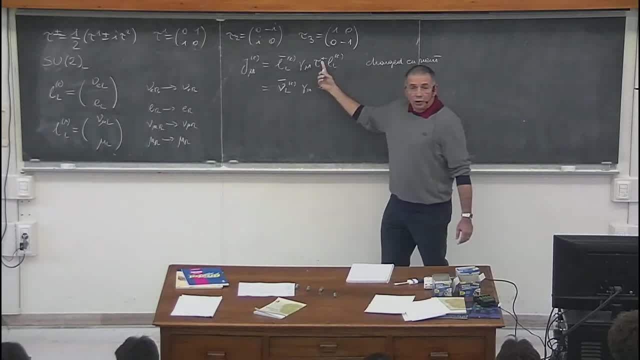 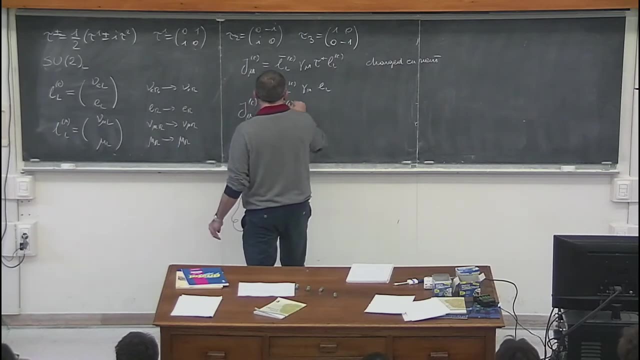 the same is true for the Hermitian conjugate current, which amounts to exchanging, to swapping e and mu. but if you look at J mu 3, J mu 3 is L bar left gamma mu tau 3, L bar L electron. and if you write it down, 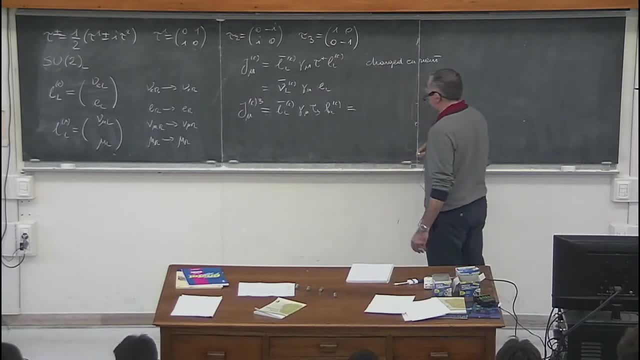 explicitly in terms of the neutrino and electron fields, you find something like nu bar left, gamma mu nu left minus. this minus sign is because of the second entry of tau 3 is negative. e bar left, gamma mu mu e left, and this is a neutral current. 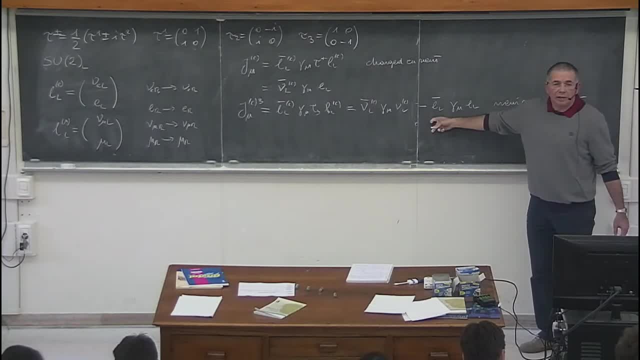 destruction of an electron, creation of an electron, destruction of a neutrino. creation of a neutrino is a diagonal current. it is what we call a neutral current, and it looks like there is no neutral current in the Fermi Lagrangian. so the builder of the 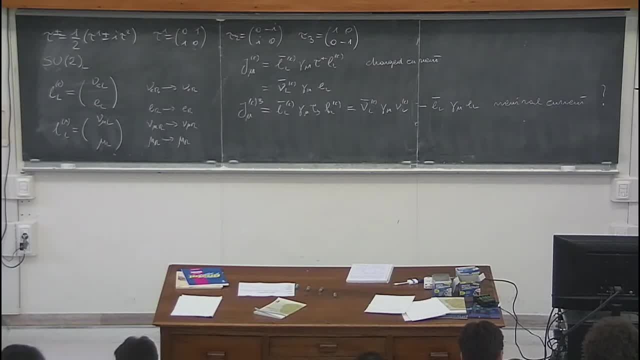 electroweak theory were puzzled by this problem. they succeeded in building a gauge group which gives you the correct charge currents, but it also gives you a neutral current which does not appear to be present in the early phenomenology of weak interactions. of course they already knew that. 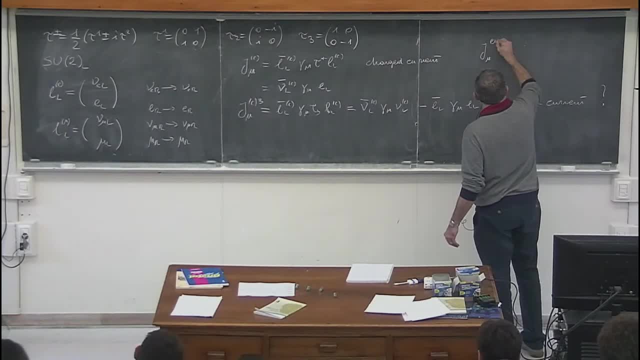 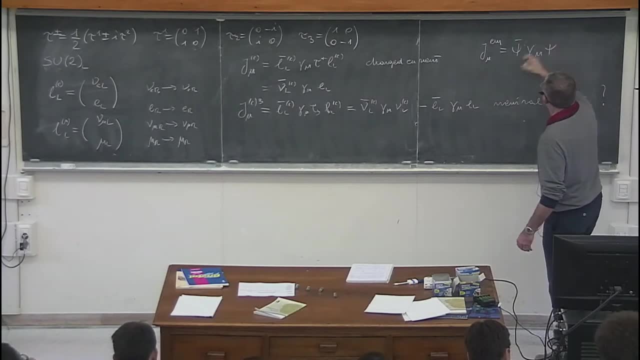 for example, the electromagnetic interactions, the electromagnetic current. it is also a neutral current, something like psi, bar, gamma, mu, the same psi. so this is a neutral current, and it would be nice if the neutral current generated by the SU2 group were precisely the electromagnetic current, but this is not true, as you 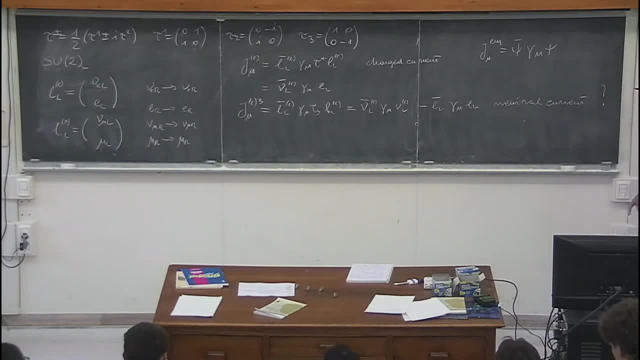 can easily see, there are two important reasons why this J mu3 cannot be identified with the electromagnetic current. the first one is that it only involves left-handed fermions, while QED is parity conserving. the electromagnetic interactions treat on the same footing left-handed and right-handed components. 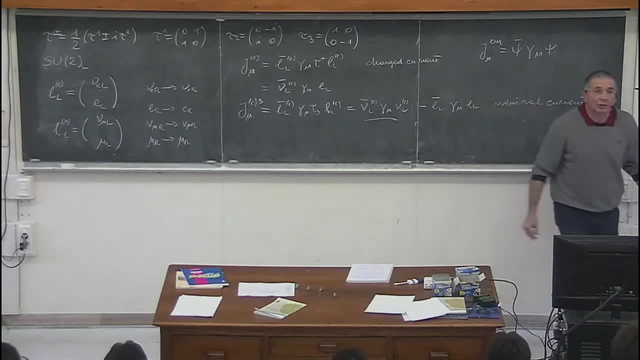 of fermion fields, and also there is a neutrino term, and neutrino terms cannot appear because neutrinos are charge-less. so this is a new thing. this is a new current, a weak current, a genuinely weak current, which doesn't appear to be present in data. 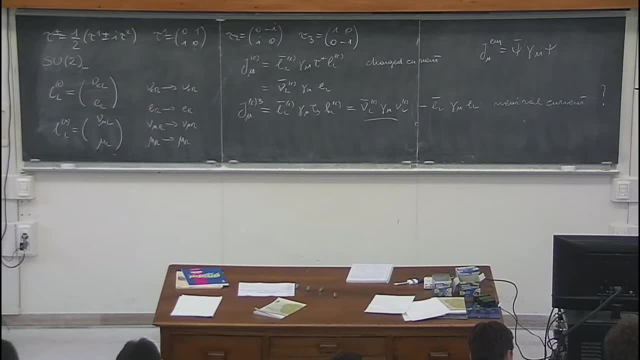 but okay, we hold on, we press on and live with it up to the point at which some evidence of the presence of weak neutral currents will be given to get rid of this unpleasant neutral current- weak neutral current. and you can do it at the price of introducing 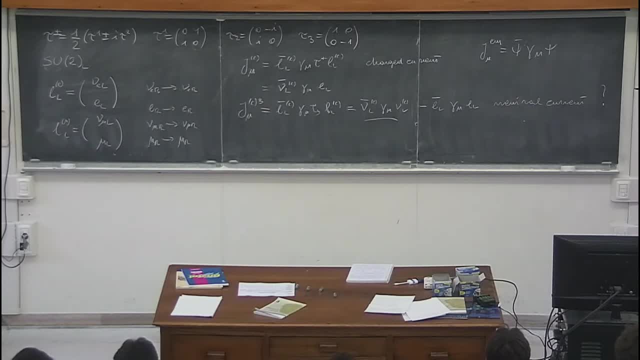 heavy degrees of freedom, which is something we are very used to. but this turned out very soon not to be needed, not to be necessary. so we keep this neutral current among the currents of our theory and go on. what do we do? uh, organizers, should I stop for a while? 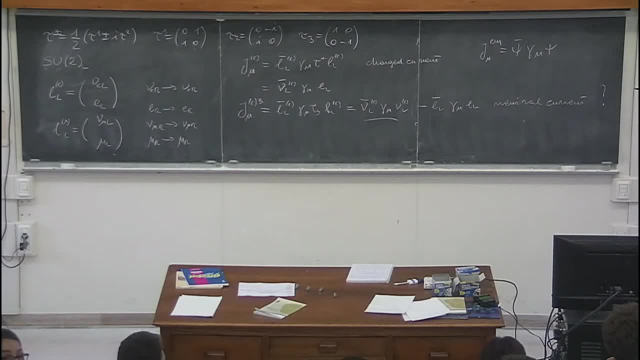 or do I go on? let me look at the faces in order to figure out. I look at careful faces, so I go on. okay, so we have a neutral current around and we will at some point decide what to do with it. so it is at this point. 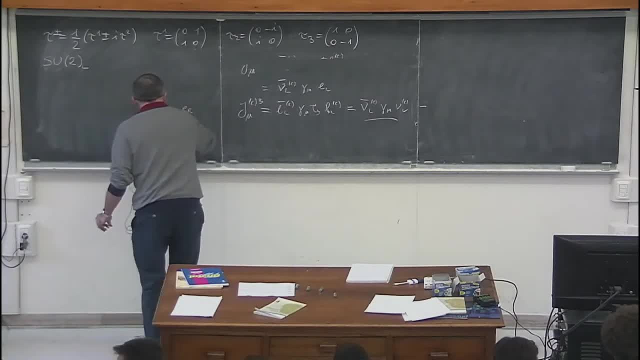 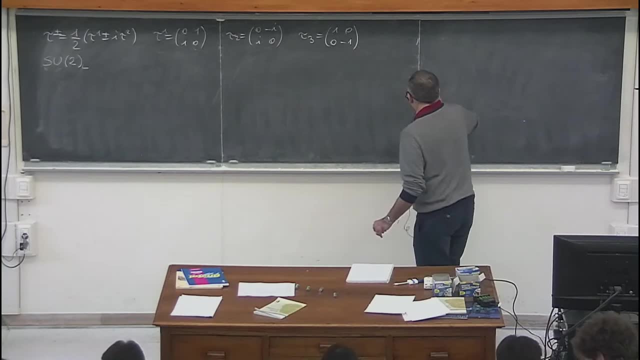 that the electroweak unification comes in because, since we have a neutral current in our system of conserved currents originating from our guest gauge, invariance we are tempted to have a neutral current in our system of conserved currents originating from our guest. 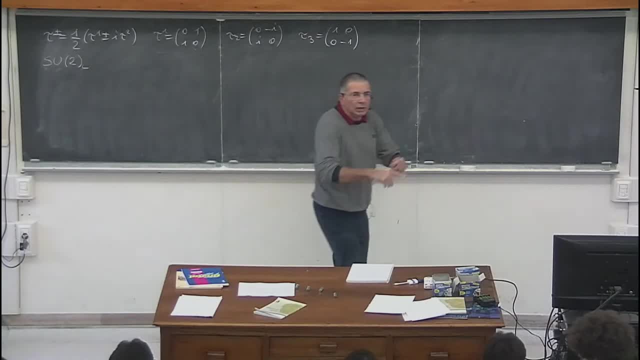 and to enlarge the gauge group in order to include in the system of conserved currents also the electromagnetic currents, which is a neutral current. and how can we do that? well, the easiest way again, which turned out to be the correct way, is to enlarge the gauge group in order to have 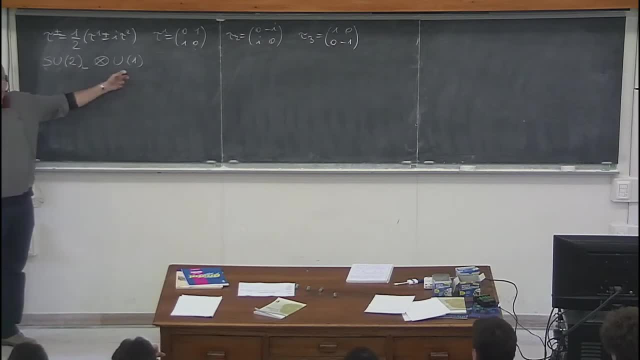 one more generator. so the idea is to take the direct product of SU2 times the abelian factor of U1. U1 is the group of phase transformation and the idea is now we have three generators for the SU2. we have one more generator for U1. 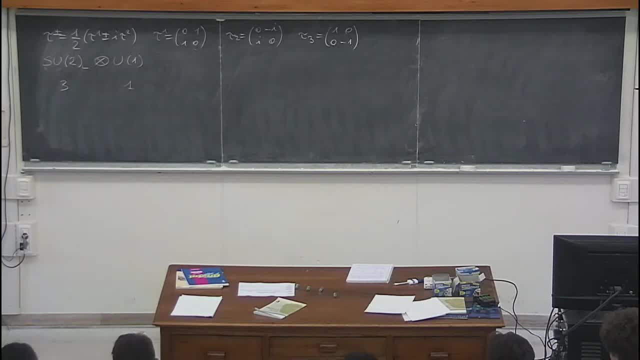 we have now four generators for the gauge group and we can try to see whether we are able to arrange this extra U1 factor of the gauge group in order for the system of currents to include also the electromagnetic current. one would naively assume that this extra factor 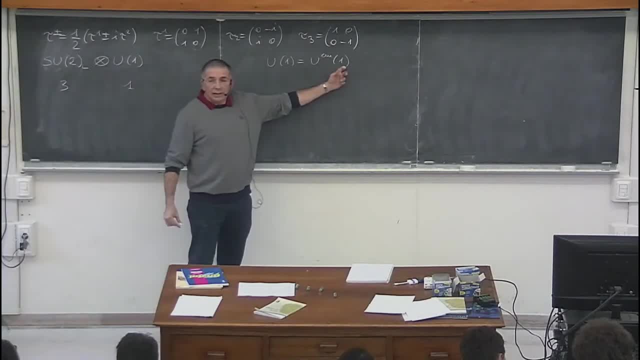 of U1 is just simply the electromagnetic, the gauge group which gives you electromagnetic. but this is impossible. let me put across a bit. you cannot do that, and the reason why you cannot do that is that these two factors of the gauge group must commute with each other. 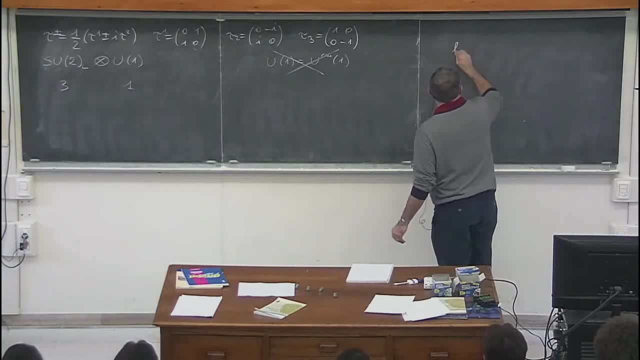 and, for example, the two components of the left handed doublet have different values of the electromagnetic charge. this is neutral and this is charge. so since they are mixed by SU2 transformations, the action of SU2 on that doublet cannot commute with U1 if U1 is the U1. 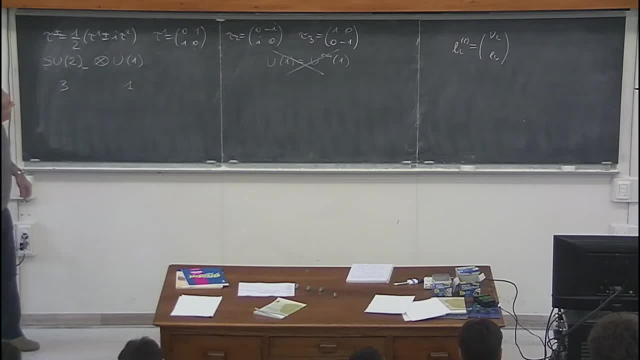 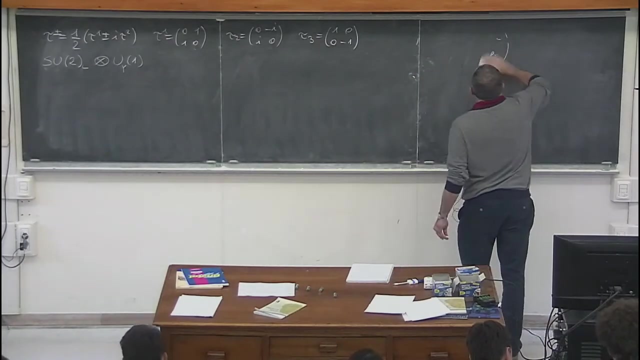 of electromagnetism. so this U1 must be something else, and something else is called weak hypercharge, which is usually denoted by capital Y, and we will see in a moment what this weak hypercharge is. so how do we build a gauge? invariant theory, the recipe. 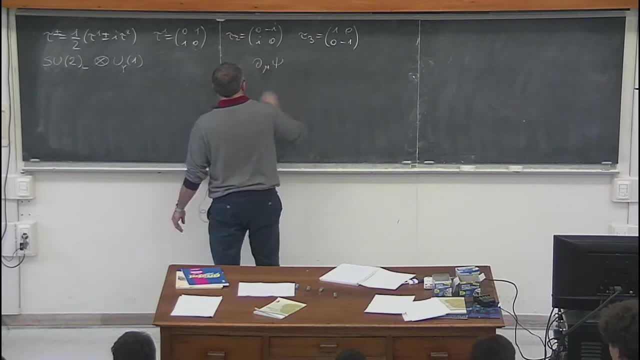 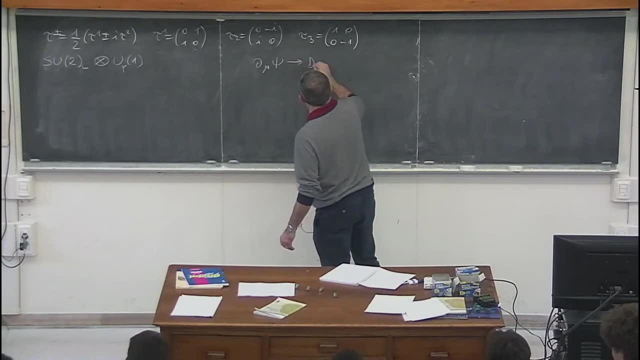 is very well known. you have to replace ordinary derivatives of the fermion fields by covariant derivatives. a covariant derivative is a derivative which transforms in the same way as the field does, and the way to define the covariant derivative is like: this is the ordinary. 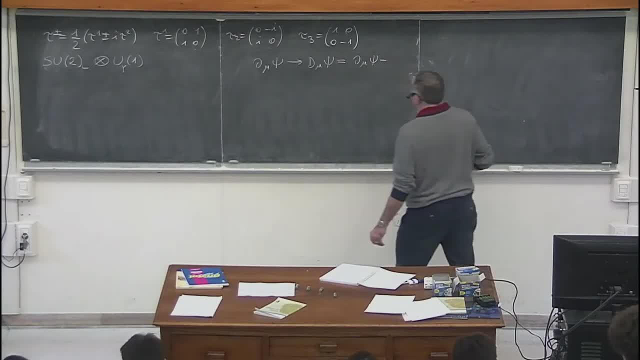 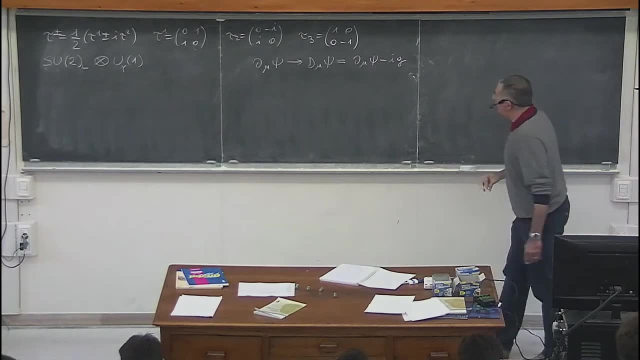 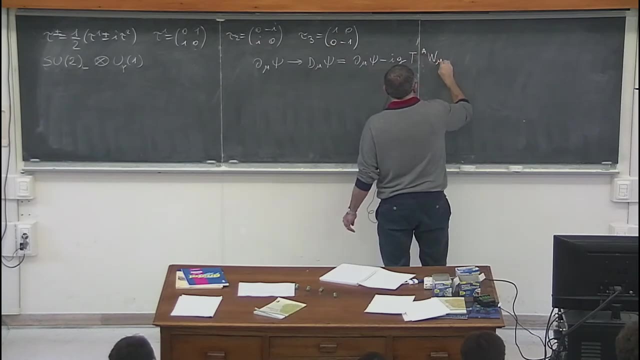 derivative of the fermion fields. here there are some conventions. minus sign, which is conventional i. the present of this coupling constant G is also a matter of conventions. let me call TA the three generators of SU2 which are relevant for the representation of fermion psi. 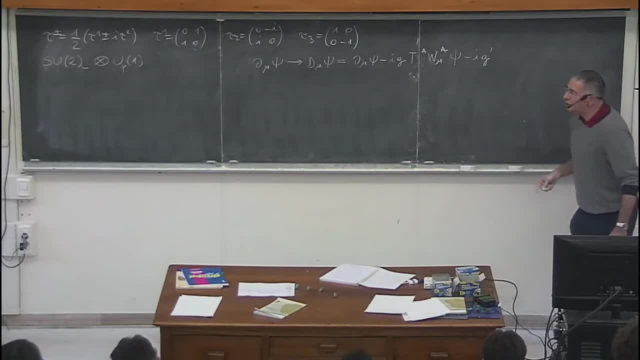 then you have an extra connection term related to the U1 factor of the gauge group. let me call G, prime, the relevant coupling constant. I will call B, mu, the vector boson, which is related to U1. and then here I have to put a hypercharge quantum number. 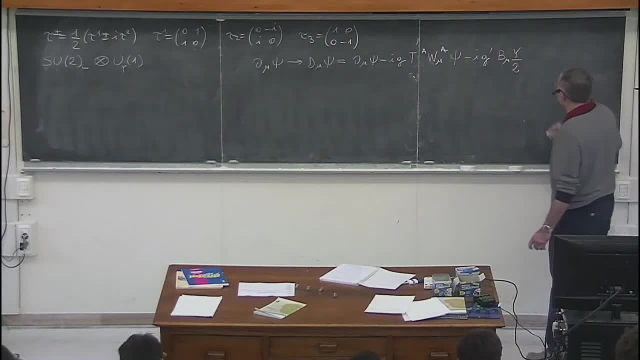 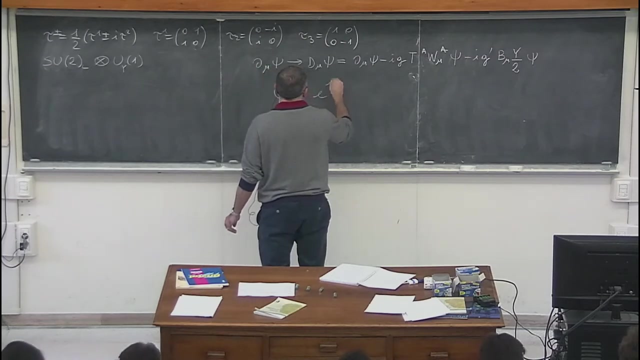 which is customarily written like this: times psi, and this is a covariant derivative, under the assumption that the transformation property of the first fermion field, psi, is e to i, G, TA, alpha a of x, exponential of i G, prime y divided by 2 times beta of x. 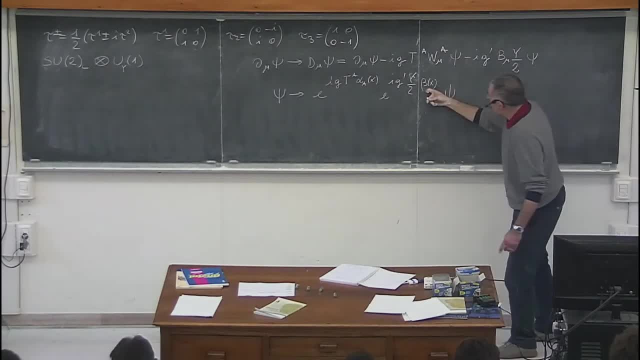 times pi, where beta of x, alpha 1, alpha 2, alpha 3 are three real functions of the space-time coordinates at which we take the field psi. if you take this definition of the action of the group on the generic fermion field, psi. 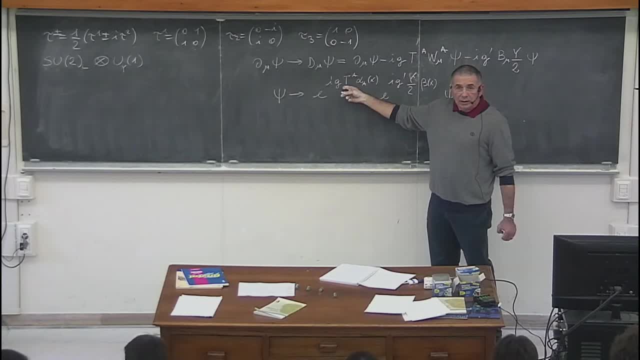 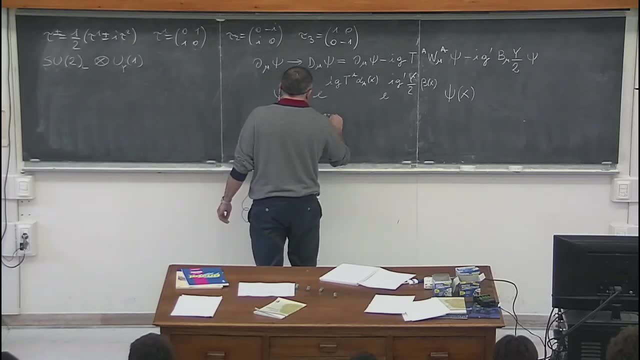 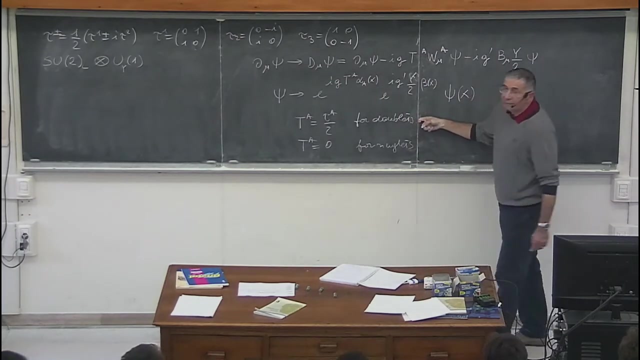 here, of course, you have to choose the correct generators of the gauge group. for example, TA is equal to the three Pauli matrices divided by 2 for doublets and TA equal to zero for singlets. left-handed. yes, you can do it, it's they, but they do commute. 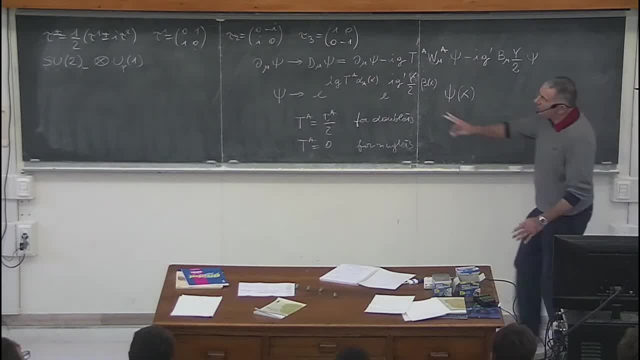 by assumption, they act on different indices. on the right-hand side they do commute, and this is precisely the reason why this y cannot be identified with the electron charge the way you see that they. well, y is proportional to the identity matrix in the representation of TA. okay, so this is. 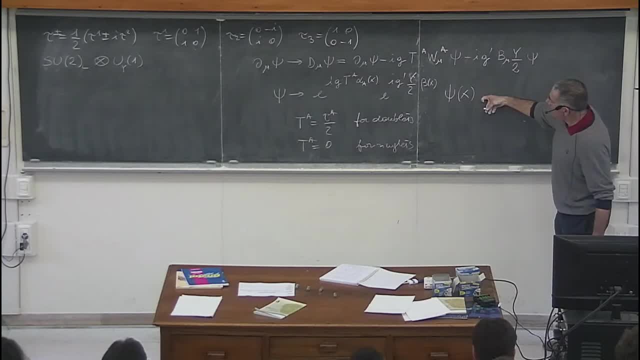 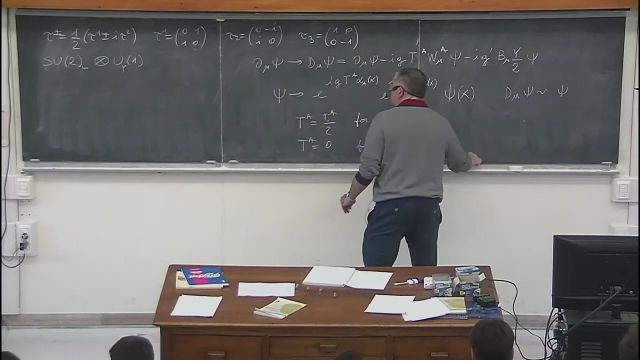 the precise definition of the gauge transformation for a generic field in a generic representation of the gauge group. and this is the covariant derivative, in the sense that d, mu, psi transforms in the same way as psi transforms. so Lagrangian density is now easy to write down. 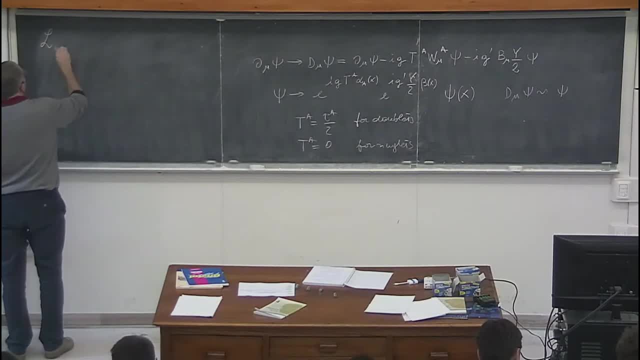 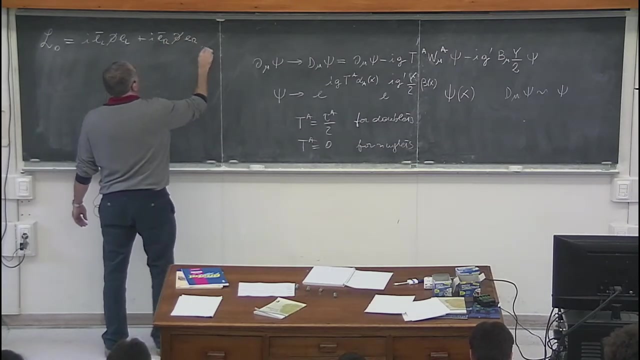 you start by writing down the Lagrangian density for the free propagation of the fermions we are talking about. so it is: i l bar left d slash l bar plus i e bar right d slash e right plus i nu bar right d slash nu right. 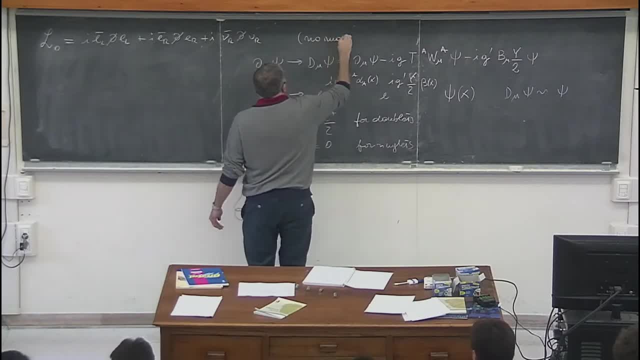 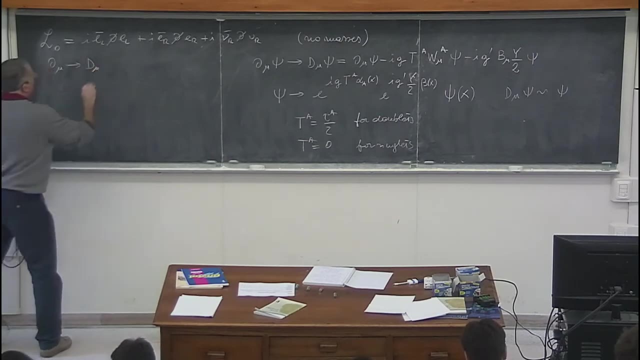 no masses for the moment. we will talk about fermion masses in later lectures. and then you replace all ordinary derivatives by covariant derivatives according to the different representations of the gauge group. so what you end up is an interacting Lagrangian. this is a free Lagrangian, it only 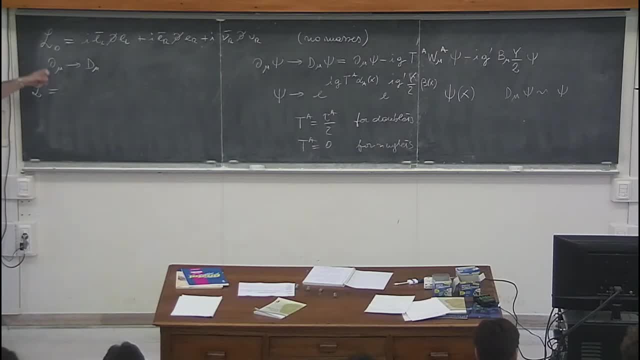 contains quadratic terms in the fields. but if you replace the covariant, the ordinary derivative, by the covariant derivative, i get interaction terms and the interacting Lagrangian is the free Lagrangian plus something, and i split the interaction terms into two pieces. the one is: 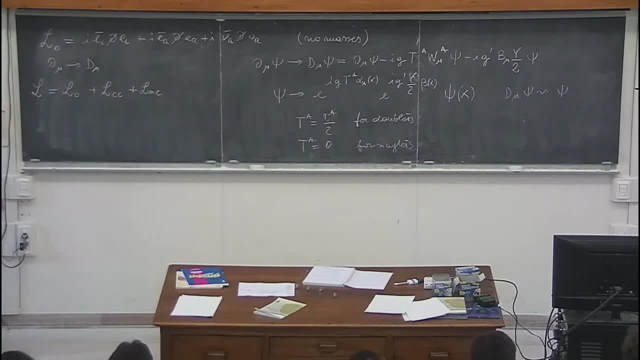 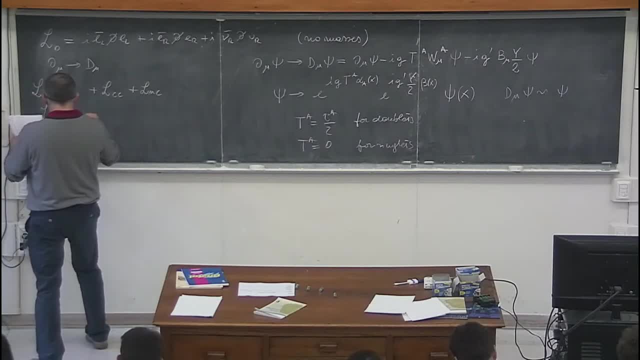 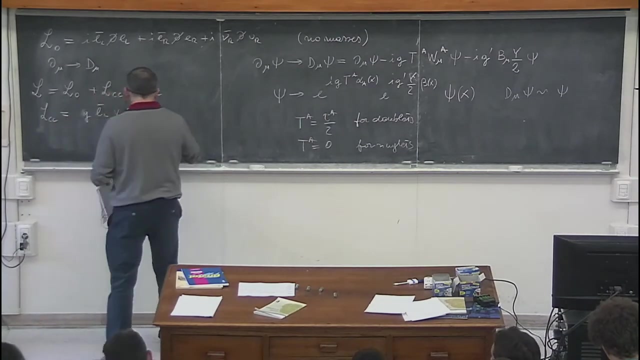 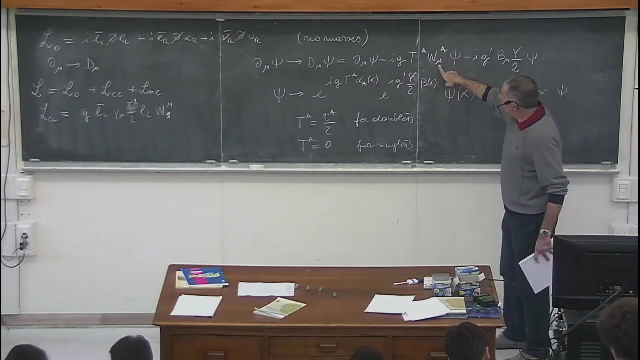 so this is simply given by g, g, l bar left, gamma mu, tau plus l left times. well, actually, ok, yeah, write it like this: tau one over two times w mu one, where w mu one is one of the three real factor fields related to the SU2 factor. 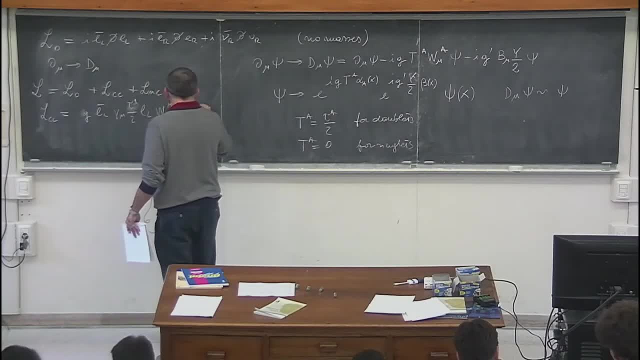 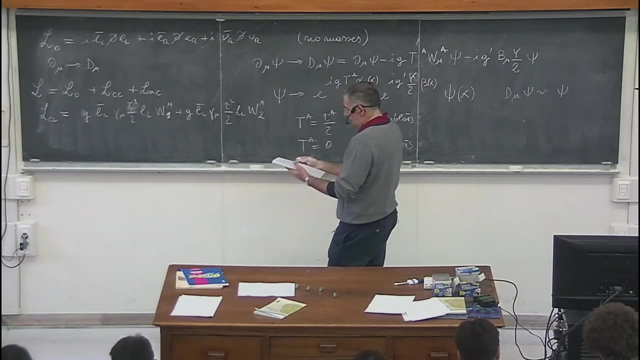 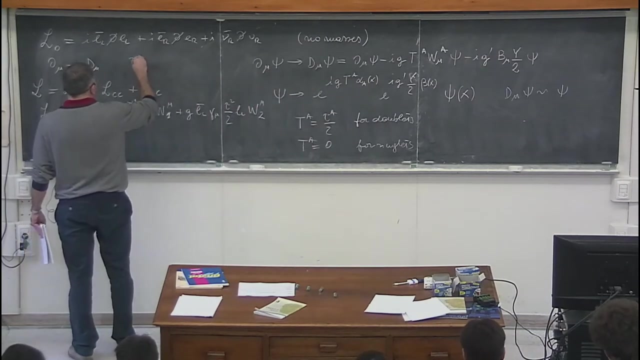 of the gauge group plus g, l bar left gamma mu tau two, divided by two: l left w mu two. and if you want to go back to our previous notation of tau plus and tau minus, you have tau one equal to tau plus plus, tau minus and tau two equal to. 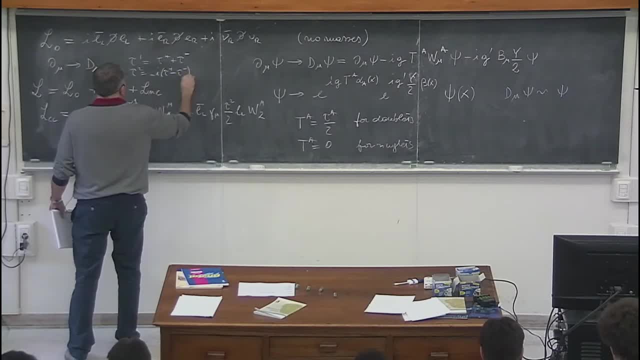 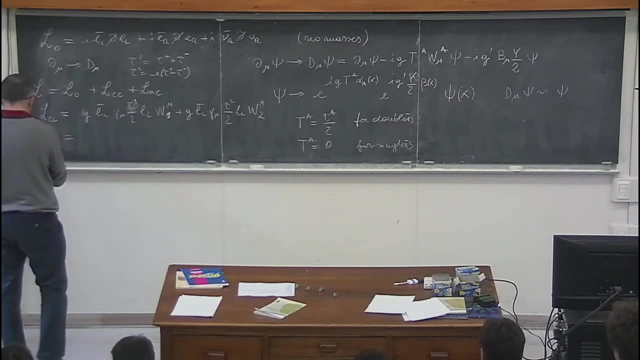 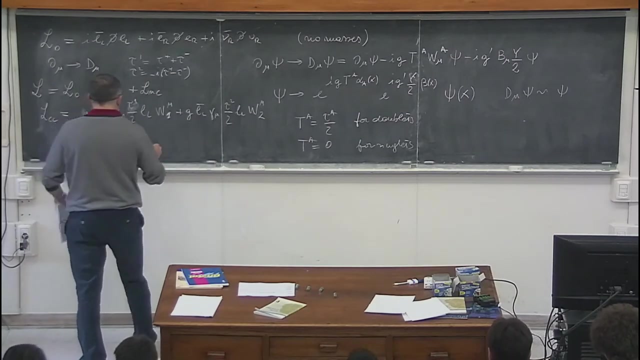 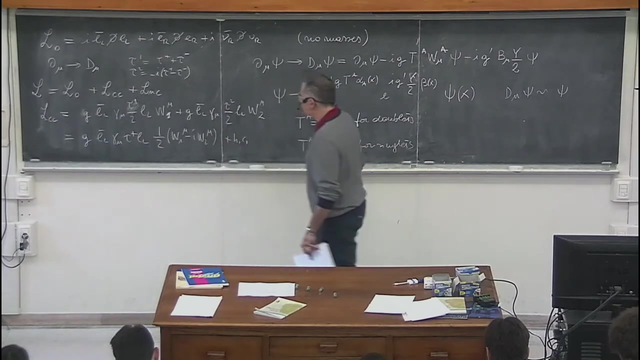 minus i tau plus minus tau minus. so this is equal to g l bar left gamma mu tau plus l left gamma mu times one half w one mu minus i w two mu plus the Hermitian conjugate, and what is usually done is to write this as: 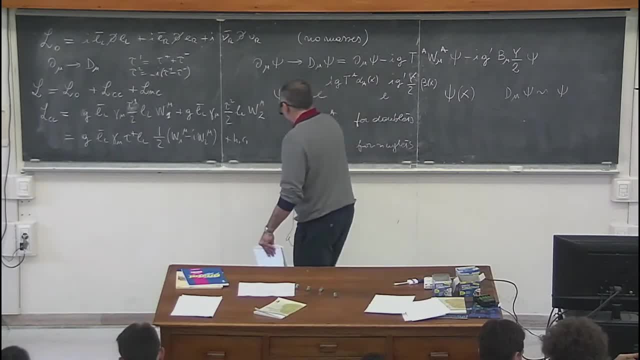 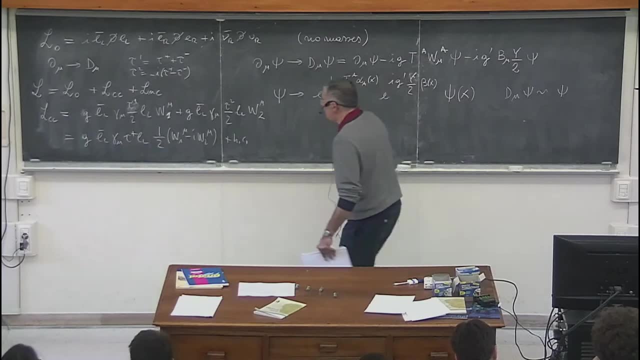 as as as g over root of two, g over root of two. l bar left: gamma: mu tau plus l left. w mu plus plus the Hermitian conjugate, where I have defined w mu plus minus equal to one over W mu 1 minus plus I. 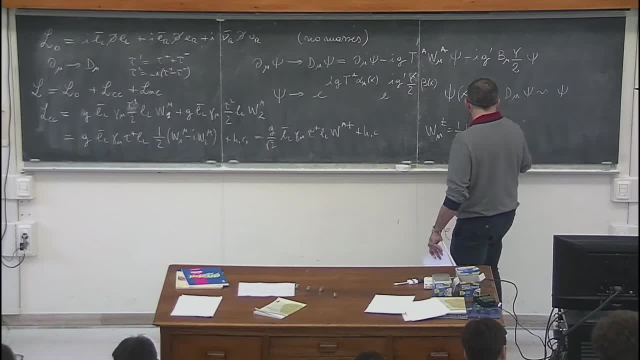 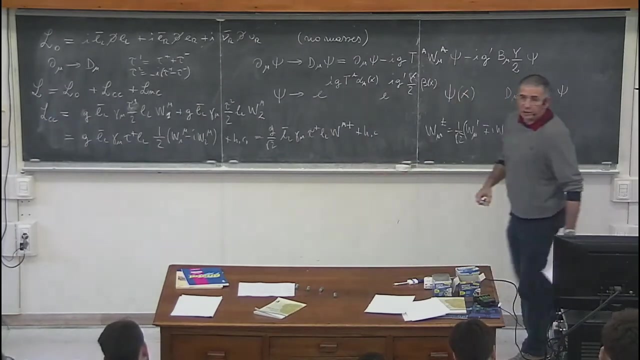 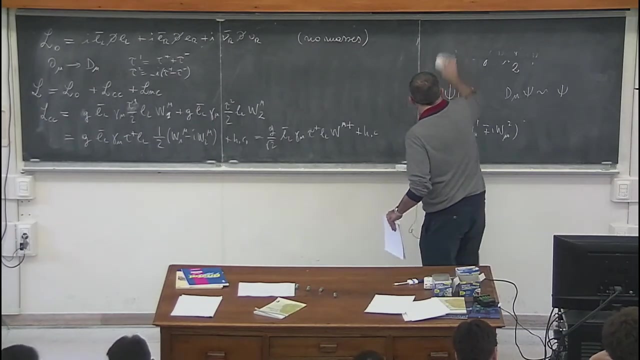 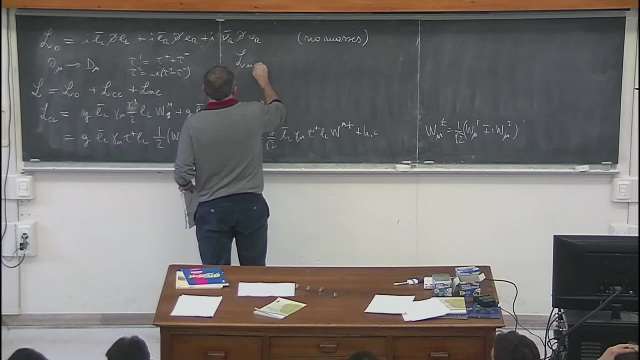 W mu 2.. These two complex combinations of W1 and W2 are two electrically charged vector bosons which are coupled to charge currents. These are the charge current interaction terms. The neutral current has two terms: One which comes from the diagonal generator of SU2, tau3. 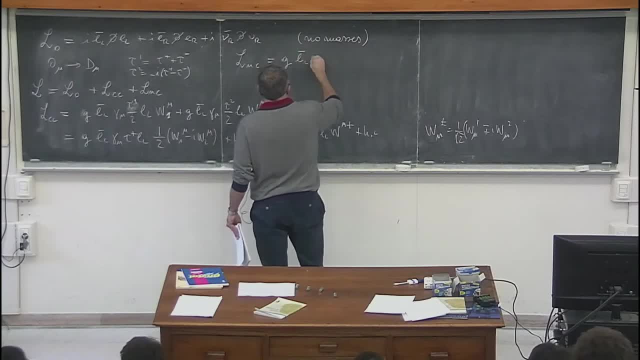 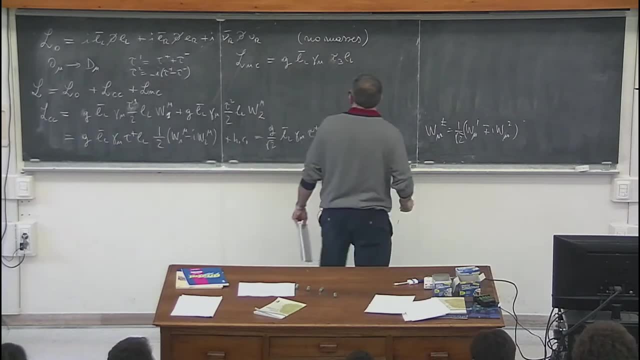 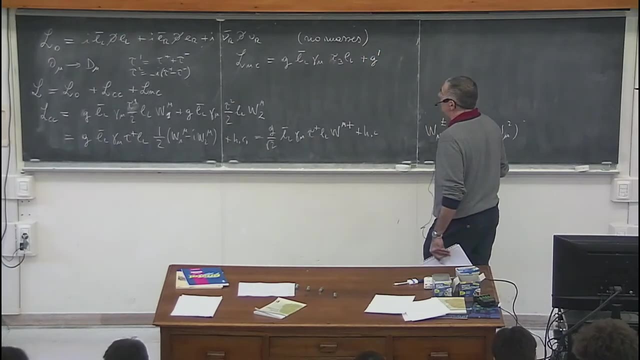 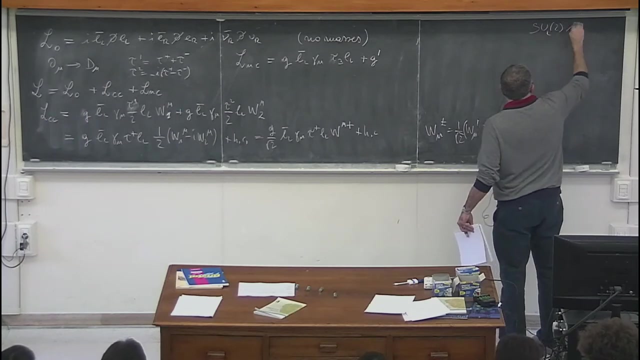 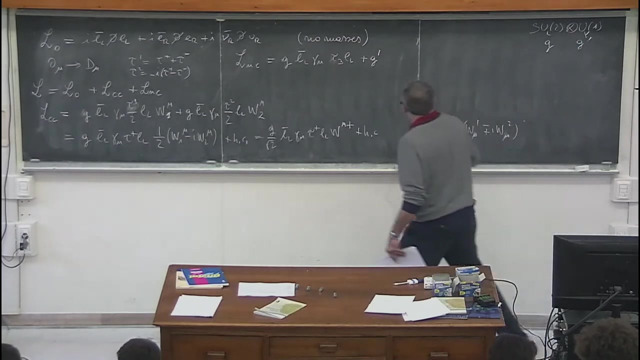 So it is G, L bar left, gamma, mu, tau3, L left, And the other one comes from the hypercharge term, which is plus G prime. I'm calling G prime the coupling constant related to factor of U1.. I have a hypercharge quantum number. 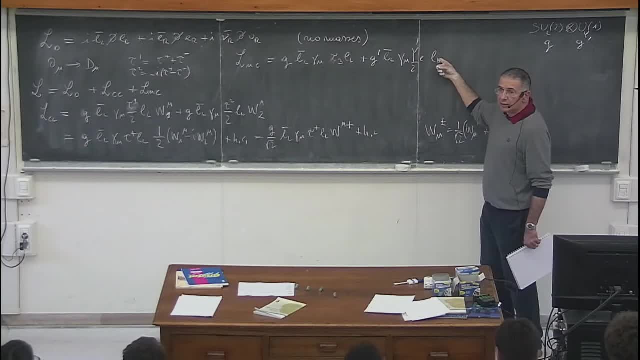 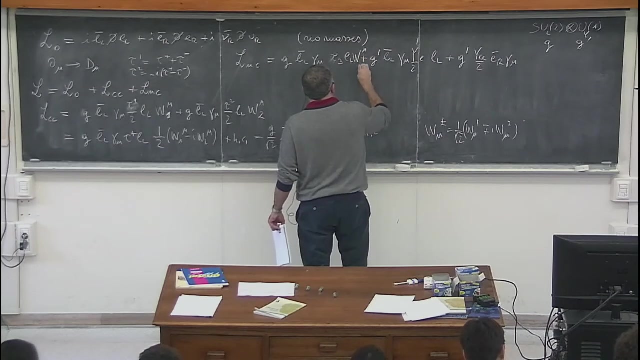 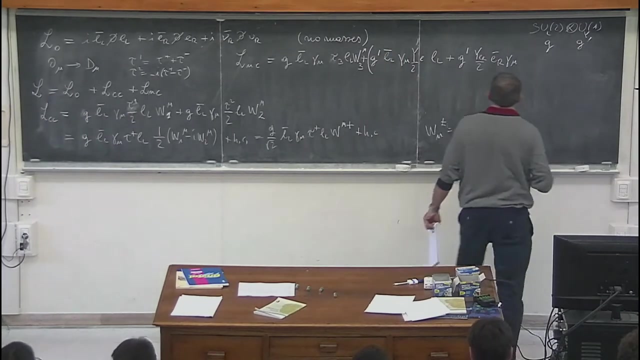 for both the left-handed neutrino and the left-handed electron. But then here I have to add terms for the right-handed electron. I'm sorry, I forgot to put here the vector boson W mu 3.. And all these terms I'm writing down here. 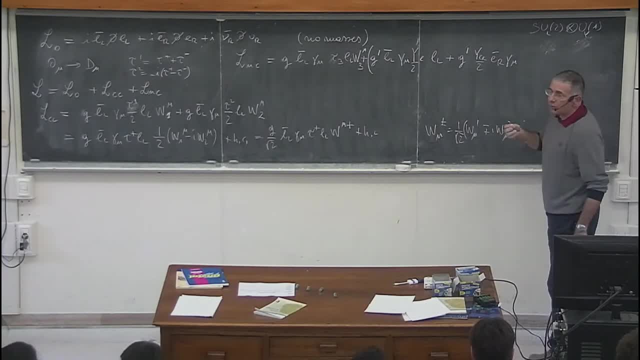 are coupled to B mu, which is the vector boson related to U1.. And the shear current number is written down here just in essentially sine 1.. And there This is the neutral current interaction term. This is rather difficult to interpret. 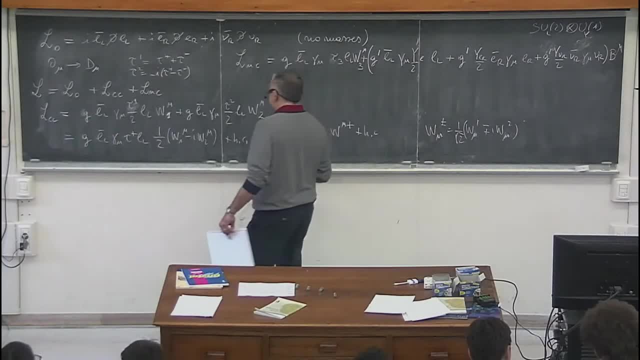 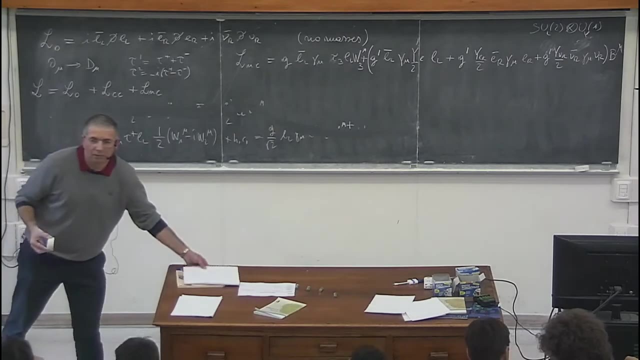 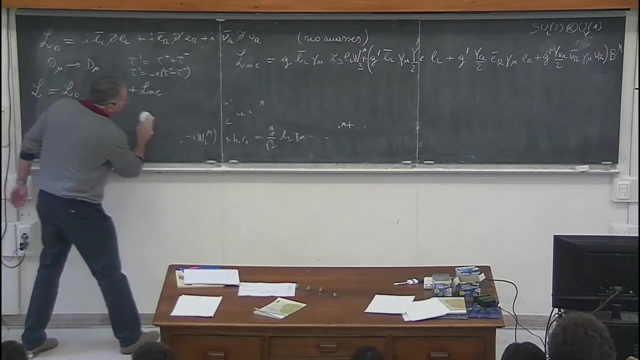 It becomes easier if you simpl finalmente a little bit. yes, I don't think so. yes, I actually don't know why there is this root of 2 in the original Fermi constant. I don't think it's related to this, because the relation between G and G Fermi 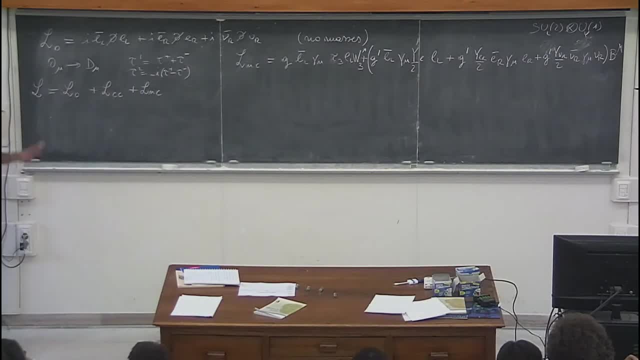 is quadratic, so we will see in a moment. so I was talking about the possibility of simplifying the looking of the look of this neutral current term and the idea is the following: let me collect all four Fermian fields: neutrino- left-handed, electron- left-handed. 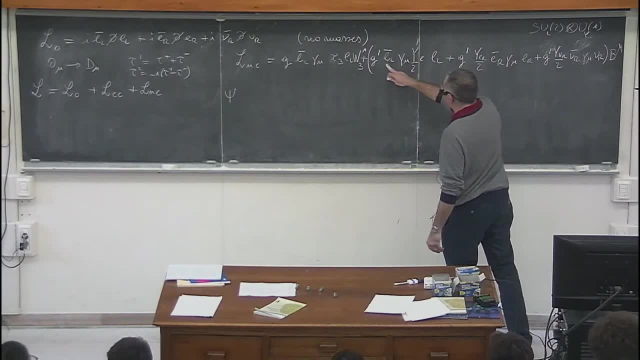 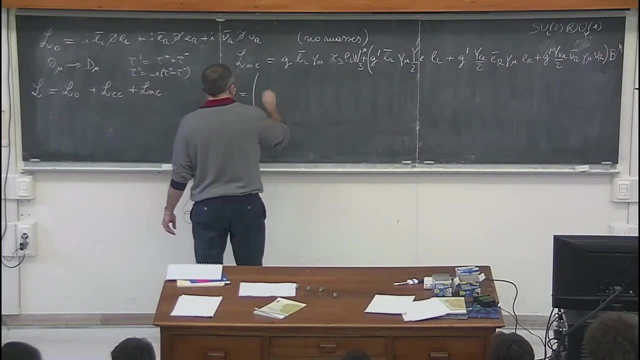 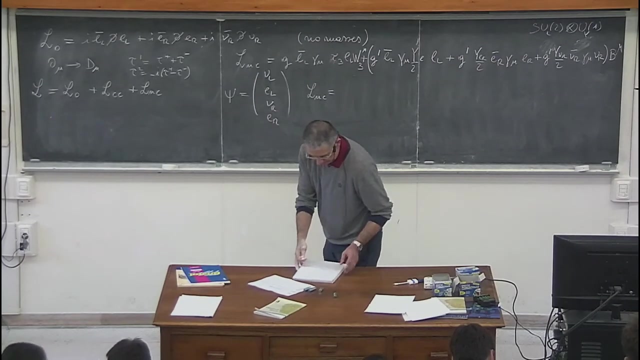 electron right-handed, neutrino right-handed into a single object and then, if I do that, I can write the neutral current interaction term as- let me copy it from here so I don't make mistakes- psi bar. where this psi is, this four component, is a a neutral current interaction term. 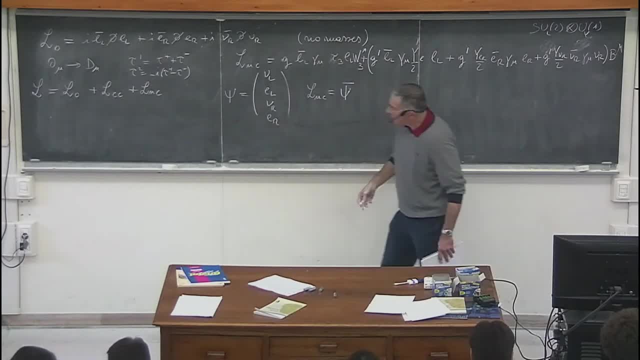 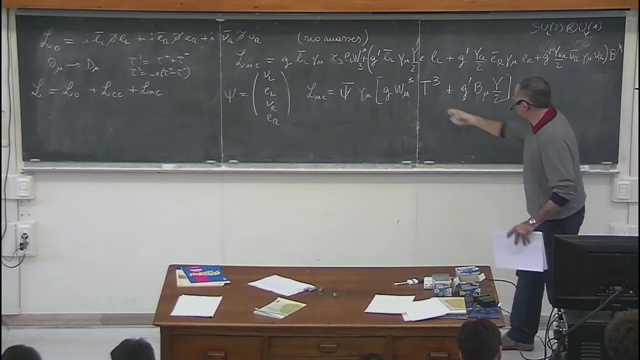 an object which is obtained by putting in the same colon four different, four components: Dirac fields, psi, bar, gamma, mu, g, w, mu, three times t, three plus g, prime, b, mu, y, divided by t, three, by two psi, and this two objects, T3 and y. 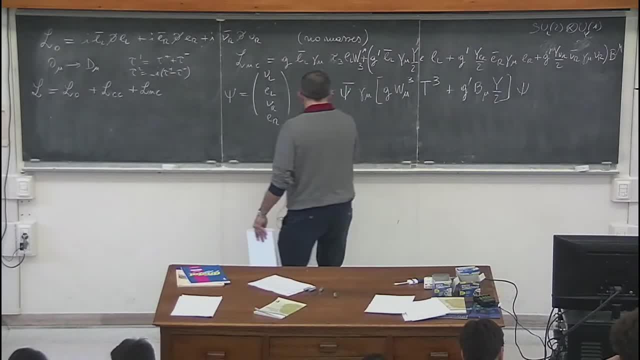 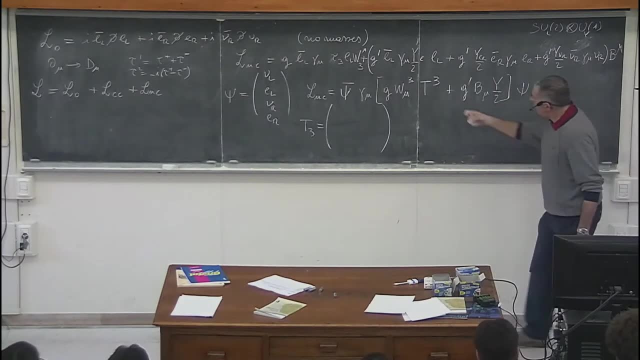 divided by two are their 4 by 4 matrices. they are diagonal matrices which carry in the main diagonal the relevant values for Themeesy, T3 and B? U corresponding to the different fields. for example, T3 is 1 half minus half for the doublet. and 00 for the two singlets and y is 0 for the two singlets and y is 2алdb in commas and y ви-adv 다 l continié Pinkes and yi otkar agradecki. we need to know that. uhm also, can you kid a lot about T3 by F streaks and yi last e Kurla 들어까지 a twenty buy翻atoon to put on the labels. at that level, For example, T3 is one half minus one half for the doublet and 0, zero for the two singlets. 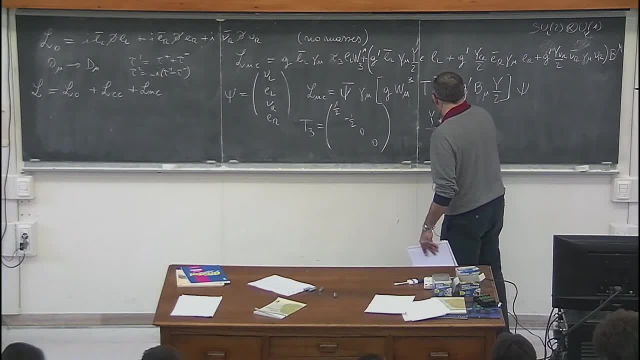 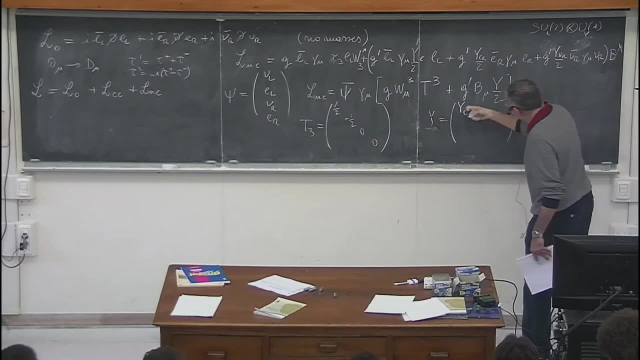 is a 4x4 matrix with the four values of the hypercharged quantum number, actually three values, because the two components of the left-handed doublet have the same hypercharged quantum number. then I have Y nu R and Y e R- Excellent. 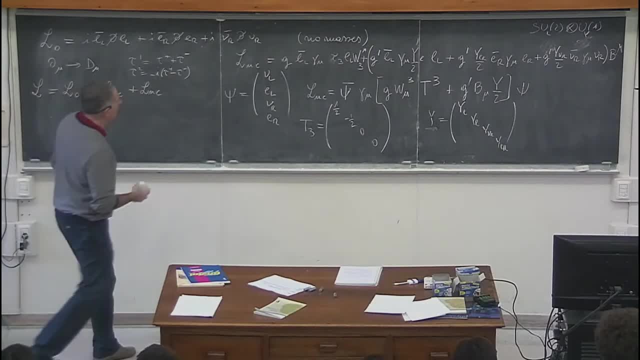 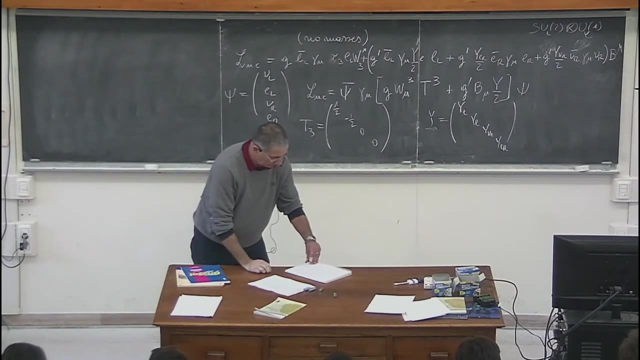 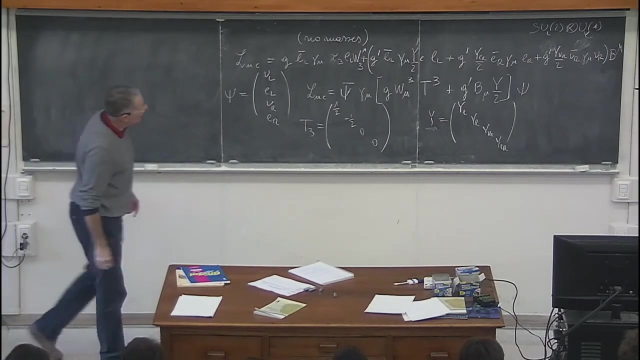 So in this way the neutral current term is easy, And we have already seen that neither the current which is coupled to W mu3, nor the current which is coupled to B mu can be identified with the electromagnetic current. So the idea here, which was originally suggested by Glashow, 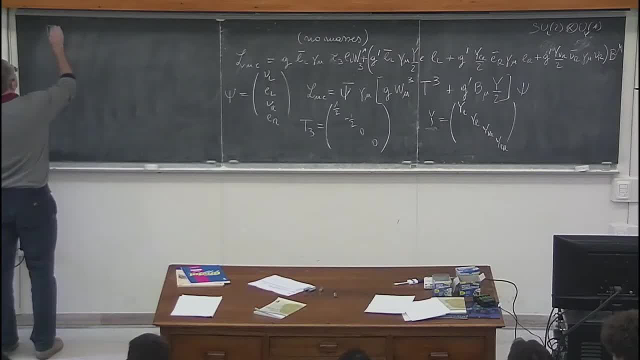 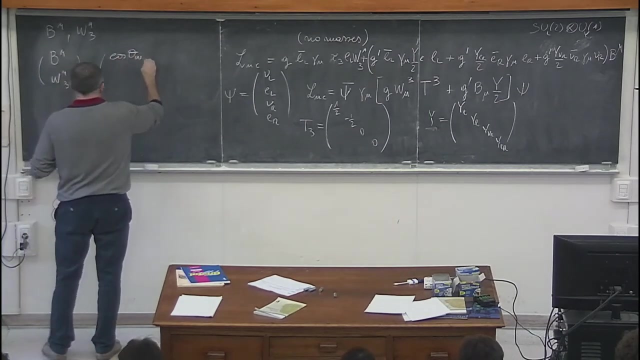 actually is to replace B mu and W mu3 by two linear combinations of them, And the linear combination was defined originally to be the following money game: the free, american free- and balance. So by shortening the value of Y nu under the currency. 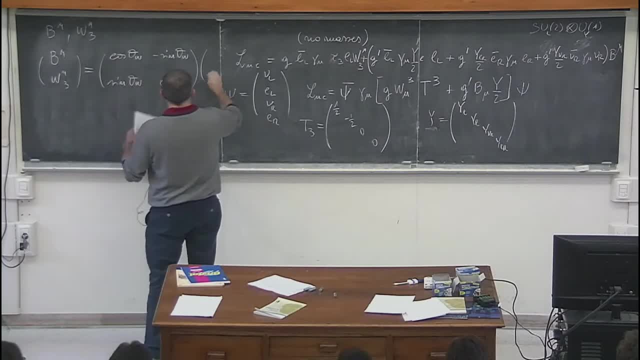 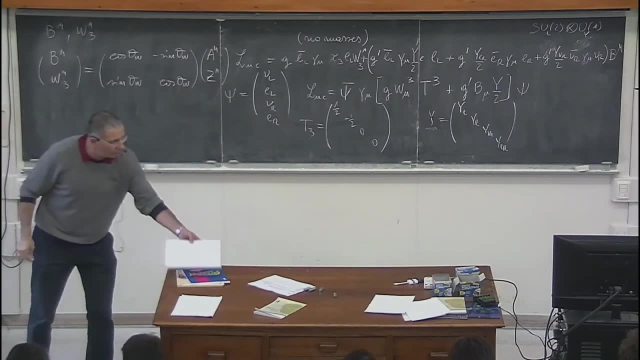 you can see that it is also a little higher. Since at this point the signal was too low, it could not be Well影片 and it for that I have lapped W. new vector fields, neutral real vector fields A-mu and Z-mu, and I define them to be linear combinations. 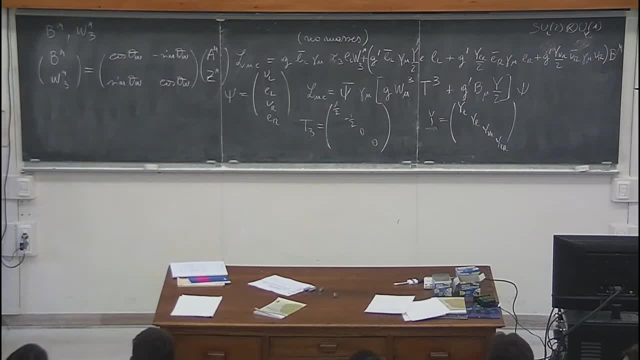 of B-mu and W-mu3.. This is an orthogonal transformation. The reason why we better choose an orthogonal transformation will be clear in a moment. In principle, one could even take a generic mixing matrix among the two, but it is convenient to take. 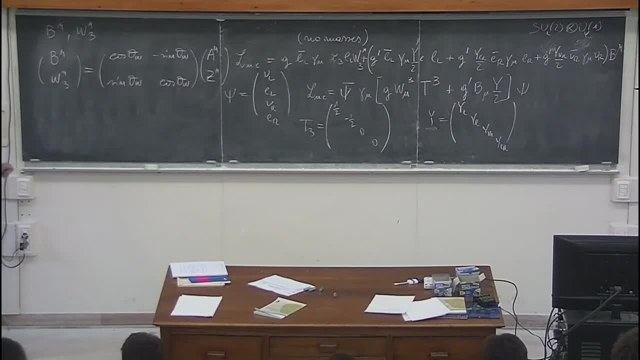 an orthogonal transformation. I just replace B-mu and W-mu3 by these two linear combinations of A-mu and Z-mu, and A-mu and Z-mu are defined by this relation here, And theta-w is a new parameter which will have to be fixed. 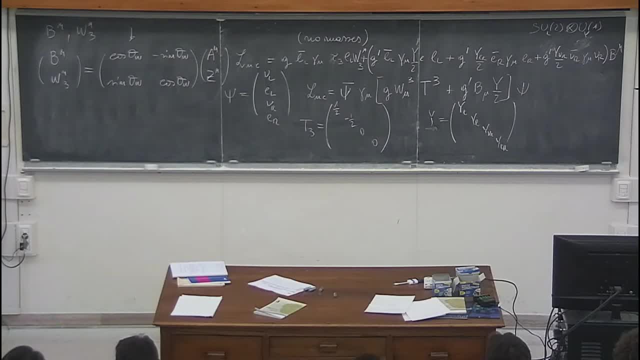 on the basis of phenomenology, at some point It's an angle, It's called a weak angle. It's sometimes called a Y, But this is actually. it was introduced by Glashow, so he was unfortunate in choosing the initial of weak. 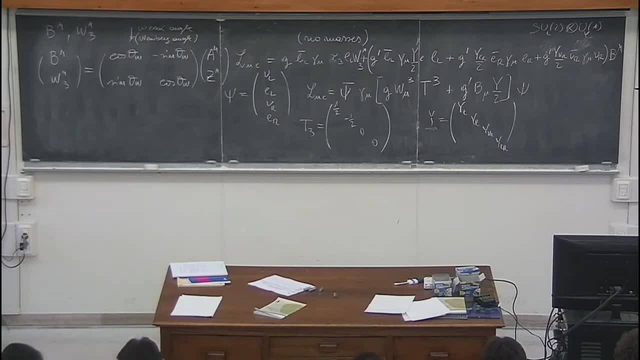 which was also the initial of Weimberg. Anyway, I do that, And if I do that it's very easy. I just replace W-mu3 and B-mu by the expressions which correspond to this rotation here, And what I get is psi-bar gamma-mu. 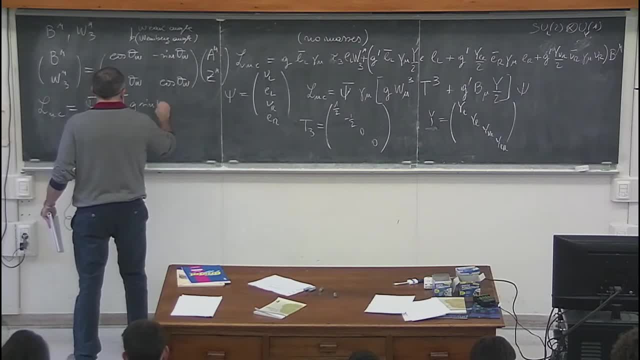 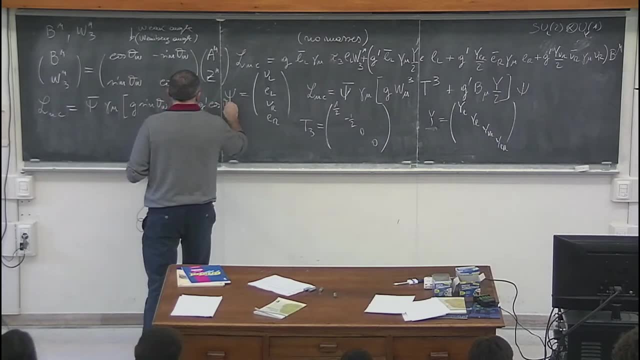 G sine theta-w, T3 plus G prime cosine theta-w. I just, or I get the integral. So I simply keep this one on And I just, and I keep going. And here we have a new problem, And that is the function of the vector boson. 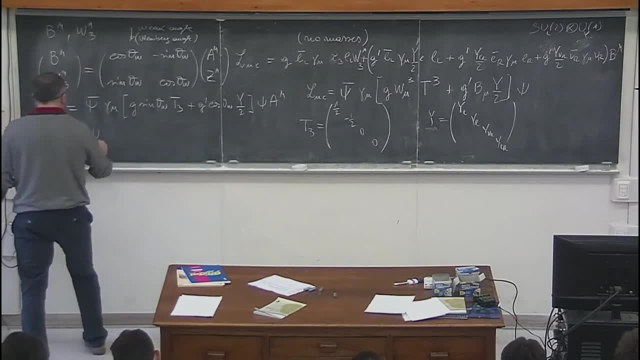 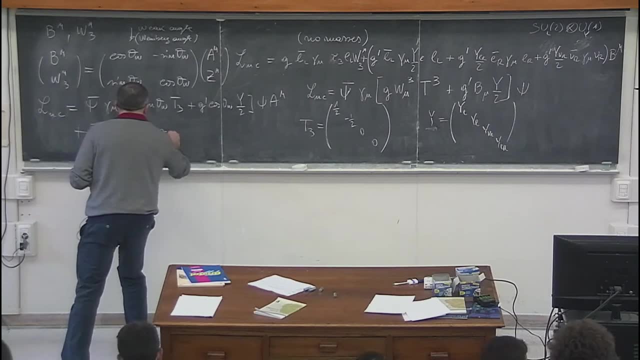 you can expect to keep it, which we're going to talk about in the next lecture, And that is that when you start the equation with Z-mu, you end up with a God-like wave, and I'm going to show you how to do that. 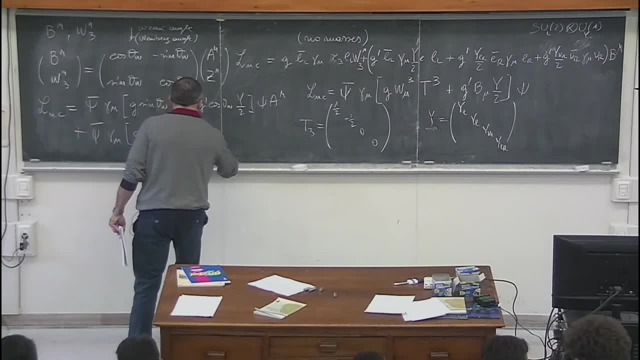 So in the example data. so you have to write down what you're going to call sine theta w the matrix of hypercharged quantum numbers, psi, z, mu. I did nothing actually, I just reparameterized the theory by this choice of linear combinations. 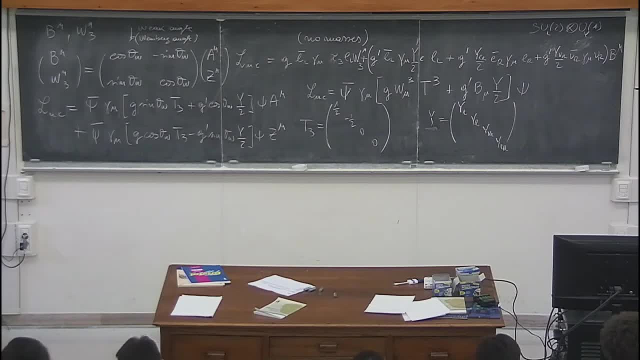 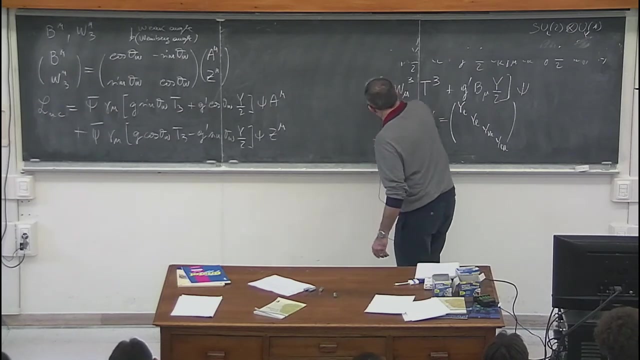 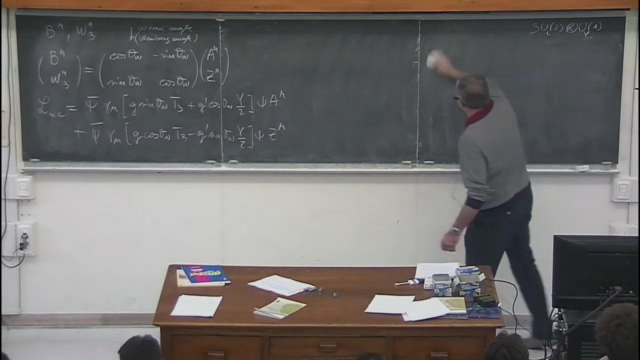 of the two neutral current vector bosons. I end up with this expression for the two neutral current interaction terms. I would like to keep. Well, You have them in your notes and I have them in my notes, And what I now want to do is to try to see whether I can identify. 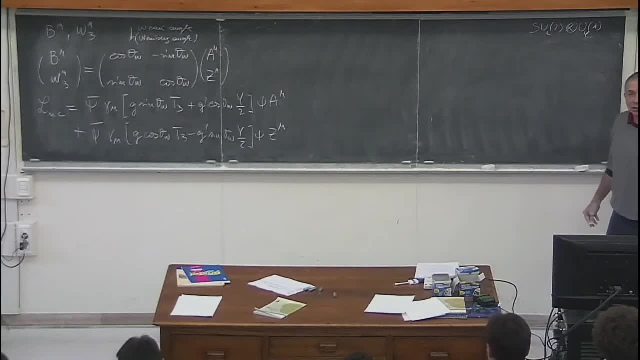 one of these two terms with the electromagnetic interaction term, which I know is mediated by a neutral current. I choose this one because I call it- And if I want this to be a mu times- the electromagnetic current. the electromagnetic current is the proton charge. 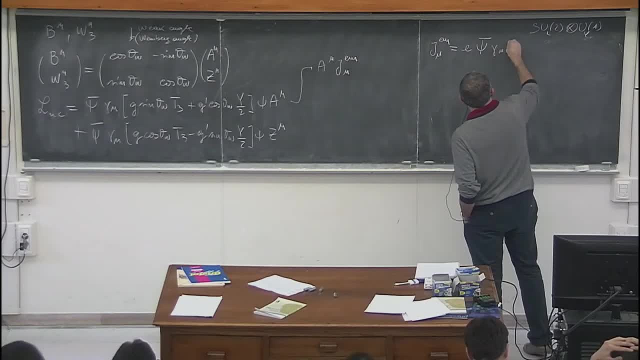 times psi, gamma, mu, q, psi, where q is a diagonal 4x4 matrix which contains in the main diagonal the values of the electric charges of the different particles in units of the proton charge. So it is 0, minus 1, 0, minus 1.. 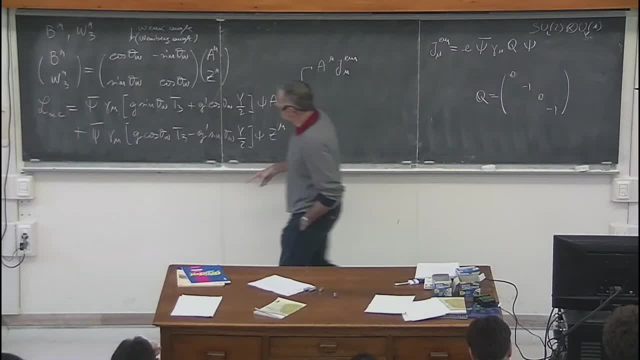 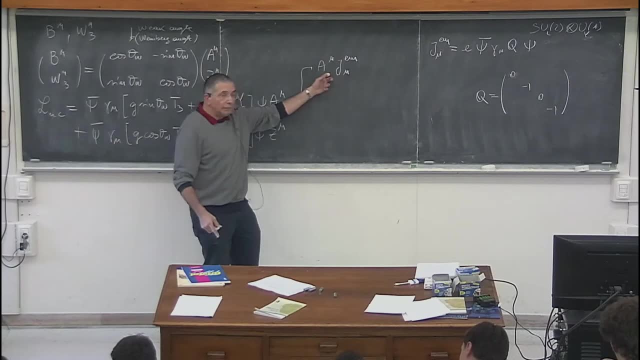 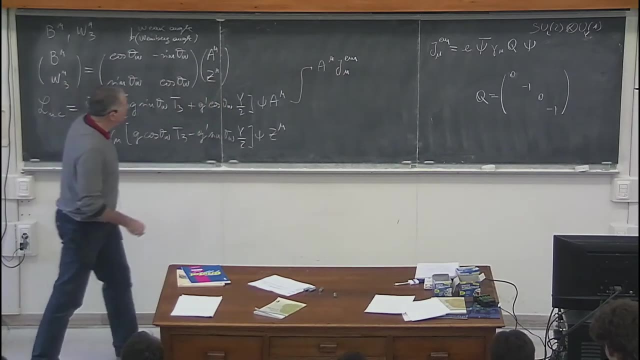 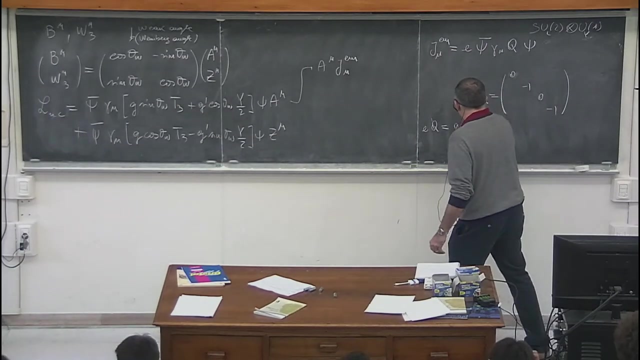 So this is true. This first weak interaction term can be identified with the electromagnetic interaction term and therefore the field which I call a mu can be identified with the photon field, provided q e times q is equal to g sine theta 3,. 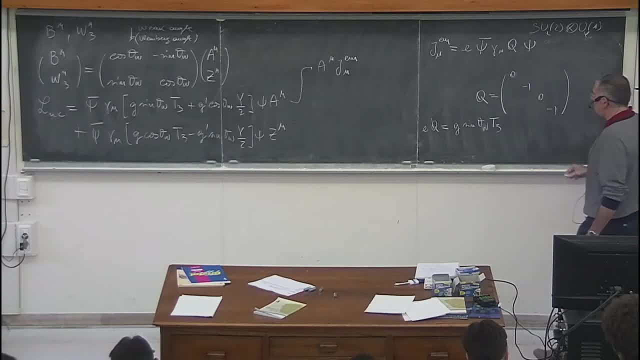 theta w- sorry t3, plus g prime cosine, theta w, y divided by 2.. So the question is if there exists a choice of g, g prime and theta w such that this identity holds true, And of course there is. 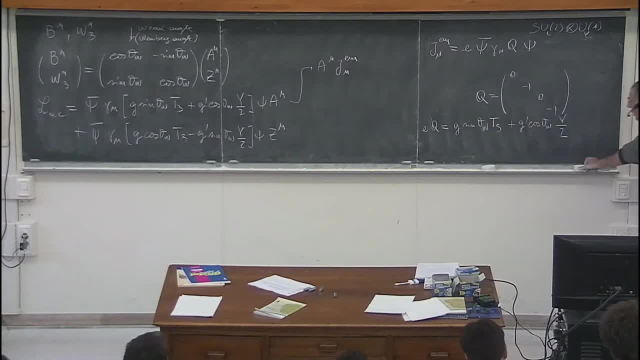 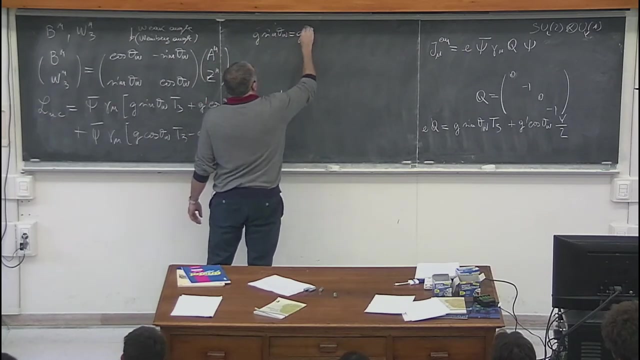 I have many parameters around I can play with, so I can force this identity. The easy way to do it is to define g and g prime in such a way that g sine theta w and g prime cosine theta w is equal to the proton charge. 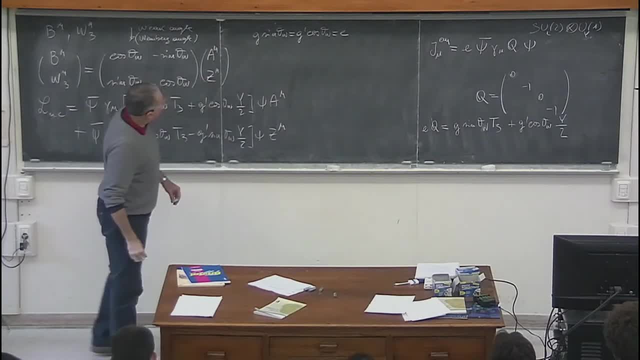 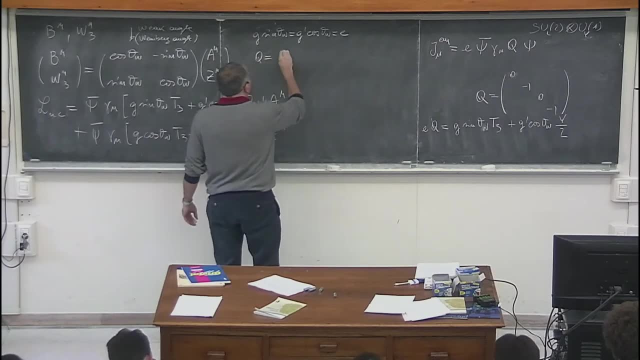 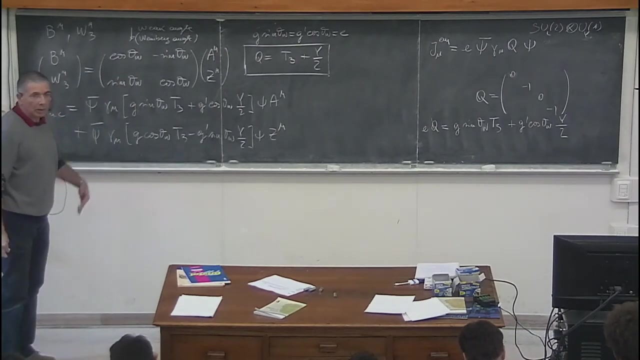 If I choose parameters in this way, then that identity becomes simply q equal t3 plus y divided by 2.. And this deserves a frame. It's a very interesting relation. It will apply in different cases. What does it mean? For example, it means that 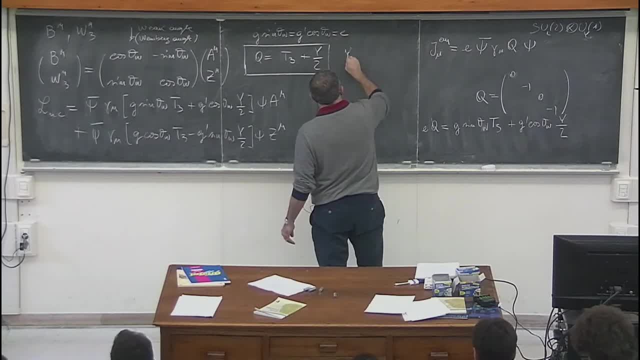 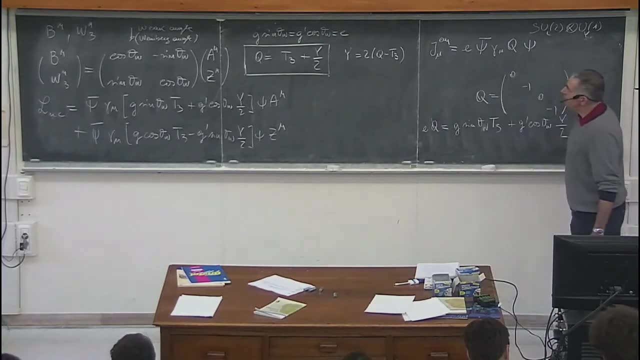 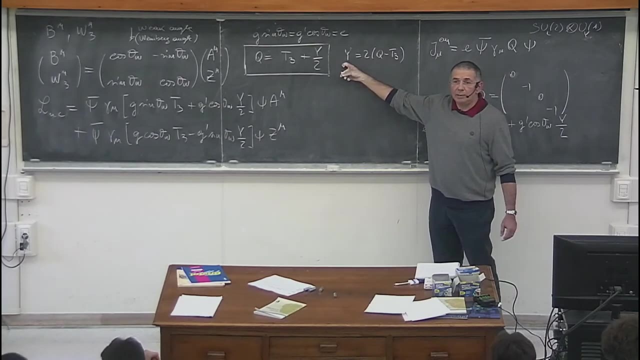 you can solve it for the hypercharge matrix, And from this relation here you can determine which choice of hypercharge quantum numbers you have to make in order for one of the two weak, neutral current terms can be identified with the electromagnetic interaction terms. This means, for example: 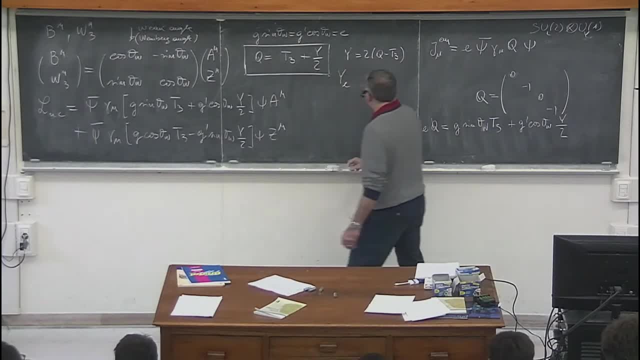 that the hypercharge of the left-handed doublet is equal to two times. For example, if I take the first component, q is equal to zero, which is the charge of the neutrino, and t3, is equal to one-half. 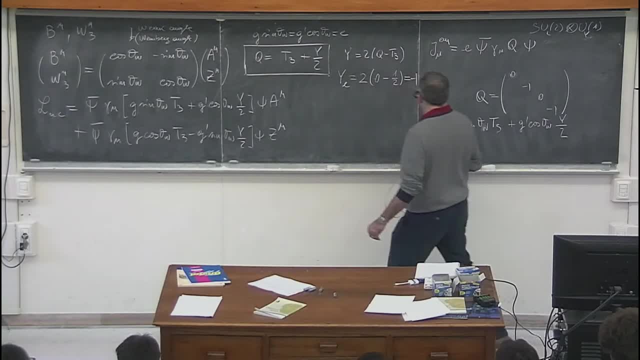 and this gives you minus one for the hypercharge of the left-handed doublet And you can check that the same value is obtained if you take the second component. If I take the second component, which is the electron, I have a minus one for the electric charge. 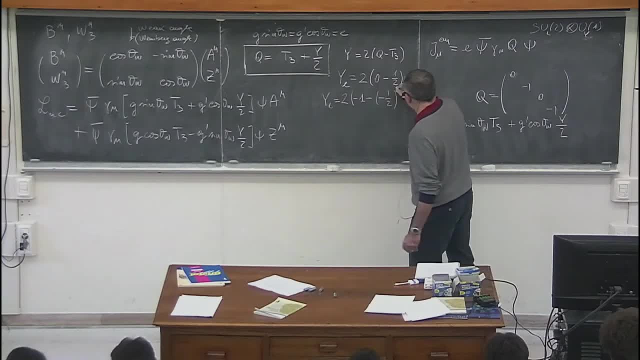 and a minus one-half for the weak isospin quantum number. Minus one plus one-half is minus one-half, so this is again minus one. And then I have hypercharge quantum numbers for the right-handed neutrino, for example. Right-handed neutrino has an hypercharge. 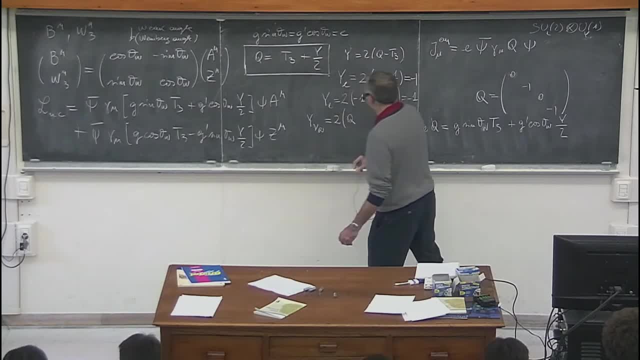 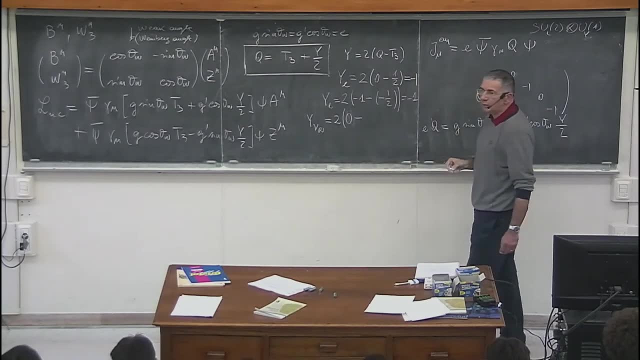 which is twice its electric charge, which is zero, minus the third component of the weak isospin, which is also zero because I have assumed the right-handed neutrino to be a singlet under the action of SU, and is zero. And finally, 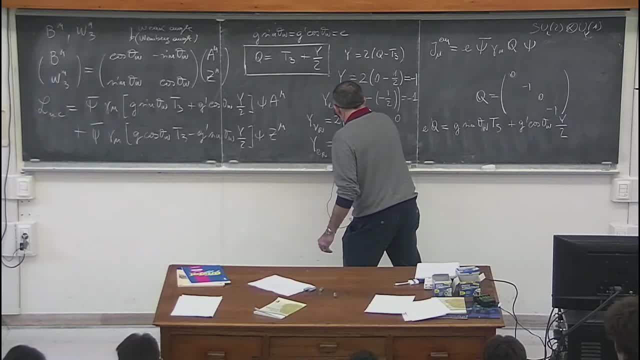 the right-handed electron has a hypercharge quantum number which is one-half, a hypercharge quantum number which is two times minus one, minus zero, which is minus two. So, with these assignments of the hypercharge quantum number, with this choice of the gauge group, 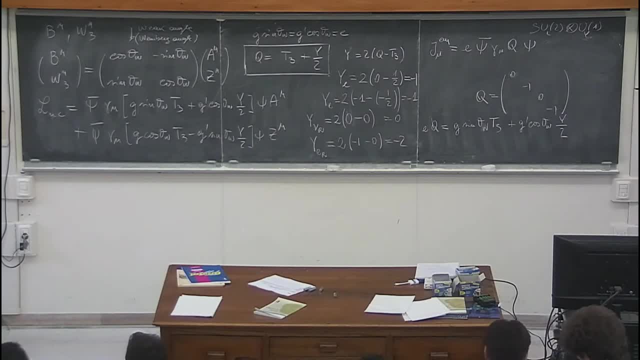 and this assignment of the hypercharge quantum numbers. I have succeeded- Weinberg and Glashow have succeeded- in constructing a gauge invariant system of currents which includes the charge current of weak interactions, those which appear in the Fermi Lagrangian. 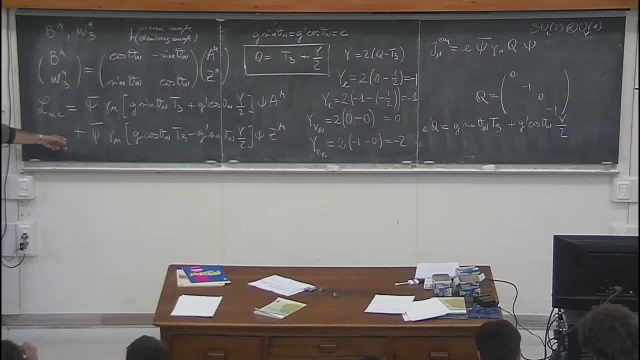 and the electromagnetic current. Again we have a neutral current which we will have to discover at some point. Let me just note that the right-handed neutrino has obviously zero electric charge. It has zero. It transformed trivially under the action of SU left. 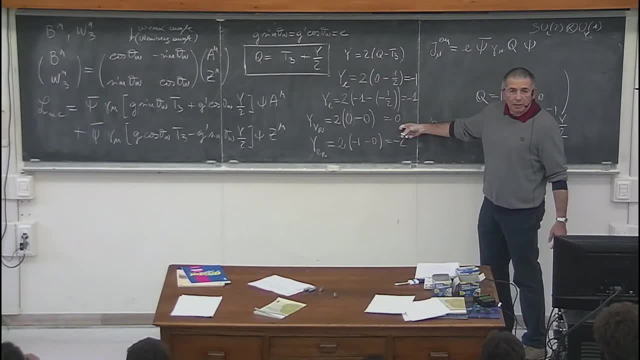 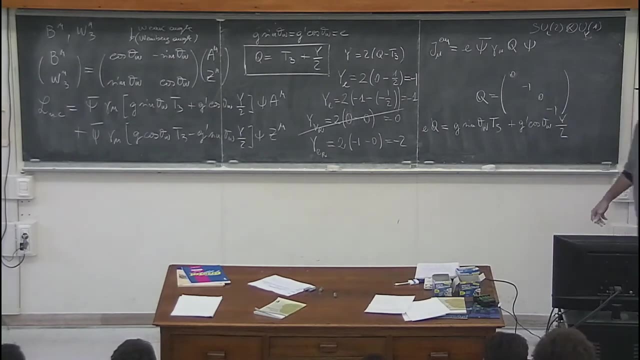 and it has also zero value of the hypercharge quantum numbers. So it looks like the right-handed neutrino doesn't take place in any sense in our construction, so I can just forget about it. It is a free object. It doesn't interact, neither weakly nor electromagnetically. 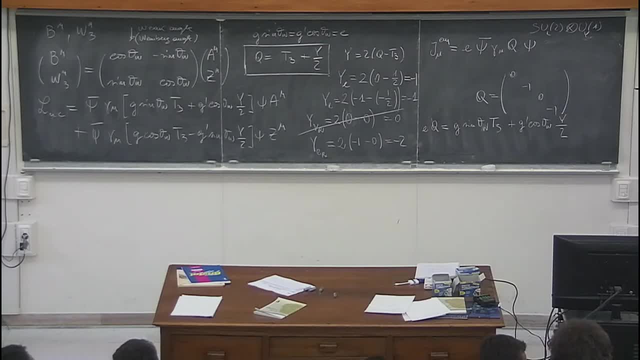 so it doesn't exist? Of course we know that it does exist and we will talk about that later. Anyway, we will not talk about right-handed neutrinos anymore for a while. What about? So this first current here I can just replace by: 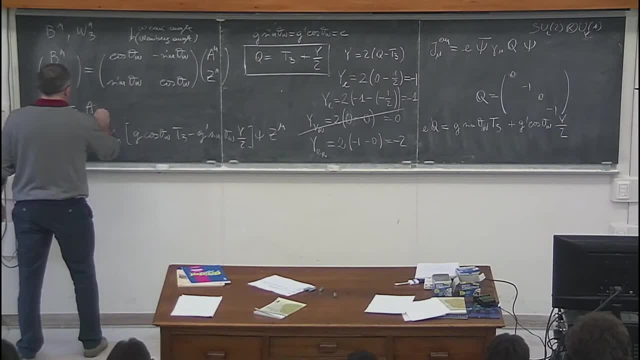 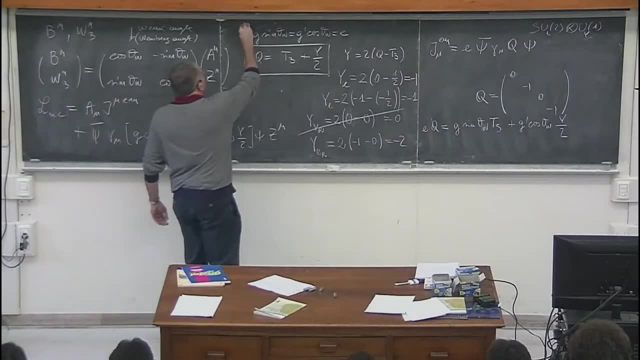 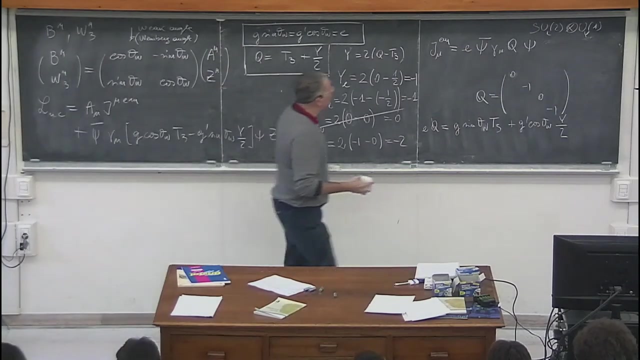 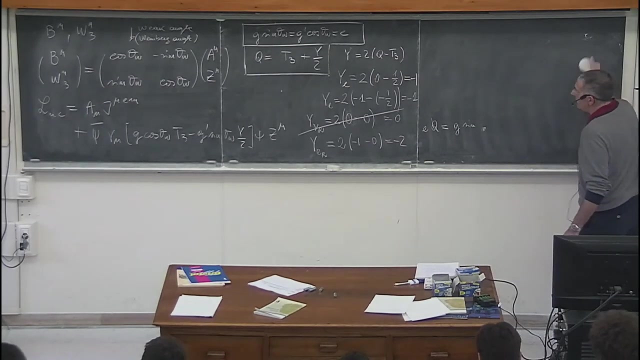 A, mu, J mu, electromagnetic. provided I have this set of choices, I have nothing to say about the interaction, the weak, neutral, current interaction term which is related to the Z boson, Except that with this assignment, we can write it like this: 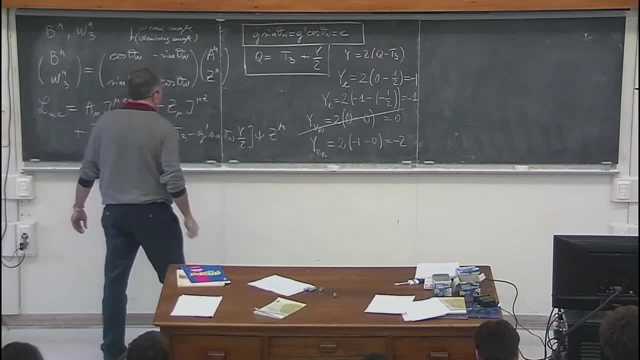 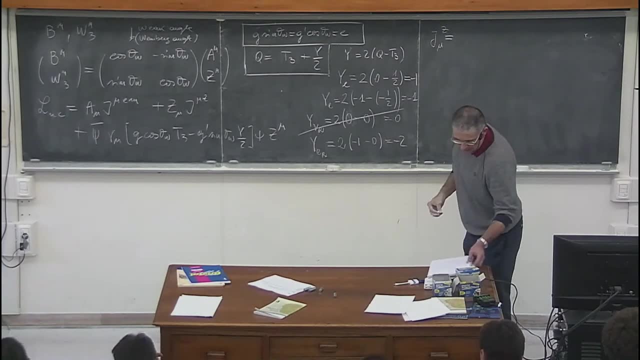 Z mu, J mu Z. where J mu Z can be written using these relations, It is written like this: It's: I introduce a new 4x4 matrix, QZ, which is given by 1 over cos, theta w, sin theta w. 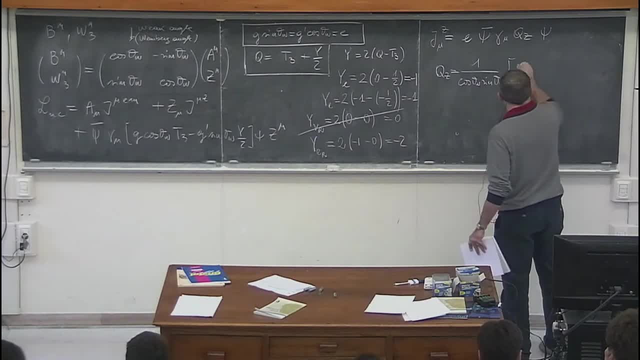 times T3 minus Q sine squared theta w, And I have to measure some weak, neutral current effect in order to determine the value of QZ and, in particular, the value of cos theta w, which is the only thing which is unknown in this combination. 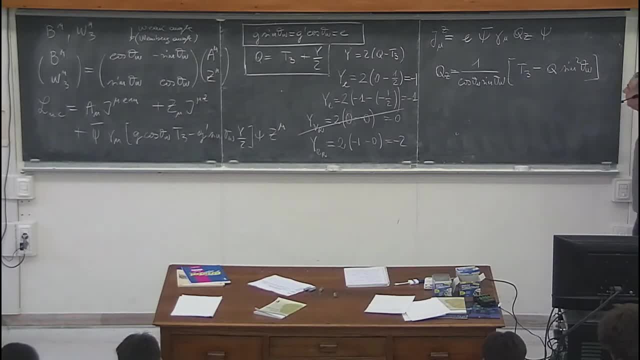 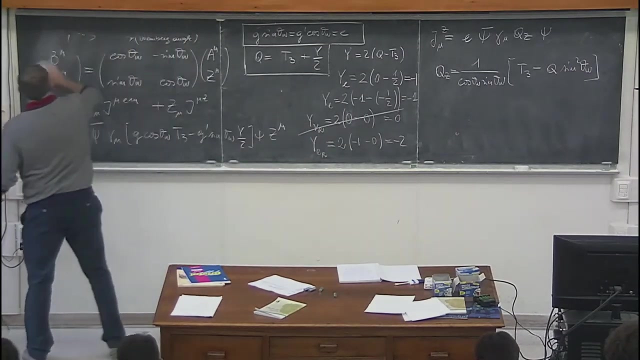 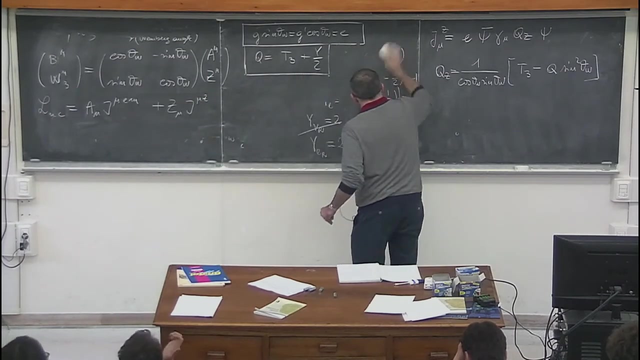 In particular. Well, okay, 10 minutes, Very good, Go ahead a little bit. What is missing? A lot of things. I better keep This, I keep These, I erase, but they are very important I have to keep in mind. 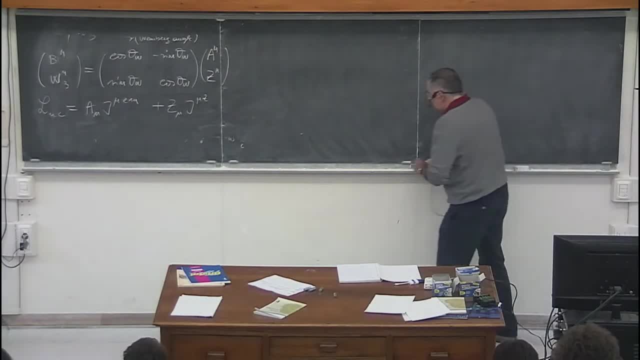 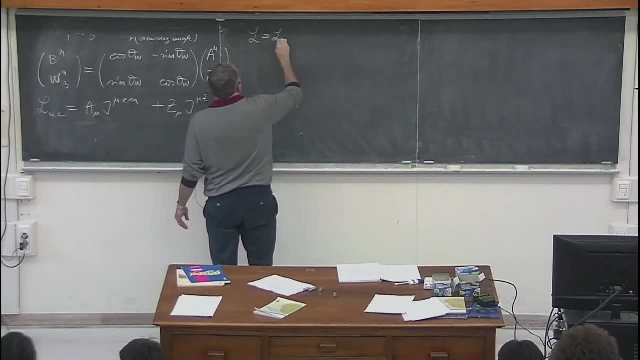 In order to complete the construction, I have to give the vector bosons their own dynamics. So I have to add to our Lagrangian L equal L0.. This is the free Lagrangian for the fermions. Then I have the two interaction terms. 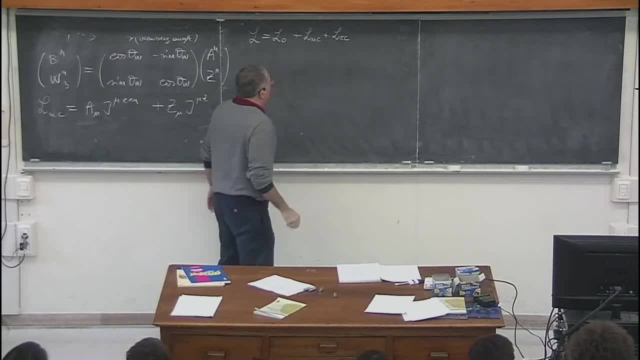 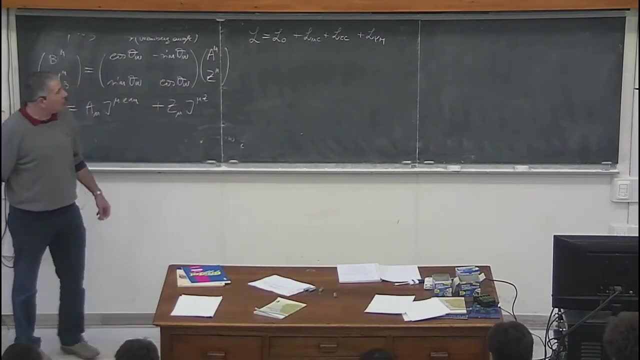 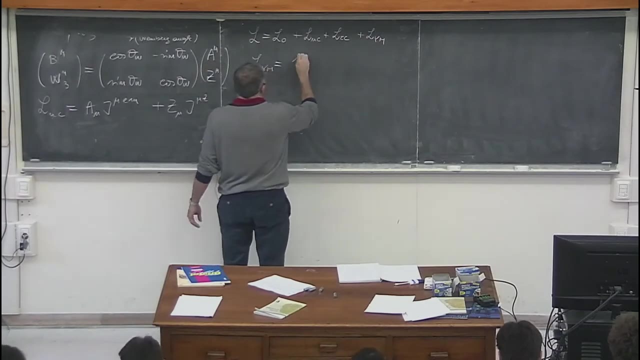 neutral current and charge current. And then I have to add a Young-Mills term for the four vector bosons. And this Young-Mills term is easy to write down: It's simply minus 1 over 4 b mu nu, b mu nu. 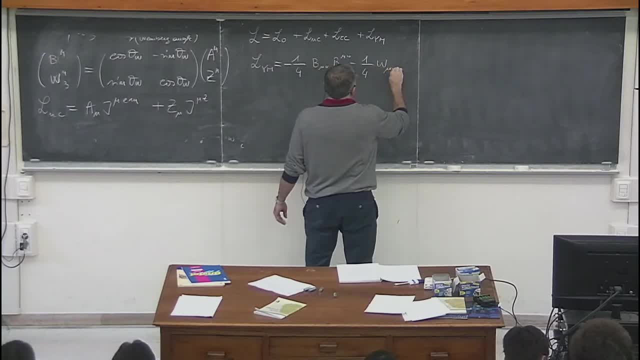 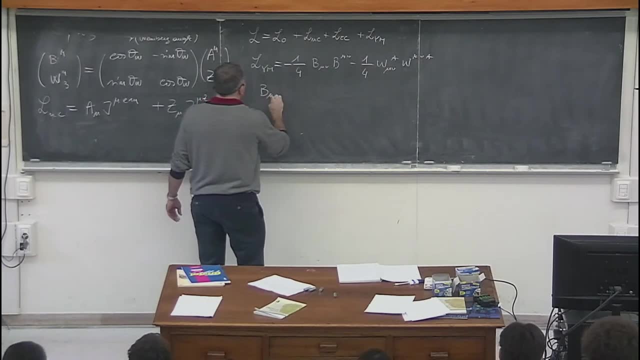 minus 1 over 4 w mu nu a w mu nu a b mu nu is easy to remember because b mu is the vector field related to an abelian factor of the gauge of groups. So it is simply the anti-symmetric combination d mu b mu minus d mu b mu. 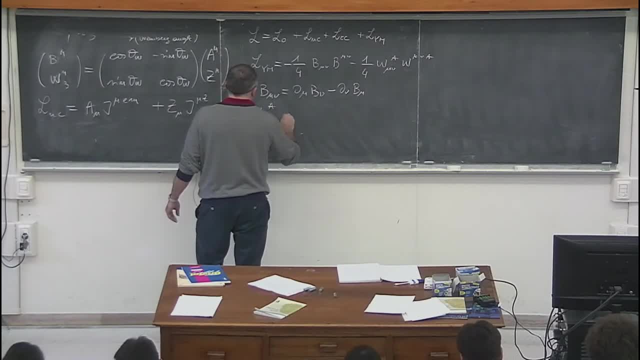 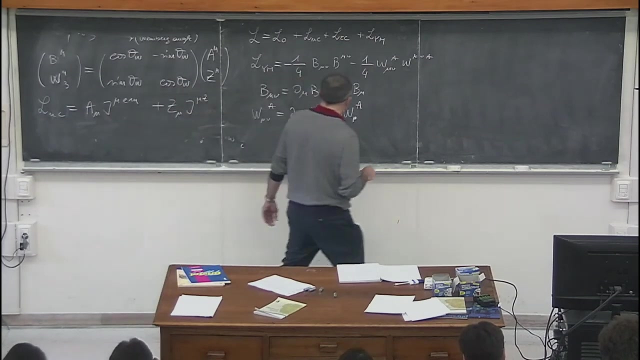 While w mu nu a, as you probably know, has a term which is similar to this one, But there is also a quadratic term in the fields without derivatives, And this is related to the fact that the group is non-abelian. It is written like this: 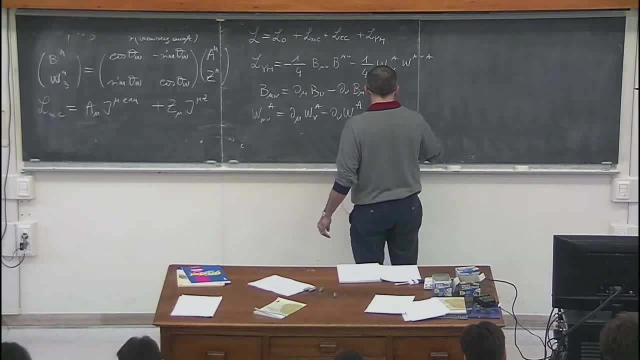 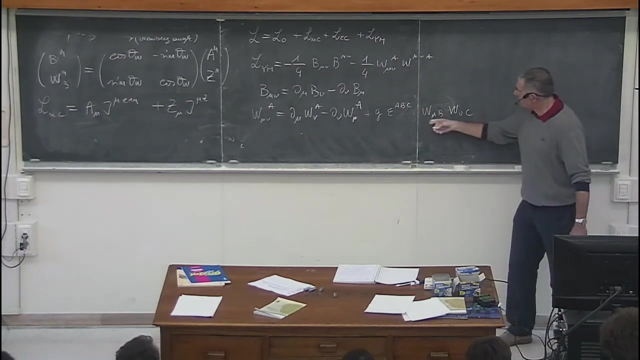 epsilon mu nu rho w mu, sorry, epsilon a b c, w mu b w mu c, something like this. Let me check the sign. Yes, like this, And this is important because it gives rise to interactions of the gauge bosons with themselves, which is not the case. 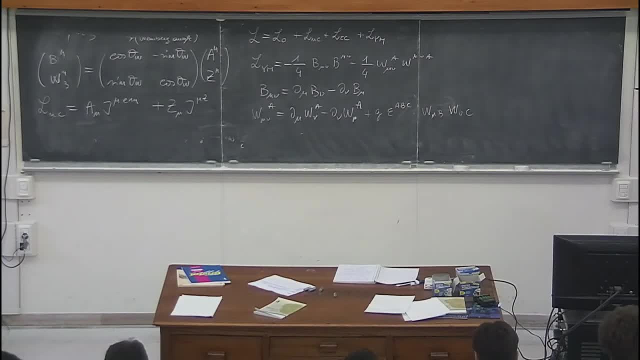 if you have an abelian gauge group. This is actually all, except that we would like to express this term in terms of: instead of w1,, w2,, w3 and b. we rather write it in terms of a mu, z mu and w? mu. 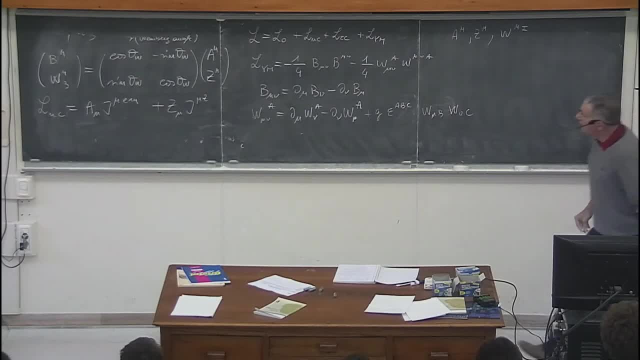 plus minus. the relation between a? mu and z mu and b mu and w mu 3 is written there. We also had w mu plus minus equal to 1 over root of 2 w mu. 1 minus plus i w mu 2, and it's just a matter of algebra. 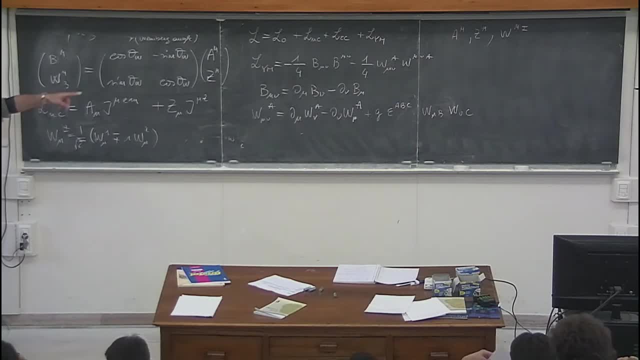 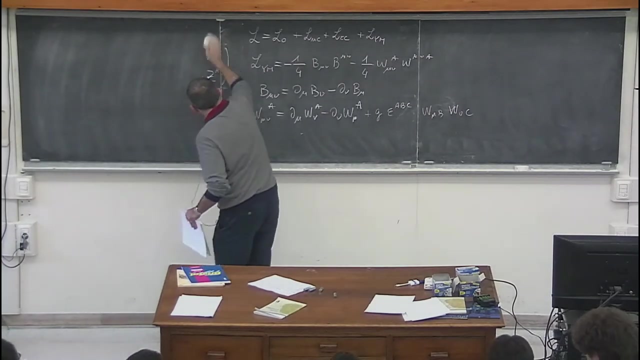 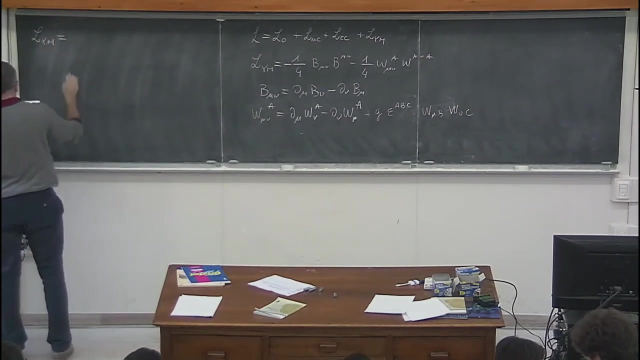 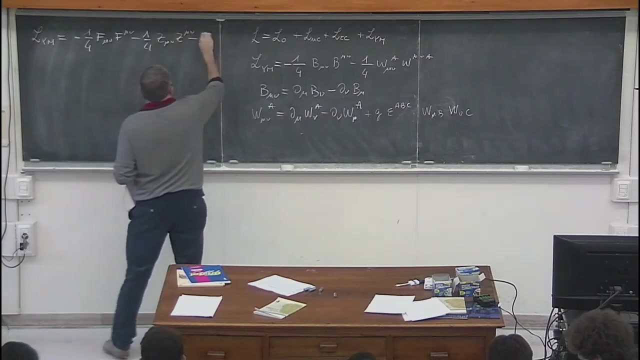 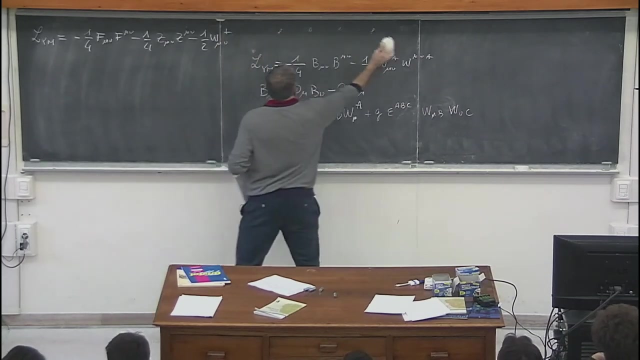 replacing this definition, this one and this one into the Young-Mills Lagrangian to get the final Lagrangian density for the vector fields. I write it down for you, just copy it. in order to complete the construction, There are three quadratic terms, which are the usual ones. 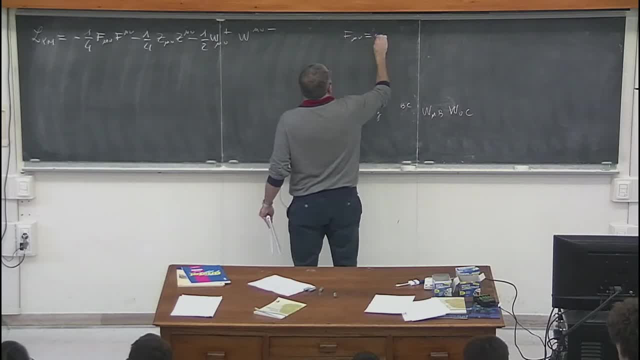 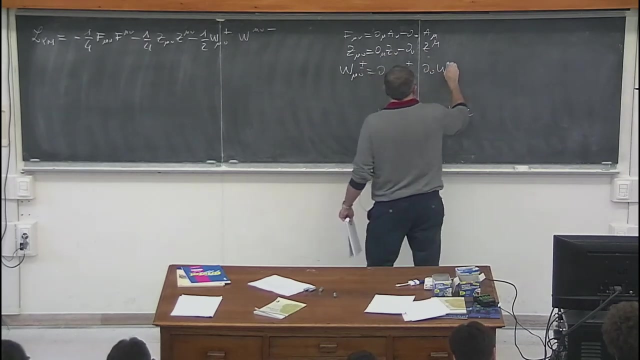 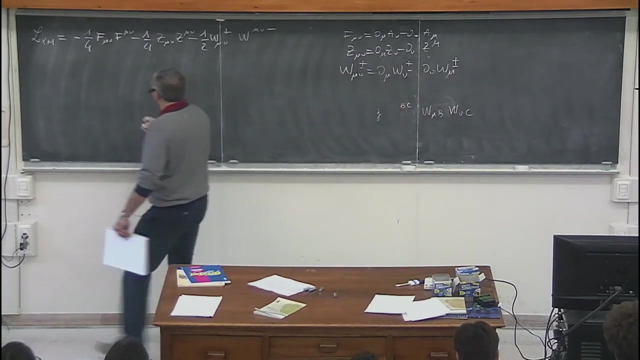 where f mu nu is a factor of 1 over 4. here, as you know from Maxwell equations, a similar factor of 1 over 4 in the z term, which is also a neutral vector, but the term, the kinetic term involving w mu nu is a factor of. 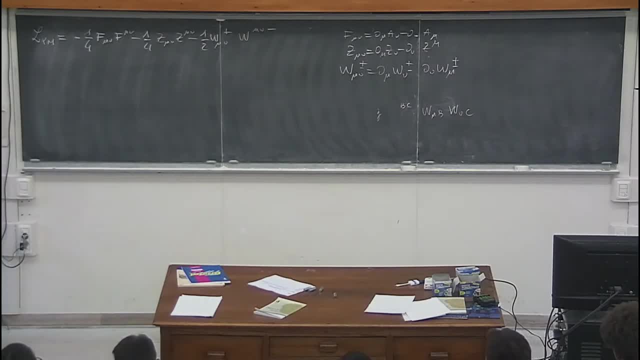 1 half because it is a charge vector. so in order to have the canonical normalization of the propagator, you have to put a factor of 1 half here instead of a factor of 1. fourth, and then you have interaction terms. This interaction terms originate 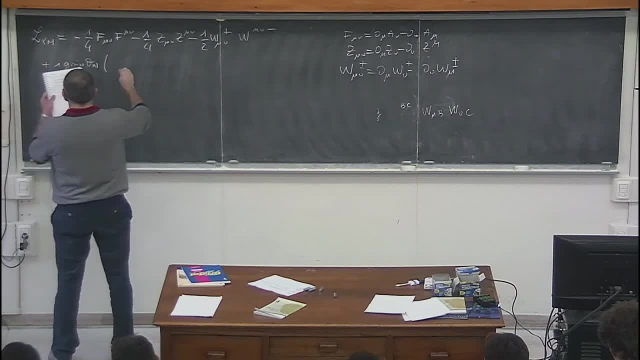 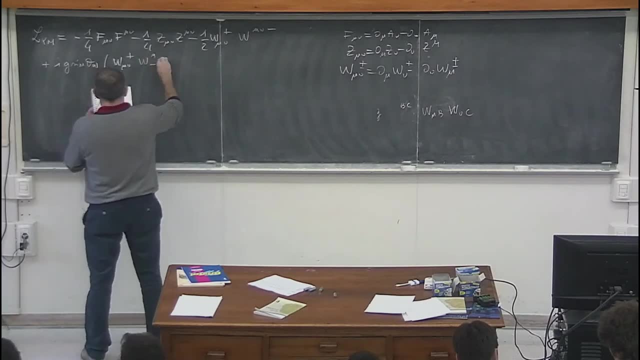 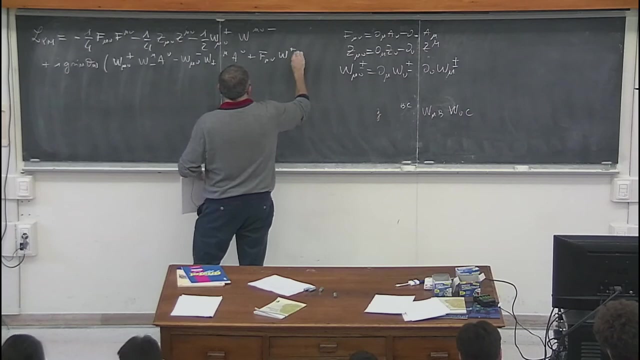 from the fact that part of the gauge group is non abelian is written like this: w mu nu plus w mu minus a nu minus. w mu nu minus w plus mu a nu plus f mu nu w plus w minus. this is easy to understand in a sense. 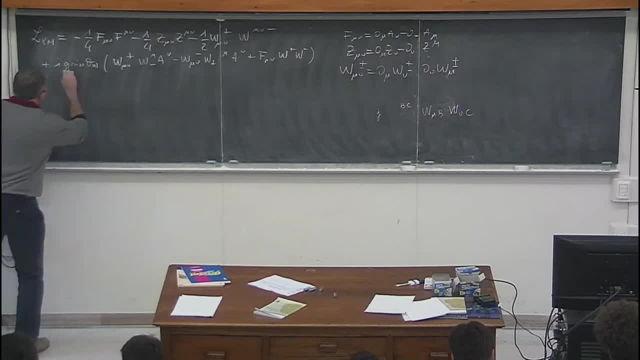 because g sine theta is simply e, and e is the charge of the w boson and this is simply. this simply reflects the fact that the w boson being electrically charged is coupled to the photon itself. then there is a similar term in which g sine theta. 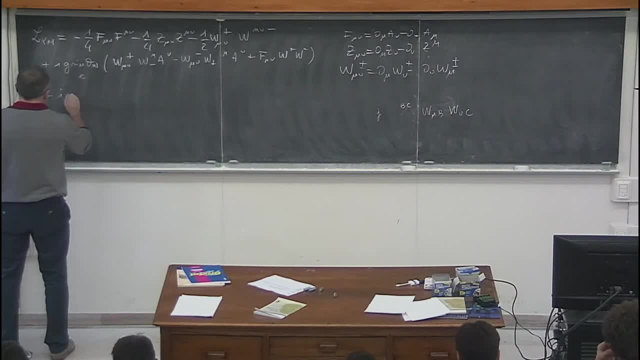 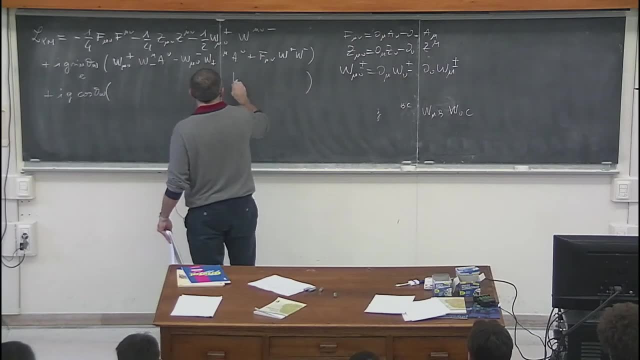 is the charge, and g sine theta w is replaced by g cosine theta w, and the round brackets are just the same, except that you have z instead of the photon field. these are three linear interaction terms, and then you have a four vector interaction term, which is sorry. 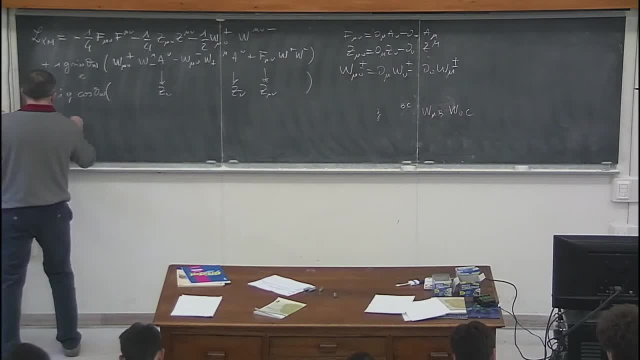 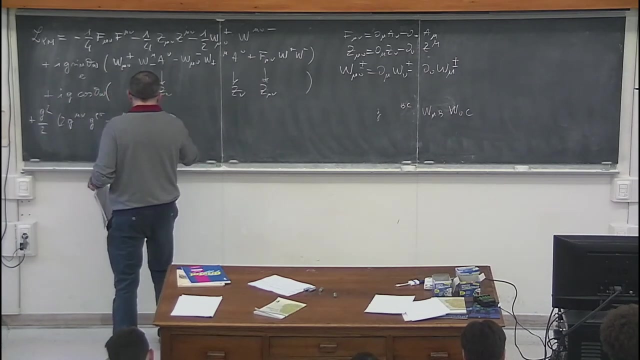 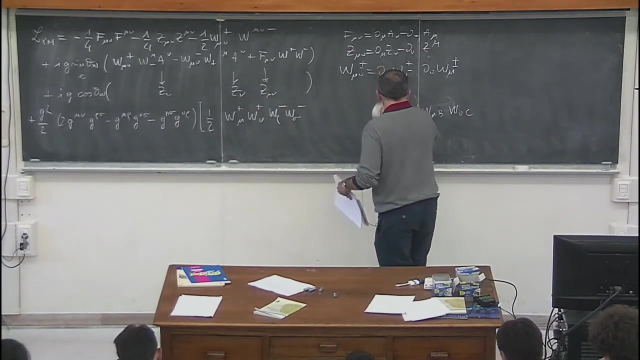 a bit long to write down two. the tensor structure is this: one two g mu nu g rho sigma minus g mu rho g nu sigma minus g mu sigma g nu rho times. a long thing. one half w. it's not very interesting. just for the sake of completeness. 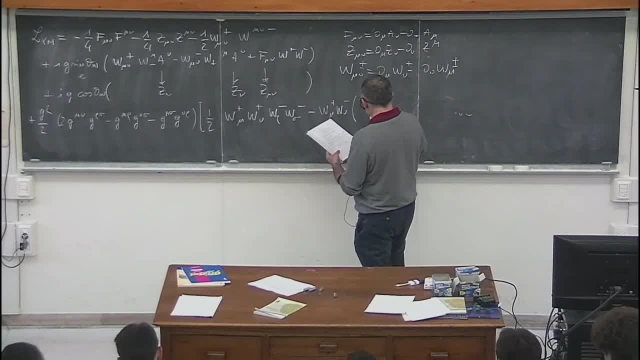 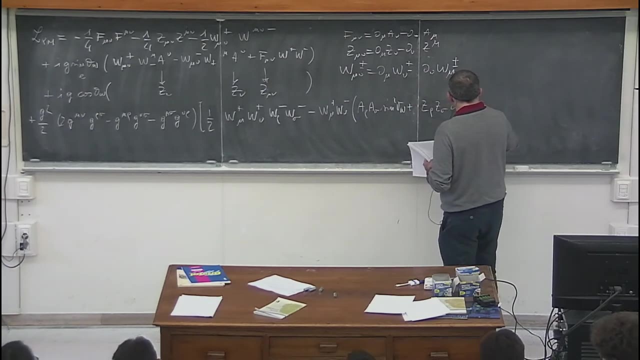 we write the whole Lagrangian line down: a rho a sigma times sine square theta w plus z rho z sigma cosine square theta w plus two: a rho z sigma sine theta w cosine theta z. and that's it. so i erased the full Lagrange and 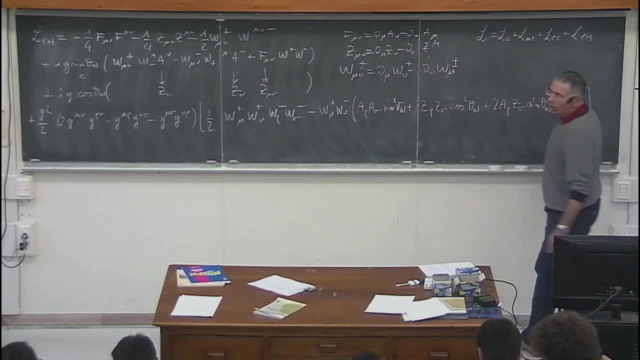 zero l neutral current, l charge current, l young mills. this is electromagnetism as we know it. It also includes weak neutral currents about which we don't know much as yet, But for the rest it is what we settled out to have. It is a renormalizable and unitary theory of weak interaction of. 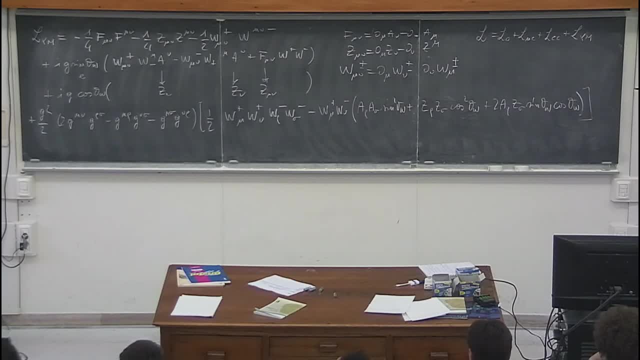 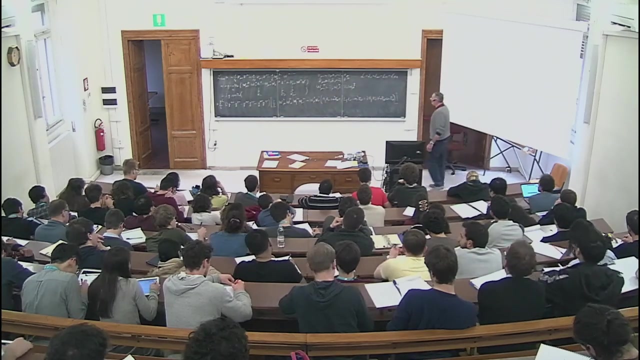 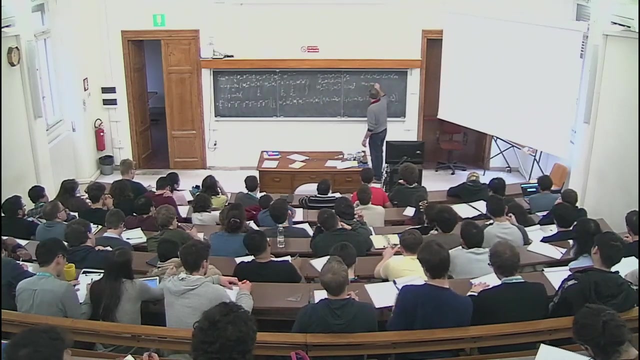 leptons. It is renormalizable and unitary. because gauge field theories are known to be renormalizable and unitary, It can be shown on the general ground. There are many missing points. The first one is how to introduce non-zero values. 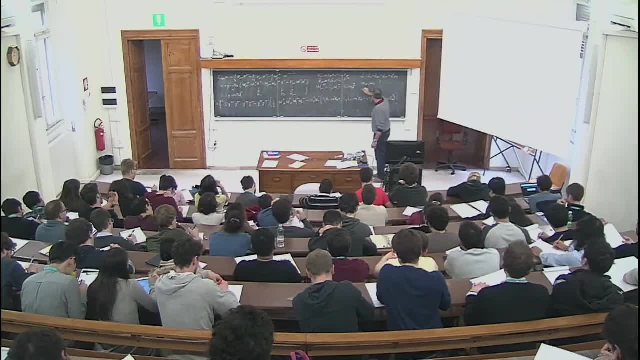 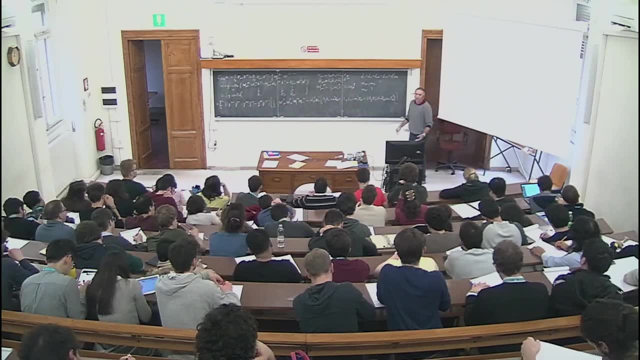 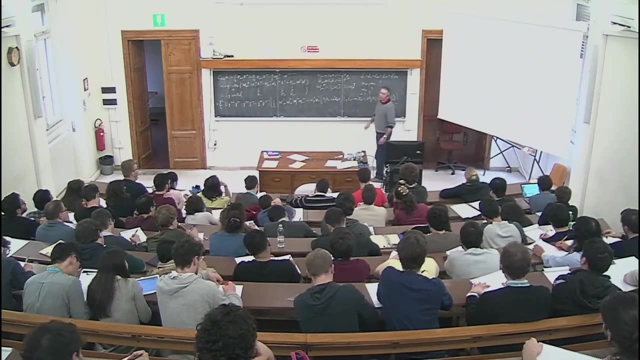 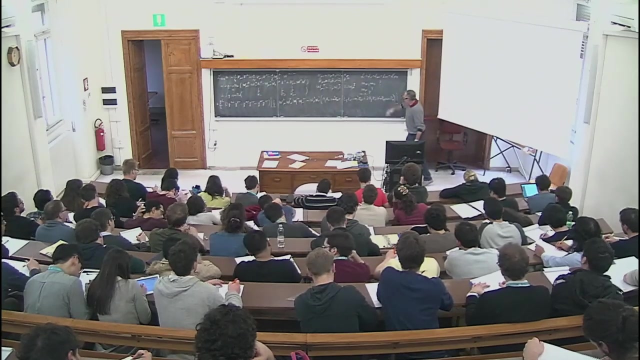 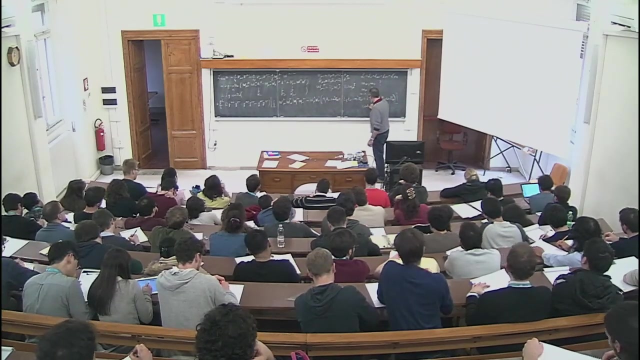 for the weak vector, bosons. The second one is how to introduce masses for leptons, at least for charged leptons, And finally, do neutral currents exist? So we will have to fill these gaps. And there is a fourth one: How do we extend the theory of this construction to hadrons? 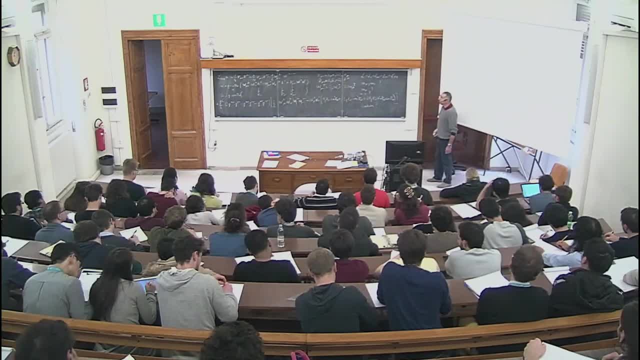 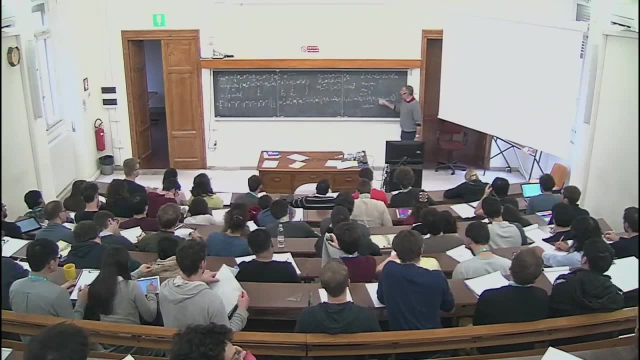 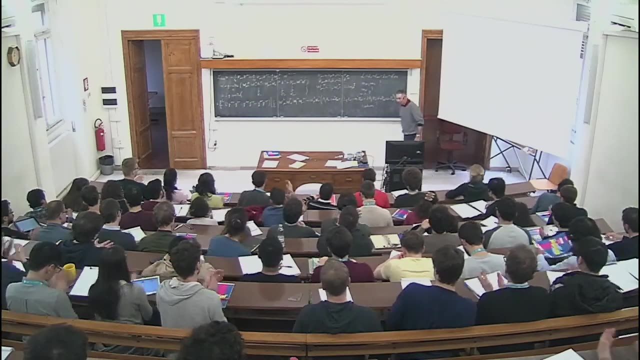 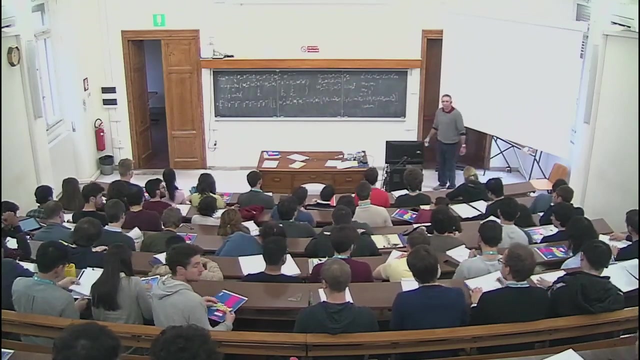 Which is an important point. So I think I stop here And we go on tomorrow with the last point And then we will attack the problem of masses. Okay, Thank you very much, Thank you.